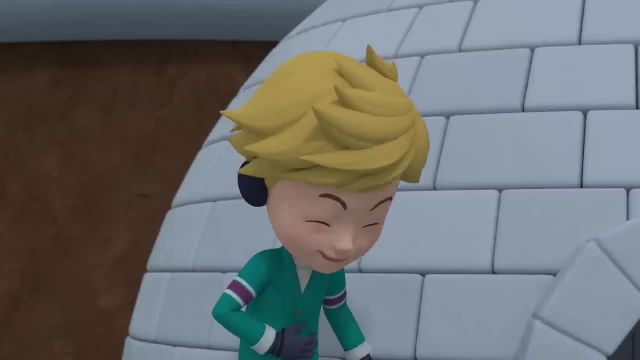 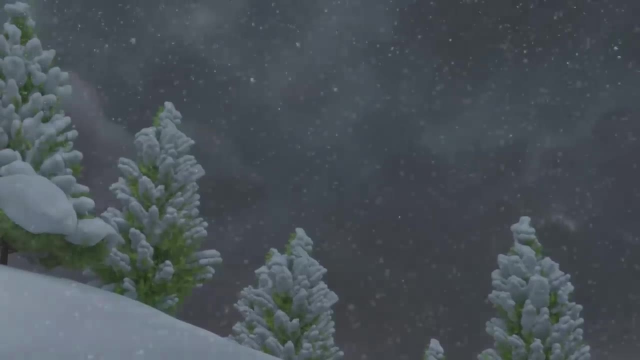 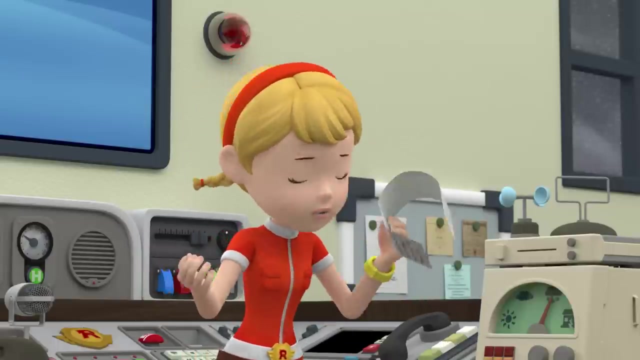 Ha ha ha. Sure, whatever It's cold, Aren't you coming in? Hey, Not till you admit I'm the captain. Oh wow, It's going to keep snowing all day. This could be the year's biggest snowfall. 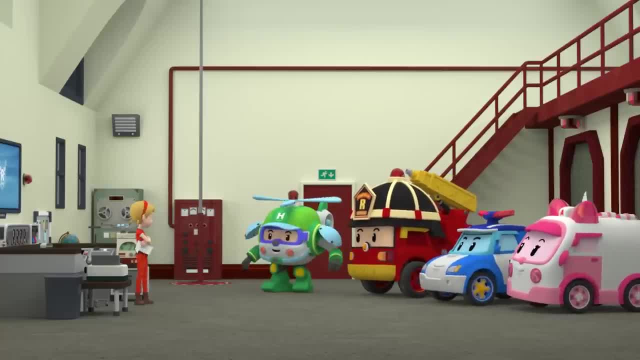 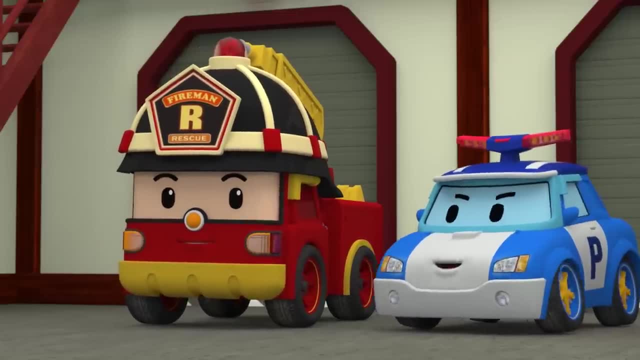 Aw cool, We should make boards and snow helicopters, Heli. on snowy days there tend to be more accidents than usual And that means we have to be on alert to help people. But I'm sure you knew all that already. 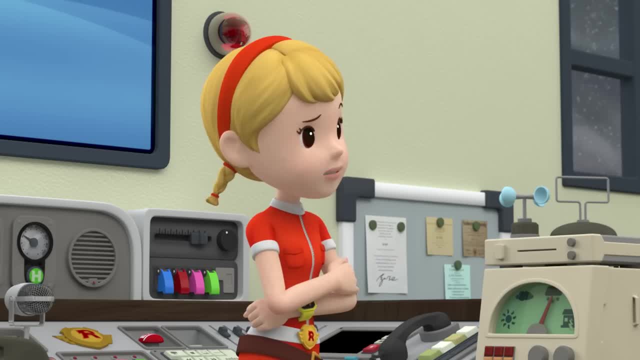 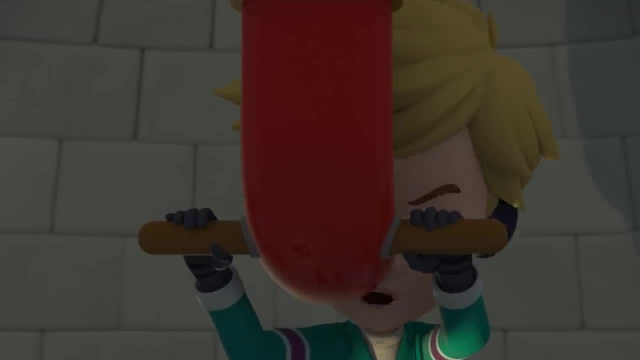 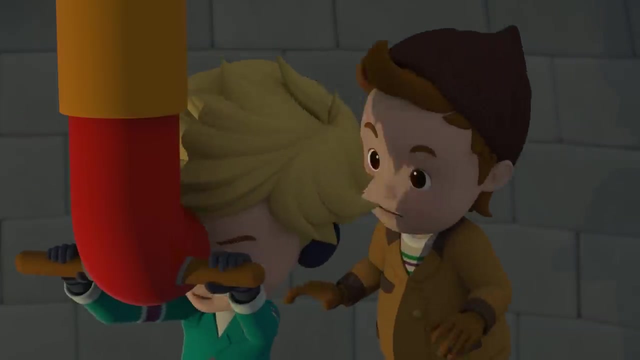 Of course I did silly. Maybe you need a refresher quiz. Whoa, There's a snow monster. It's a 12-legged elephant, yeti, A what I want to see. Wow, there's a polar bear passing. 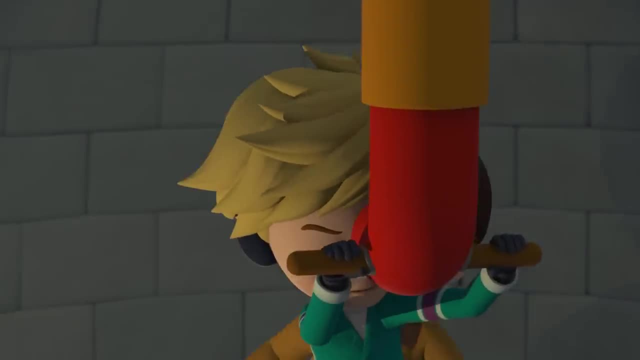 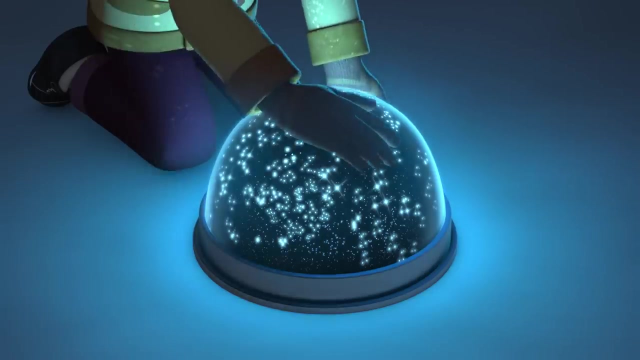 Come on, it's my turn. And an army of emperor penguins. So cool, Peter, Whoa, Charles, what's that? This is my constellation projector. It projects the night sky. Cool, right. Yeah, it's pretty. 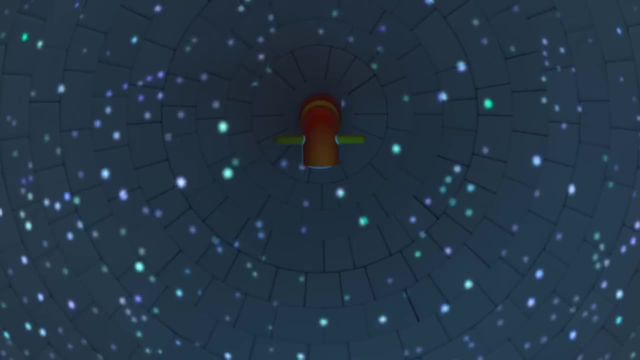 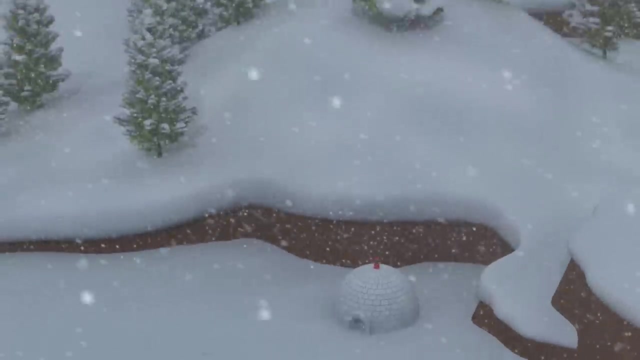 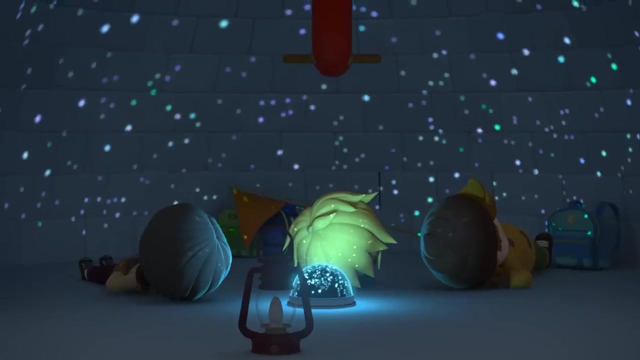 This is what we'd really see in Antarctica. Well, we'd see auroras too. Hey guys, let's go to Antarctica. Yeah, Huh, Is that you, Johnny? What's going on? Oh no, the exit's covered in snow. 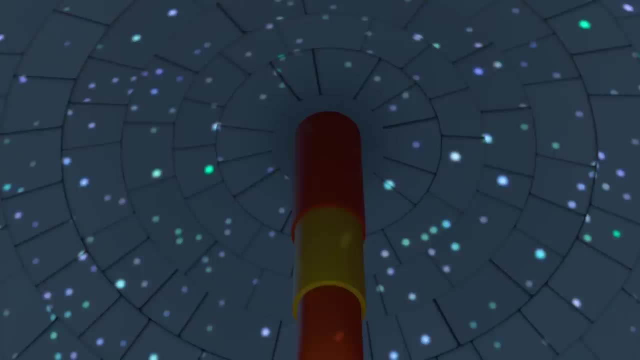 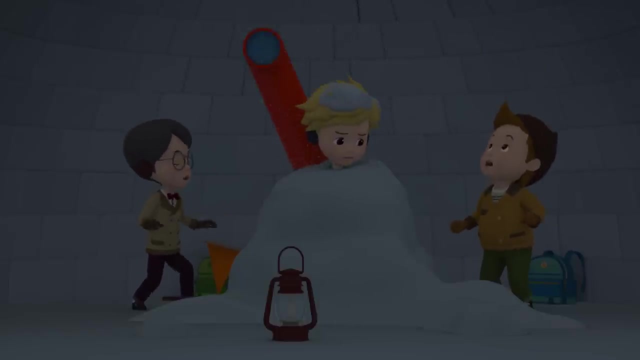 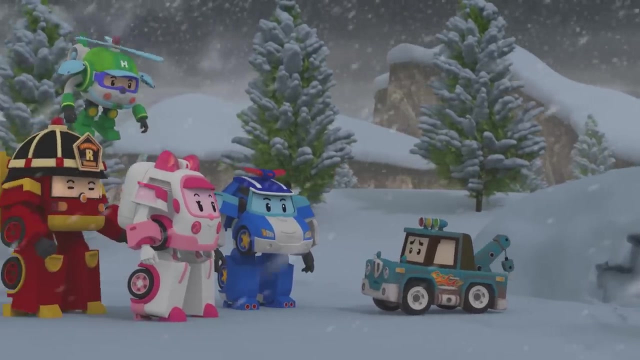 Our view outside's blocked too. It's all black, Peter, We might be in trouble. you guys Help. Thanks for your help. I was really stuck Spooky. whenever it snows, the roads can get really slippery with ice. 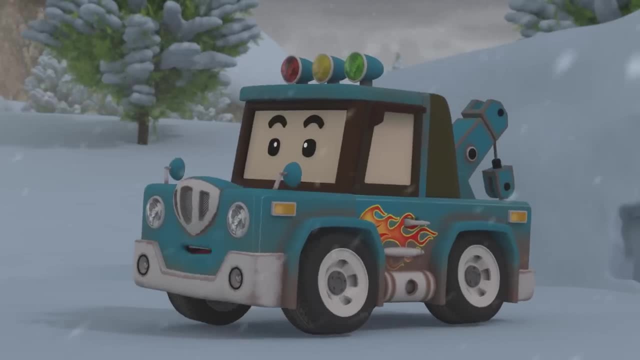 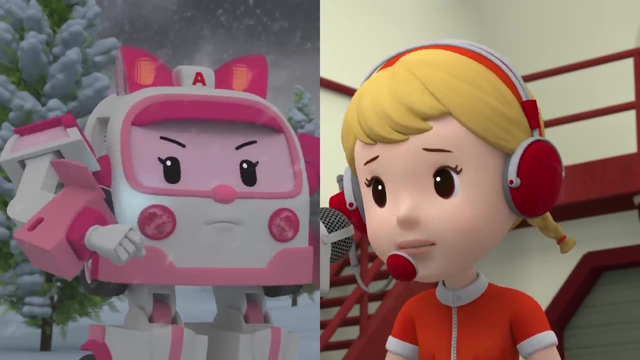 So it's important to go slower than you usually would. I sure will. Huh Hi Jin, We need your help. The kids were playing on Apple Street, but they haven't come back yet. Dispatch the team right now. Understood. 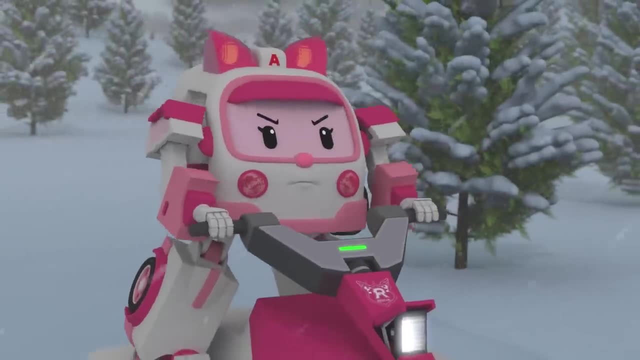 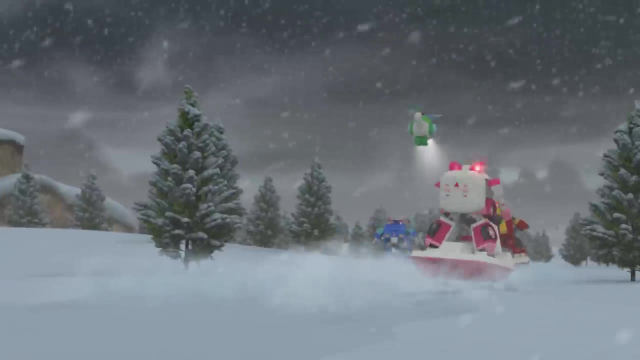 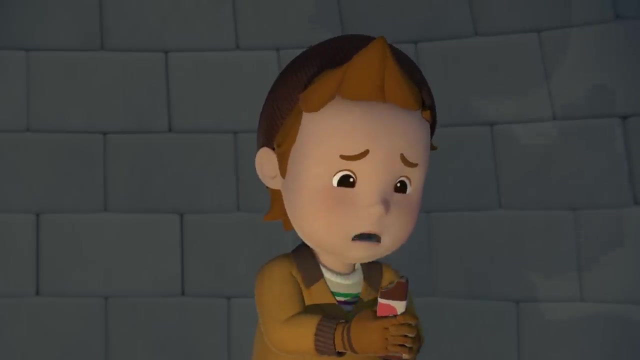 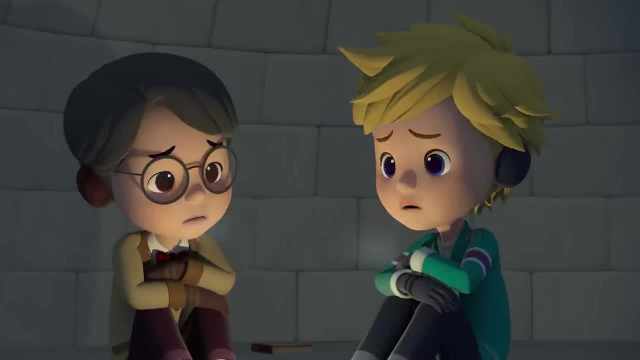 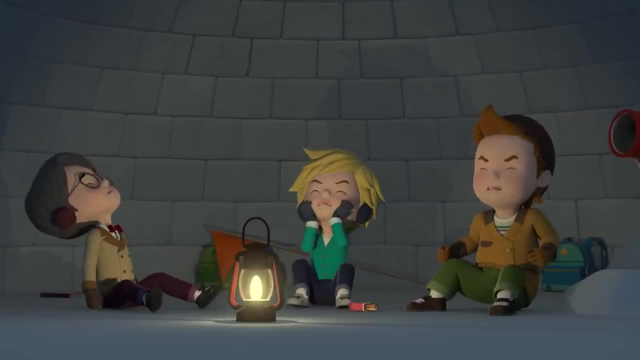 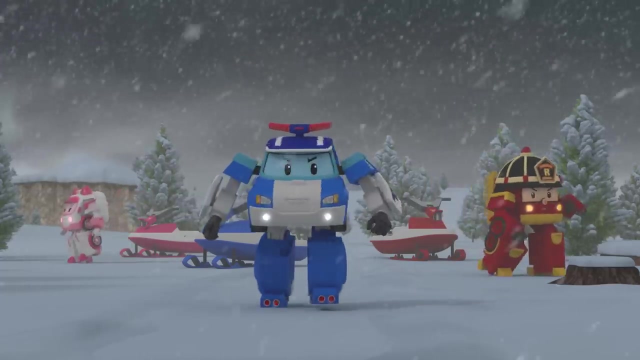 It's frozen solid. We're all frozen solid. What if we're not discovered for years Like dinosaurs? We're done for Kids Rescue team. We're in here, Peter, Johnny Charles, Listen If you hear us yell. 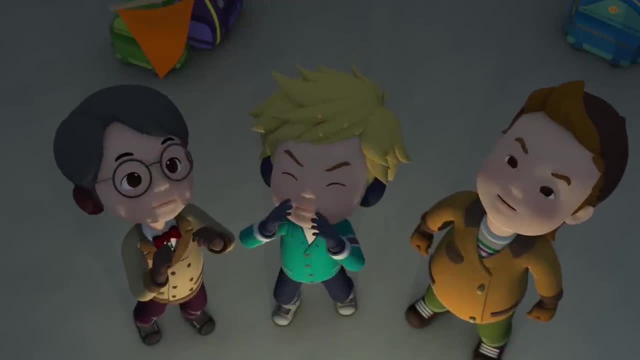 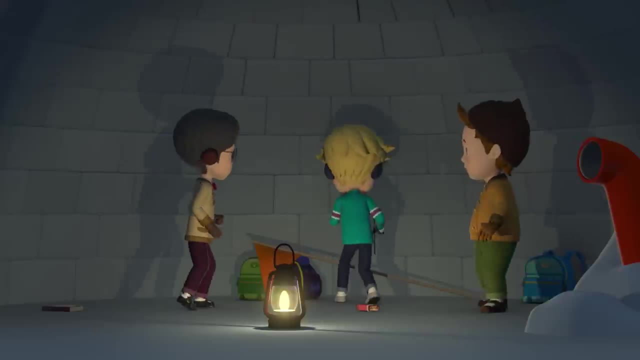 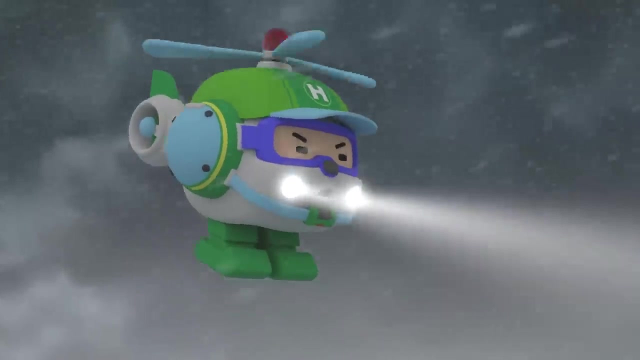 Down here. Can you hear us, Peter, Johnny? I don't think they can hear us at all. This is the end. Oh, wait a sec, We're down here. Come on, Hello. Oh, what's that? I see them. 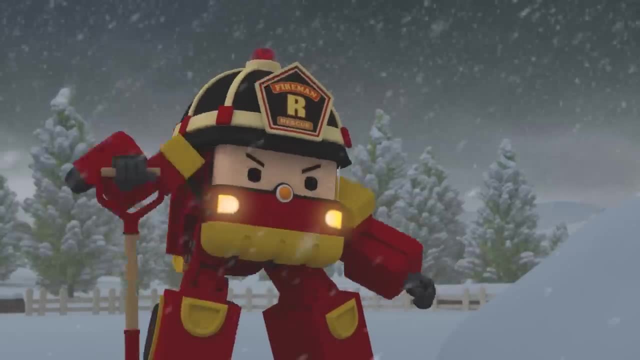 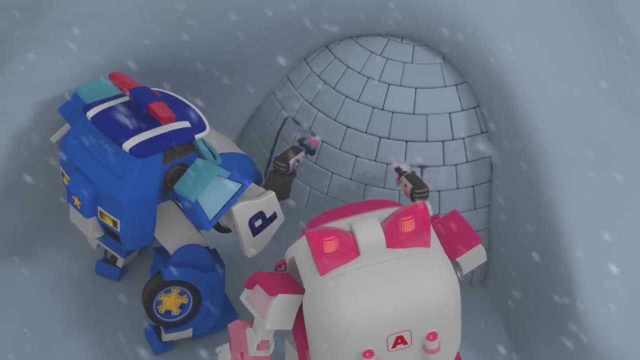 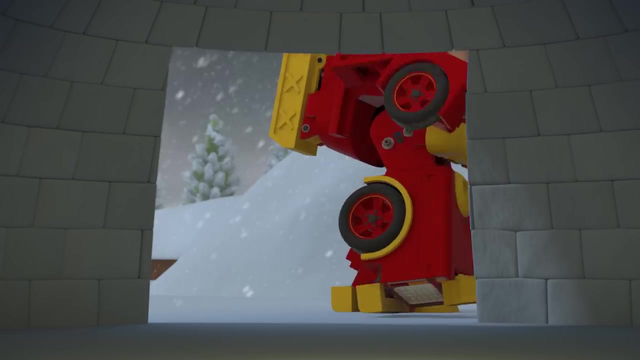 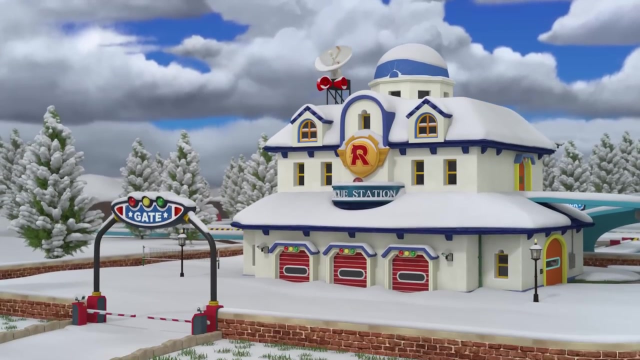 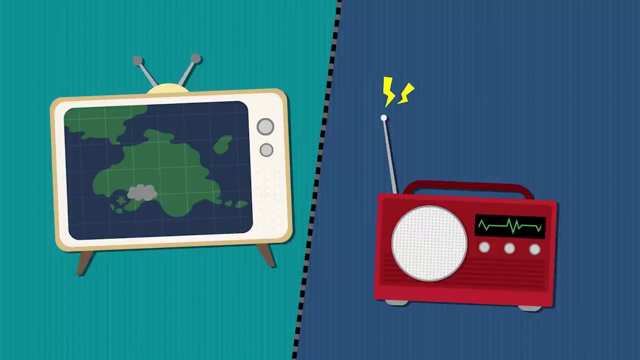 Oh, All right, stand back, We're back. Hey kids, You okay. Hi, Hi Roy, Thank goodness, you're all safe. Thank you. When the snow is heavy, there are some things to remember In winter. pay attention to weather forecasts. 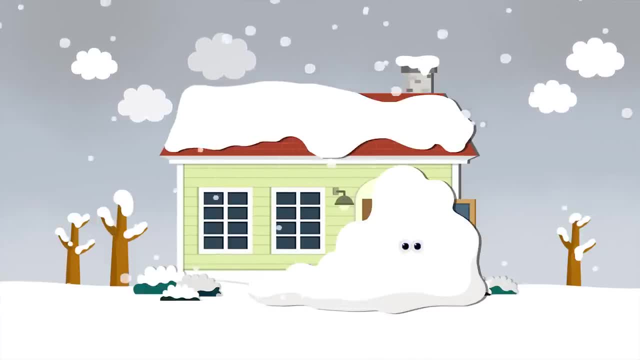 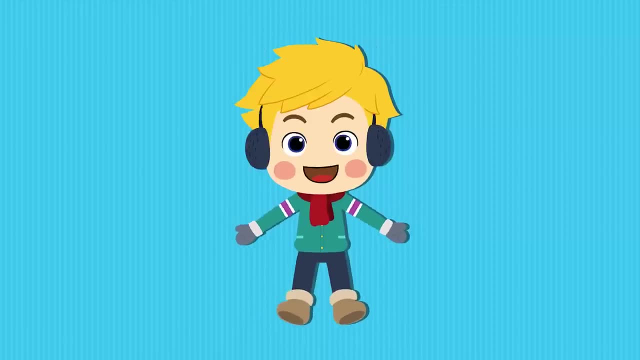 to see how bad the snow is expected to be, What's expected be On days with extra heavy snowfall. it's best to stay inside And if you do go outside, remember to wear your gloves, a scarf, warm shoes and something to. 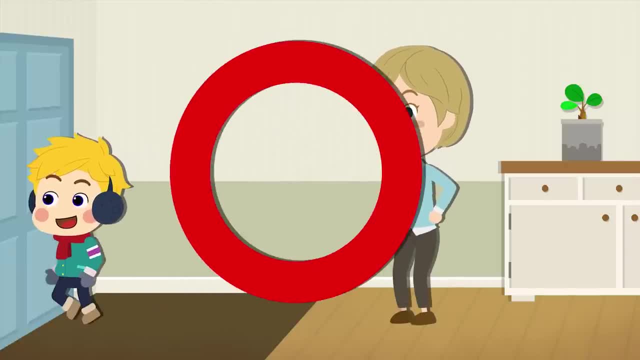 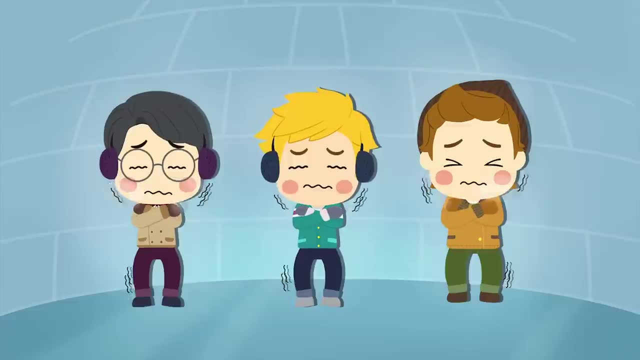 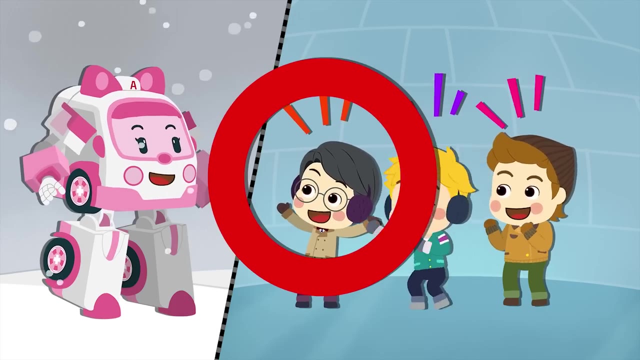 cover your ears. Always tell your family where you're going and when you'll be back. If something happens and you need help, try as many ways as possible to signal for help. While you wait for help, move around to keep your body temperature warm and remain calm. Hmm, got it. We'll do our best, You guys. Huh, It just stopped. 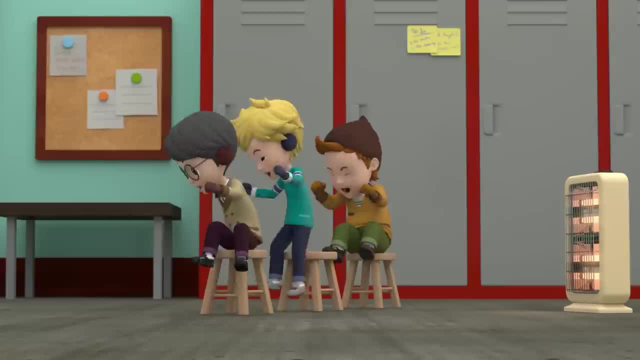 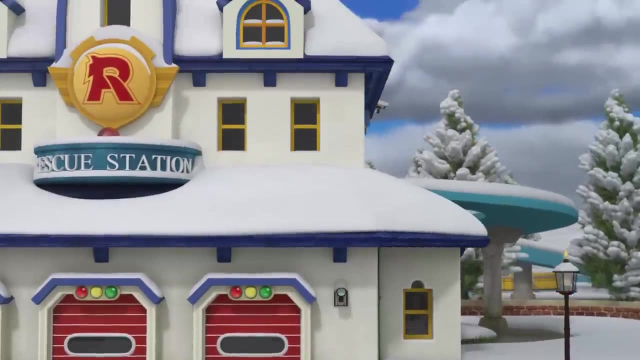 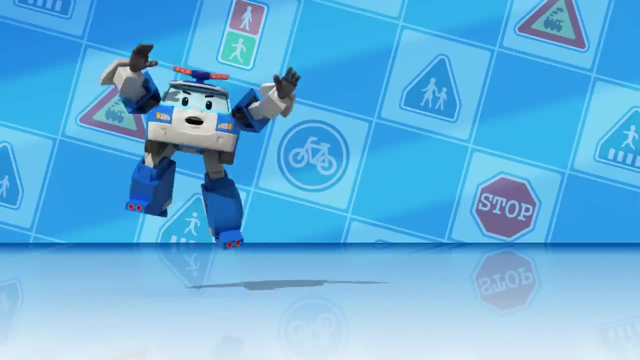 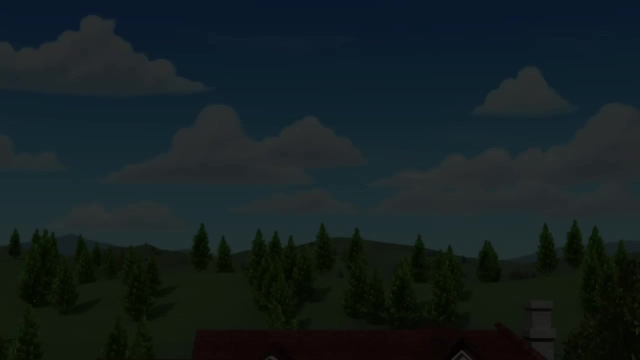 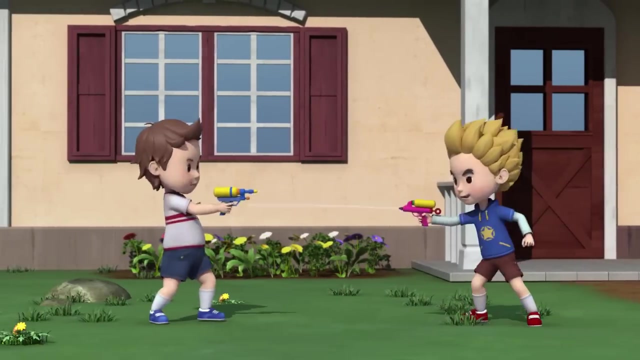 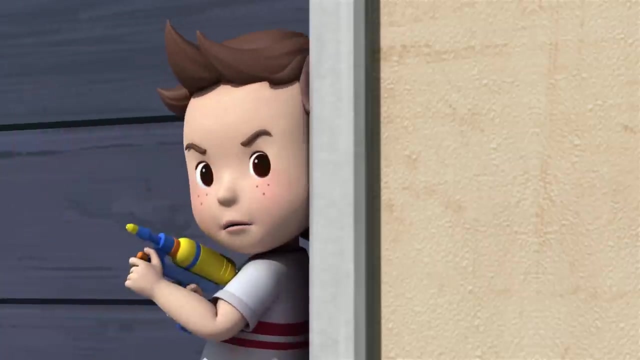 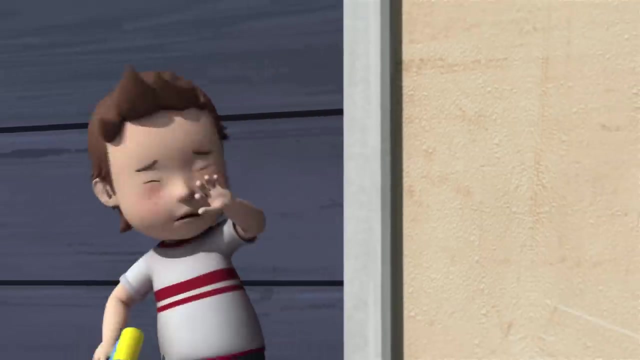 snowing, so snowball fight, Really, Alright, Snowball fight. Well, we do what we can. Don't run between cars. Take that, Oh yeah. Stop Got you. Now it's my turn, Oh no. 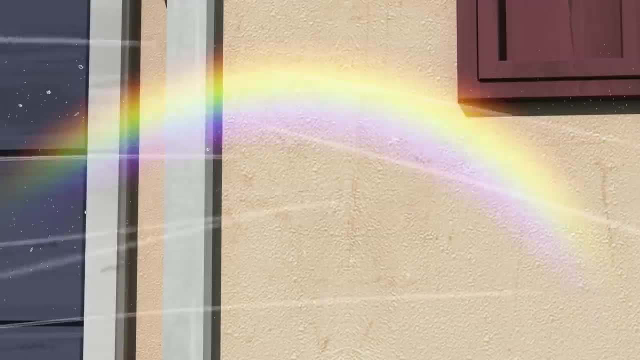 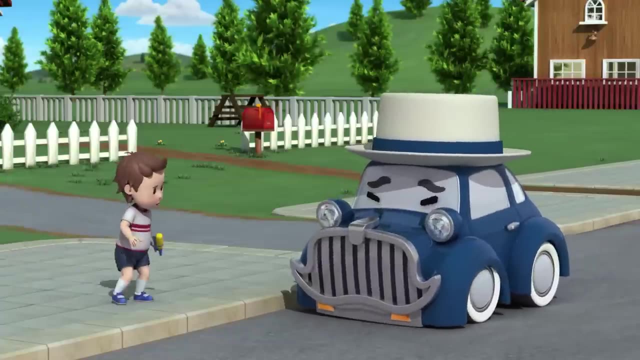 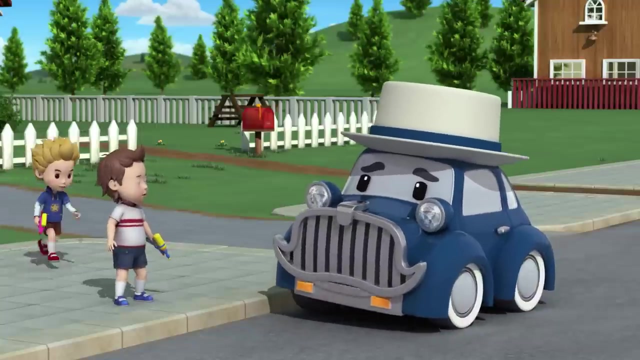 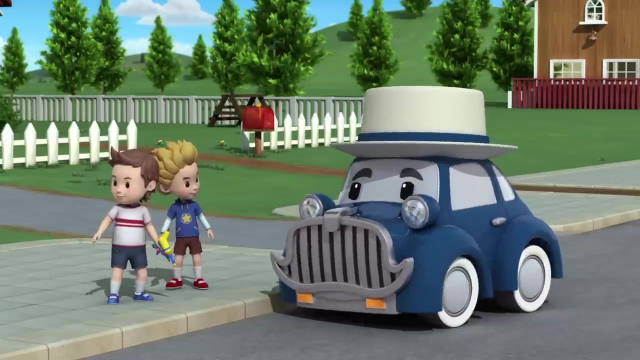 Oh, no, My turn, Take that. Oh, that's so cold. I'm really really sorry, Mr Musty. Oh, never mind. Now let's see. I'm looking for Lewis's new house. Oh, I know where his house is Over there, The house with the blue roof. 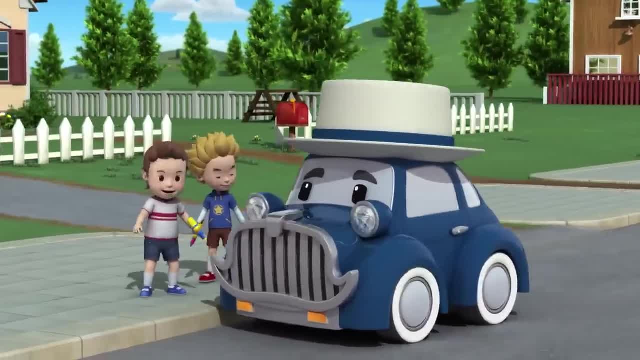 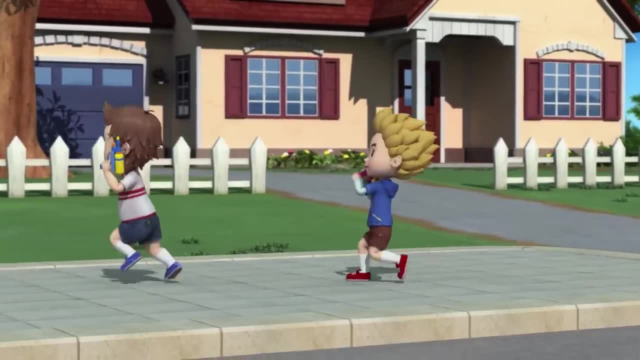 I see it now. Thanks a lot. Bye-bye, Mr Musty. Huh Hey, stop, Yeah got you. That's not fair. You snooze, you lose, Stop. Uh-oh, I'm running out of ammo. 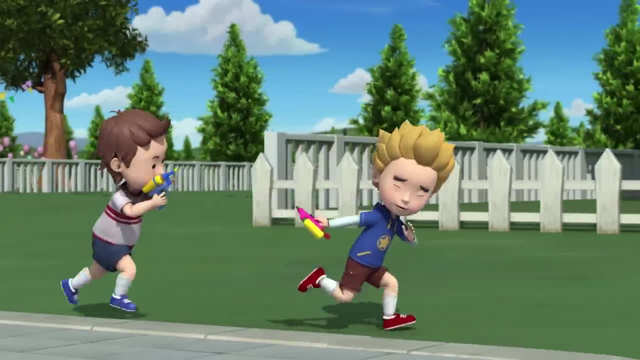 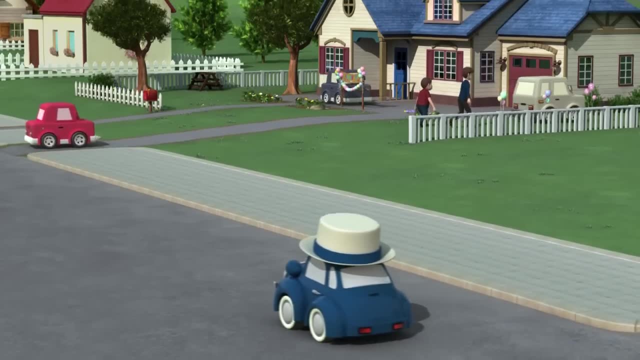 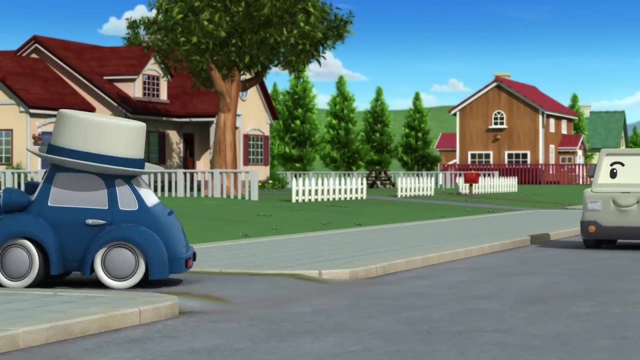 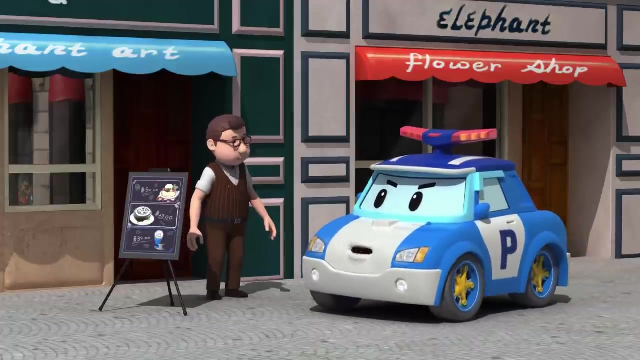 My turn. Oh come on. Yeah, Stop. No, How do you like that? Oh yeah, Oh look, There are so many visitors here. I hope I can find a space. If you put that big sign in this small alley, it could block a driver's view and cause a bad accident. 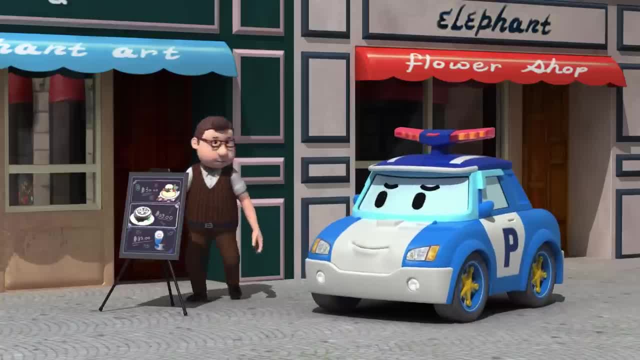 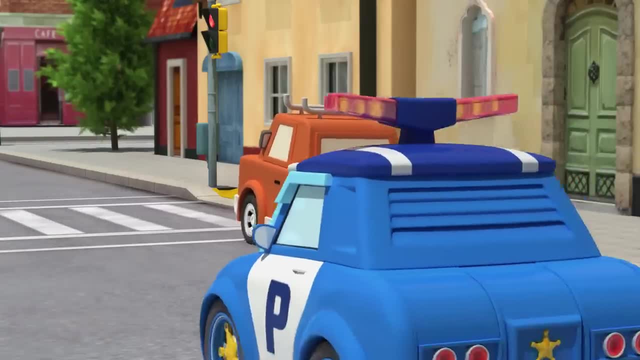 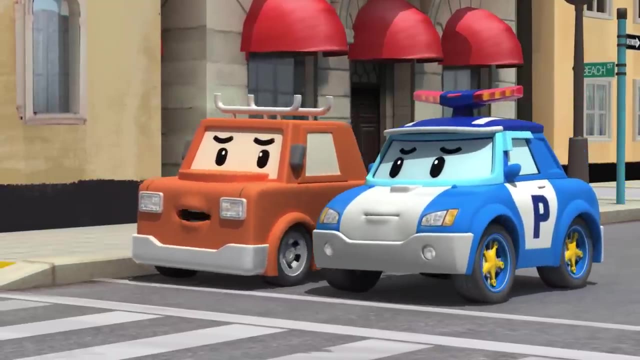 Oh right, So sorry, I'll move it now. Polly Good, Have a nice day. If you park right in front of the crosswalk, the children won't be able to see when they try to cross the street Right. 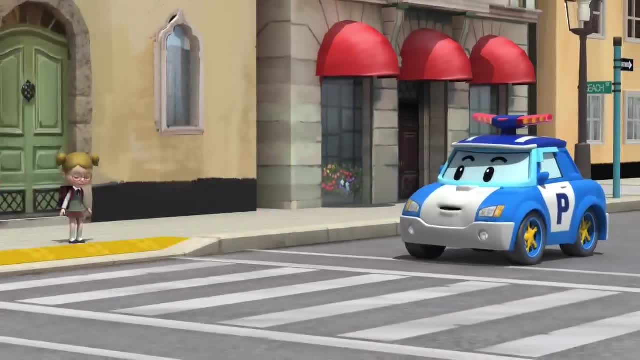 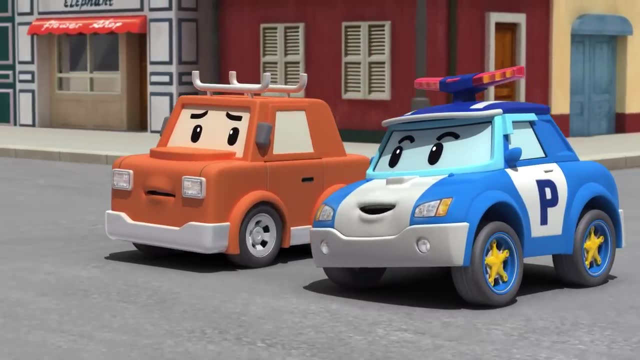 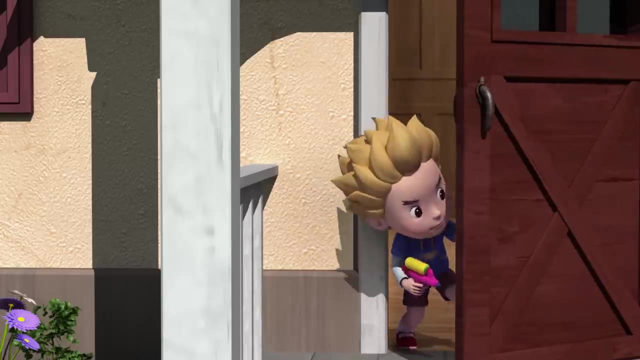 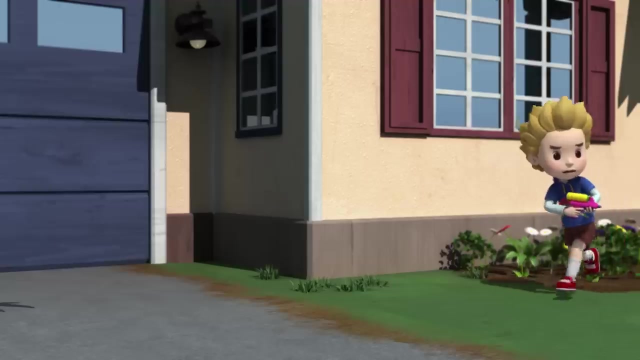 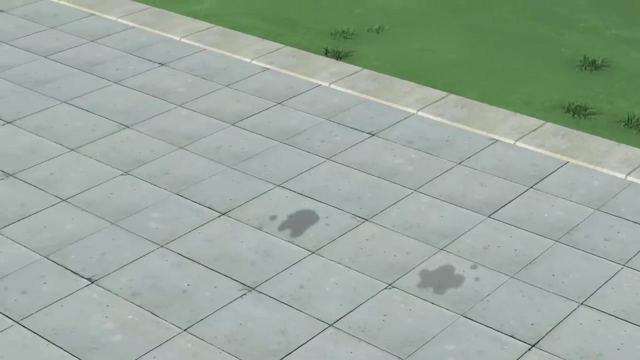 I'll move now. Good, It's safe to cross. Thank you, It looks like you're lost. Can I help you? Yeah, Oh, please. Where could it be? This'll be great. I've got you now, Whoa. 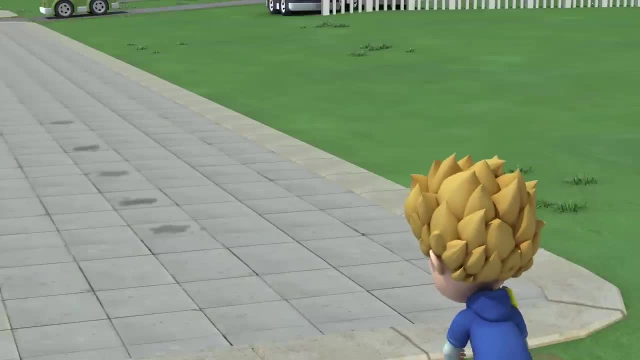 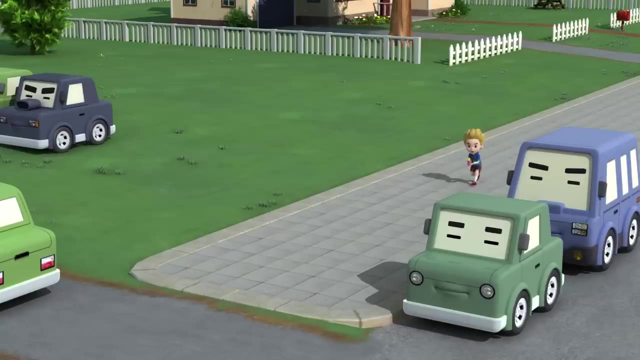 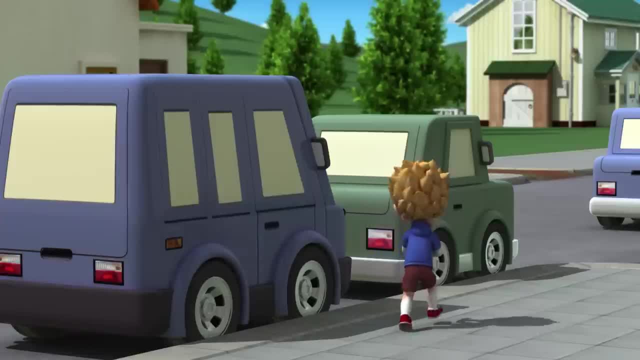 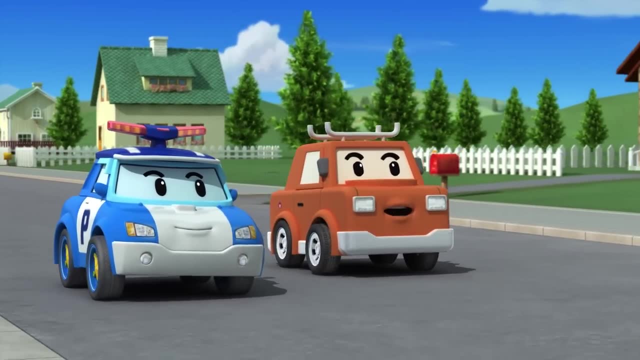 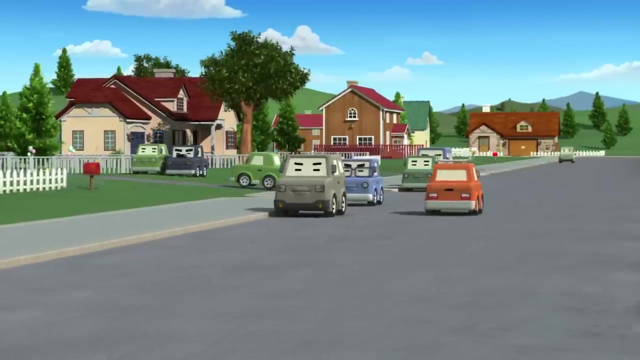 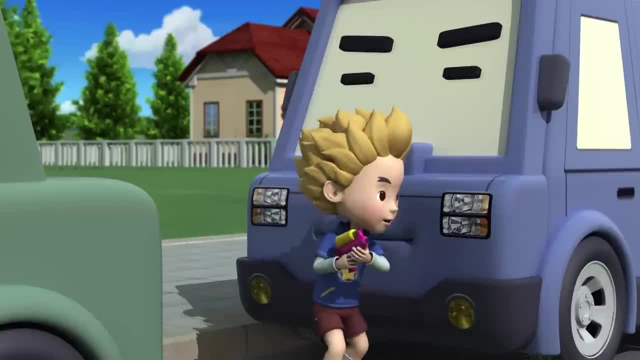 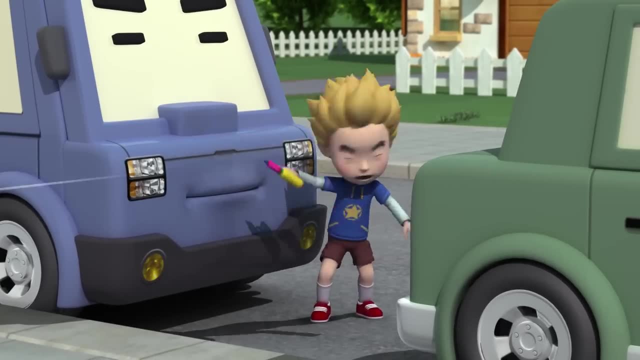 Haha, here it comes, Payback time. Unh, You got me. I g i v u f p. Ariiii, Look out. Ariiii, Ariiii, Ariiii, Arii, Ariiii, Ariiii, Arii. 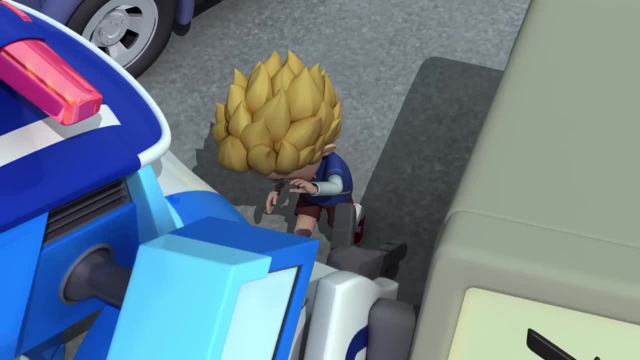 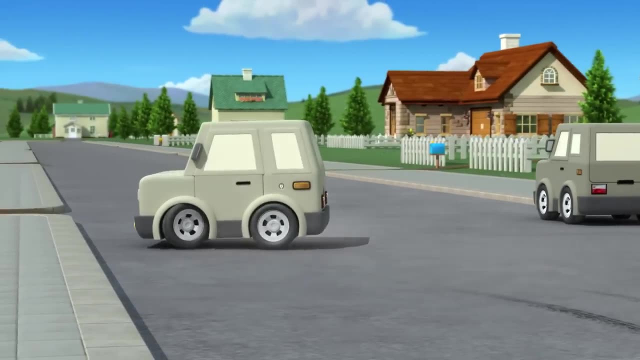 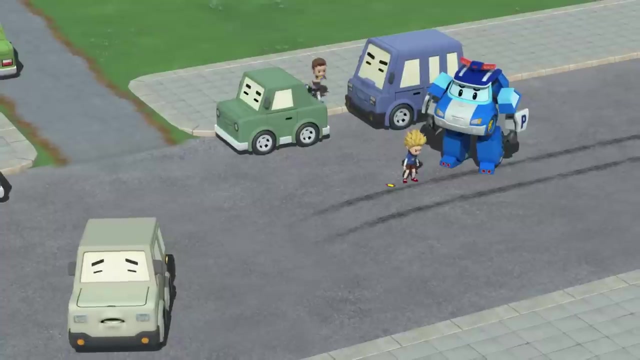 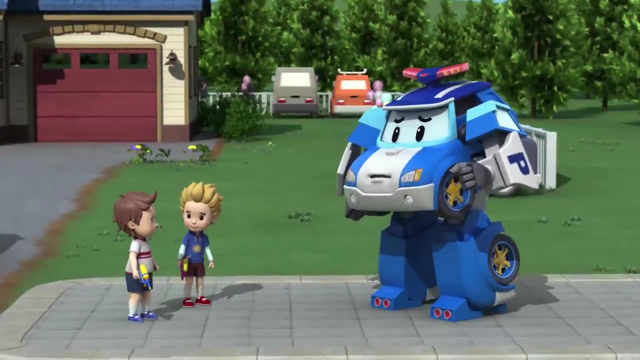 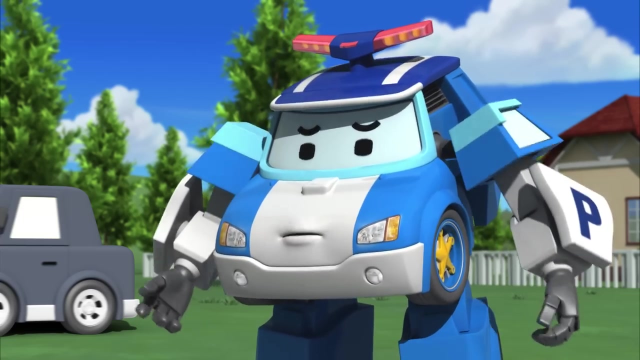 Arii, Ariii, Ariiii, Ariiii. Are you all right, Polly, Kevin and Doug, I can't believe you two just ran out into the road. We're really sorry, Polly. Did you know if you run in between parked cars you're 18 times more likely to get into an accident? 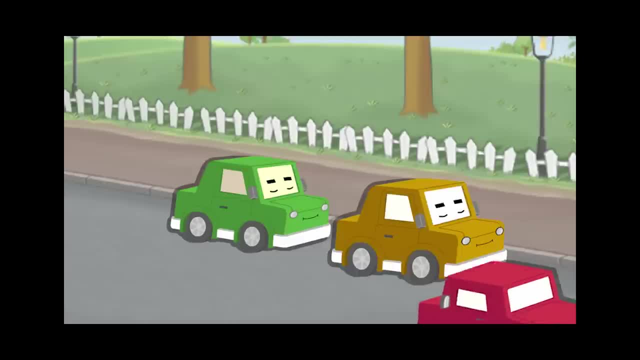 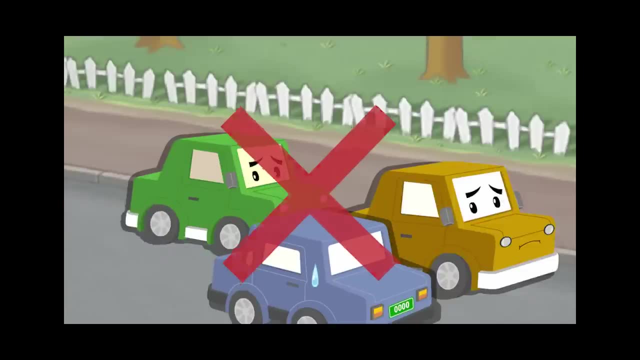 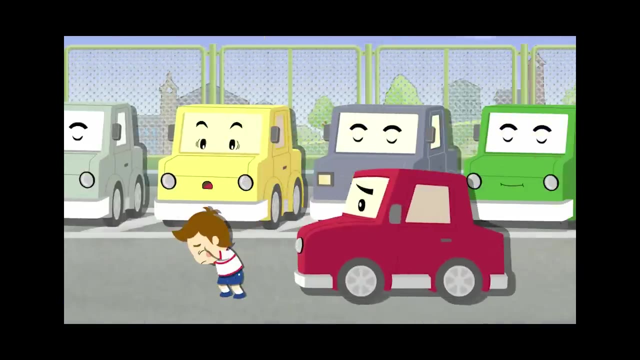 It's very dangerous- Did you say 18 times, Right? If small children like you pop out from between parked cars, it's nearly impossible for drivers to see you in time and you could wind up getting hit. So whenever you have to walk out onto a road, if you're in a parking lot or near cars at all, 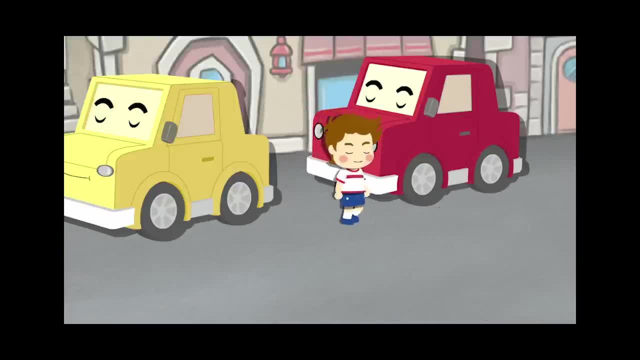 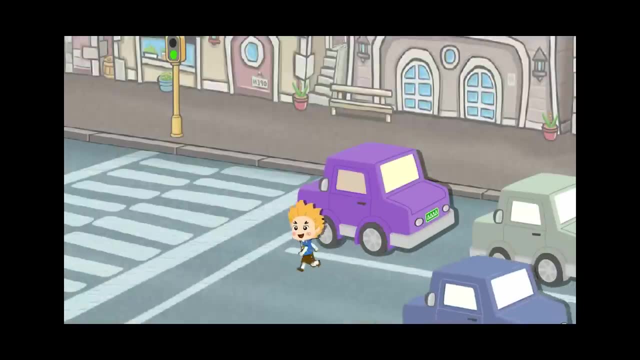 you must look around first and then walk slowly and carefully. Even if you're at a crosswalk, you must never, ever run out in front of a bus or in between cars. Also, since you never know when cars are going to move. 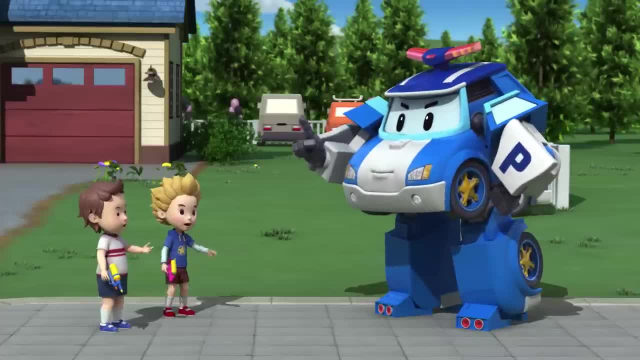 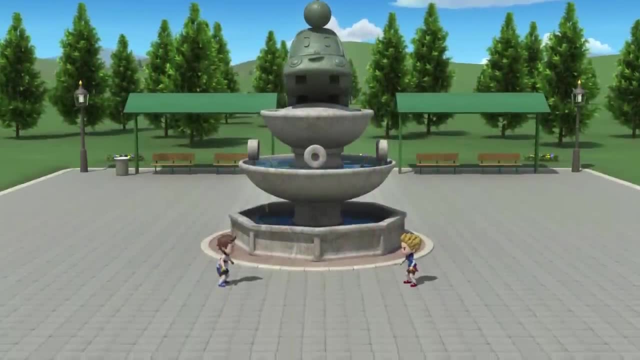 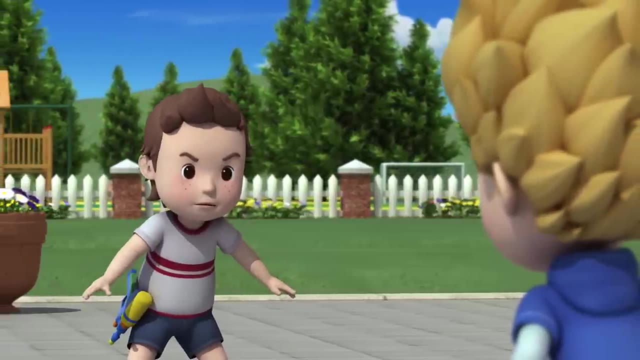 you shouldn't ever play around them, even if they're parked. We hear you, Polly, So we finally meet. It's time for a duel partner. You're on, I'm gonna count up to three, then we draw. All right, partner. 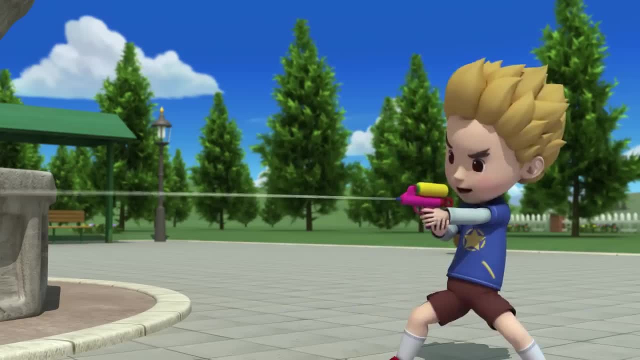 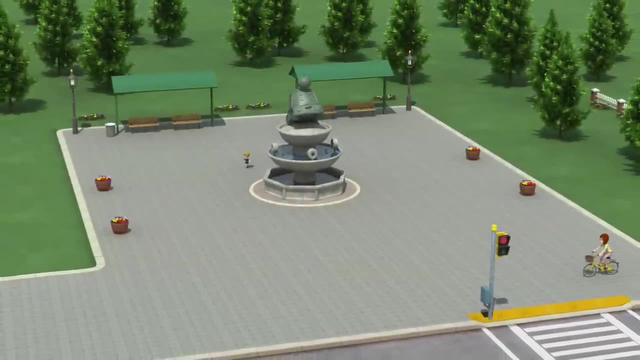 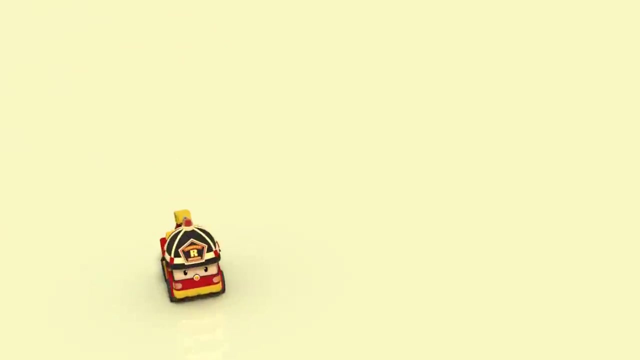 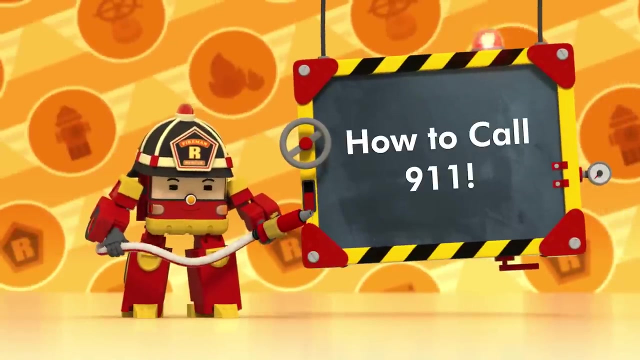 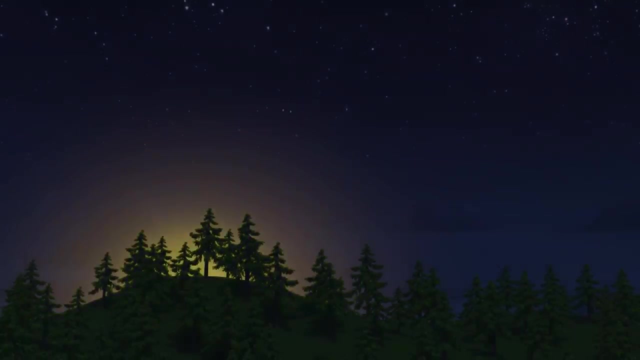 One, Two, Three. How do you like my monster water gun pilgrim? That's not fair, Doug. Come back here you barmits. Come on, Doug, I'll pay that time. How to Call 911? You guys guess what I heard. 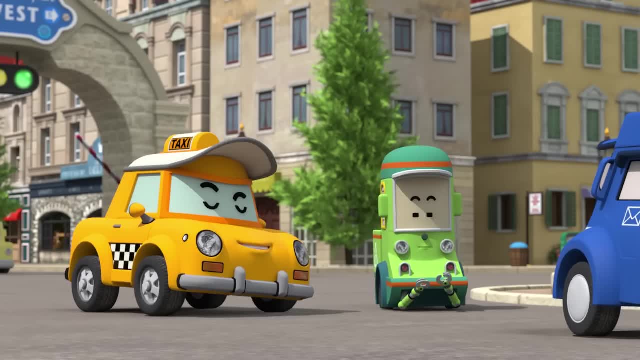 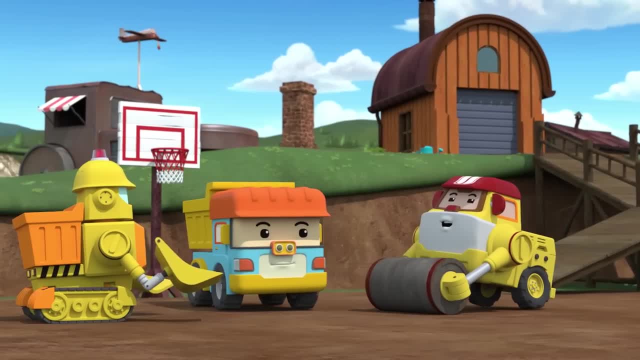 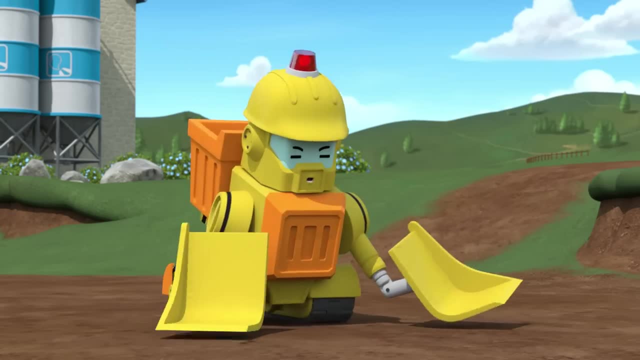 Light everywhere. Yeah, that's right. I've never seen a meteor. What do you think they look like? I heard It's just a rock that falls from space. Just a rock. No way, It's gotta be sparkly like a Super Ball. 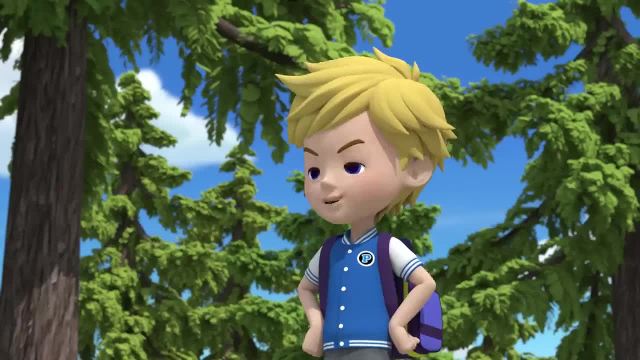 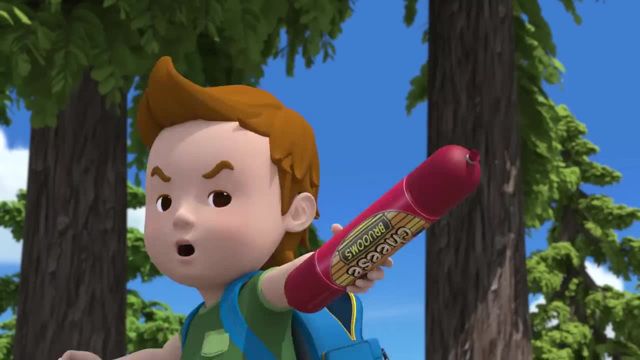 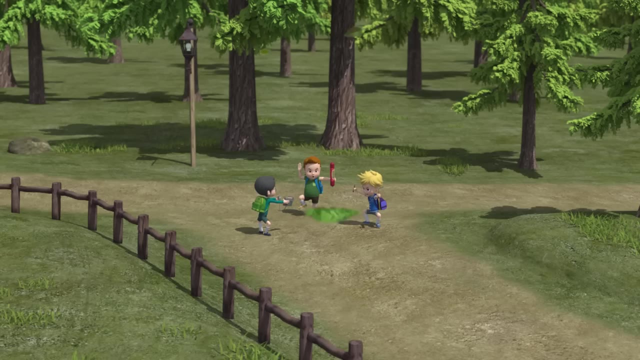 The three of us are gonna get to the bottom of this. you guys, Are you ready? Ready Magic dowsing Rocky to find its energy? a jumbo sausage, cuz we're out here for hours and I might get hungry. alien communicator, ham radio- wait, how are any of those gonna help us find a shooting star? Peter, you just. 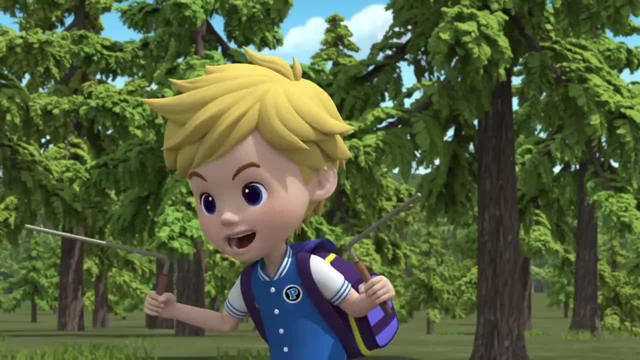 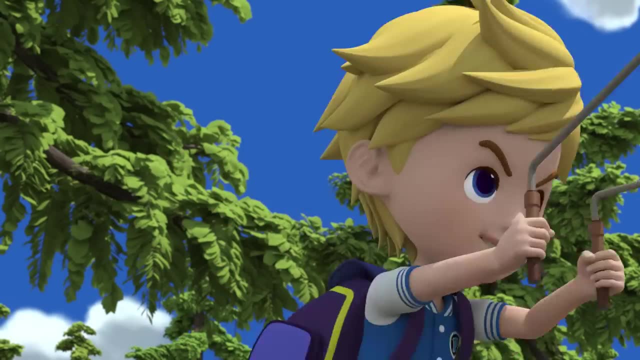 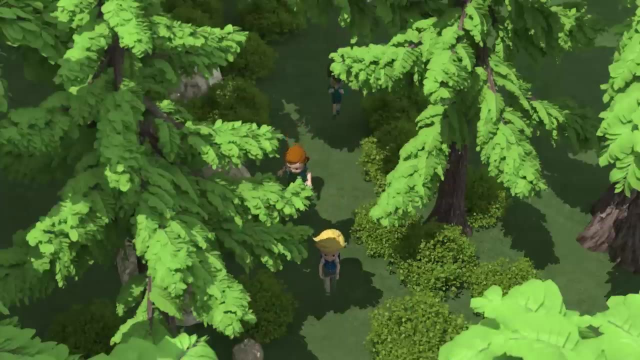 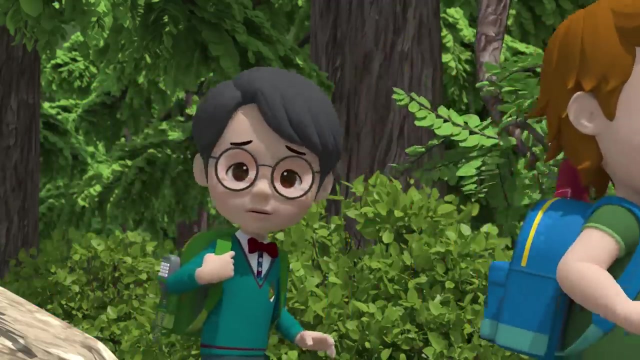 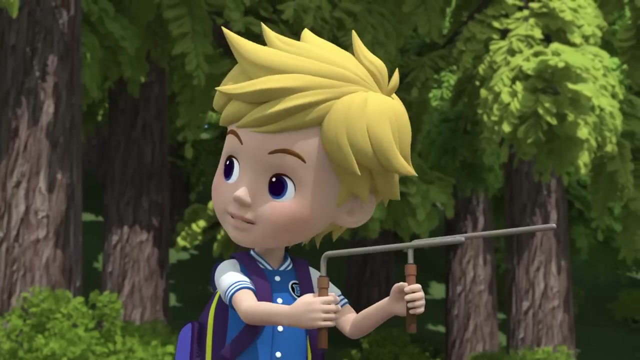 brought sticks and I'm pretty sure you can't eat those. check this out. ha, let's go. super dowsing rods. hmm, I felt it this way. let's go. is he feeling okay, who knows? are you sure this is how to get to the star? of course it is. I totally know the way. so this is still the way. we'll be there in no time. oh. 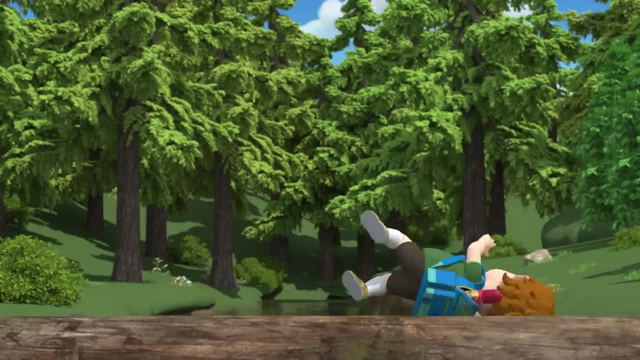 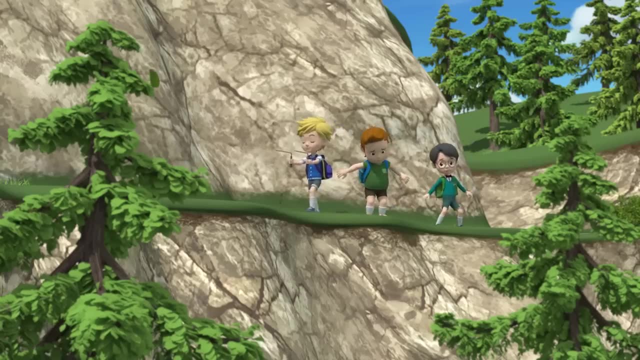 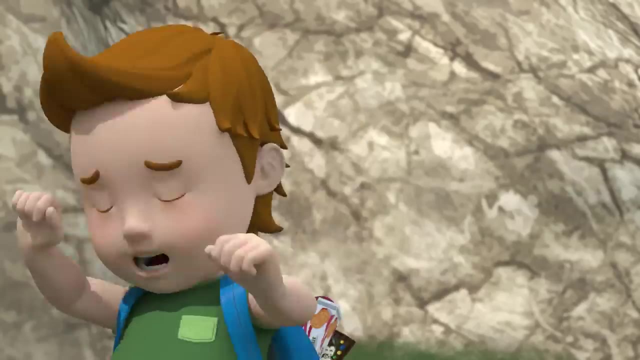 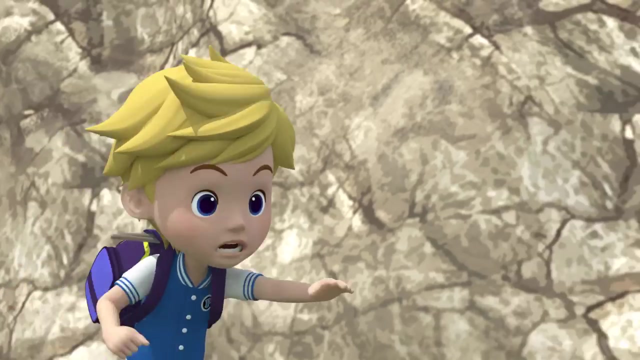 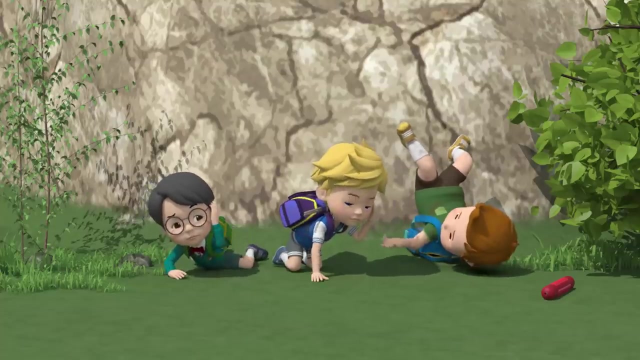 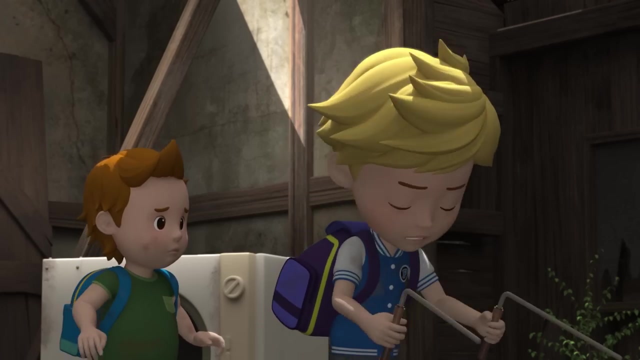 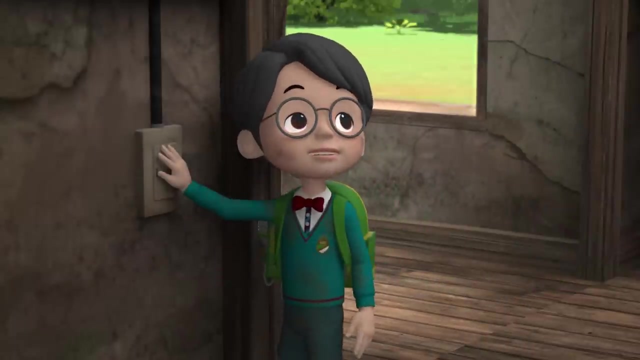 over here. so you're still a hundred percent sure. yes, guys, I keep telling you I got this. don't fall, Peter huh. what is that? it's really dark in here now, but I know I saw something, Charles. is there a light over there, right here, the shooting star? that's gotta be it. 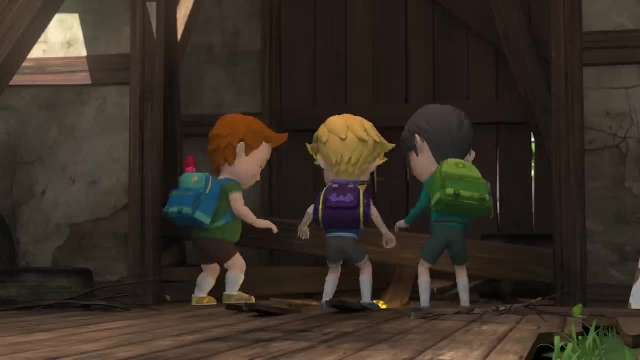 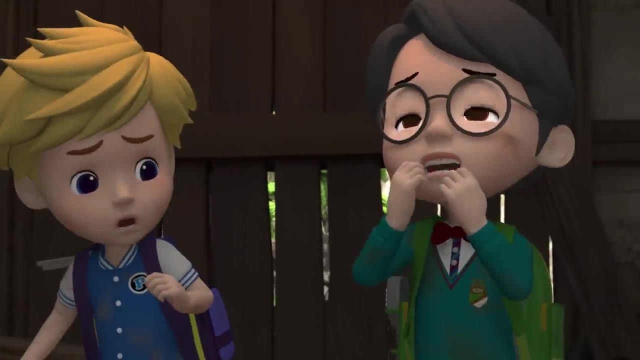 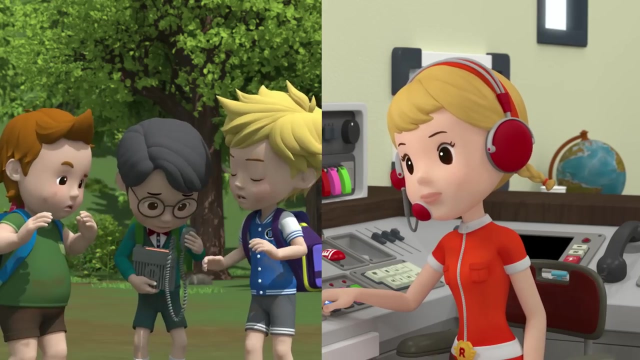 we should call 9-1-1, but I don't have a phone or anything. that's right, your radio thingy. we should call 9-1-1, but I don't have a phone or anything. that's right, your radio thingy. rescue squad: Jim speaking. there's a fire. we don't know what to do. where is it? where are you guys? 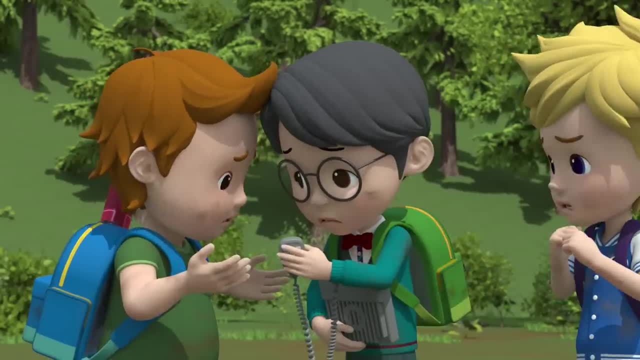 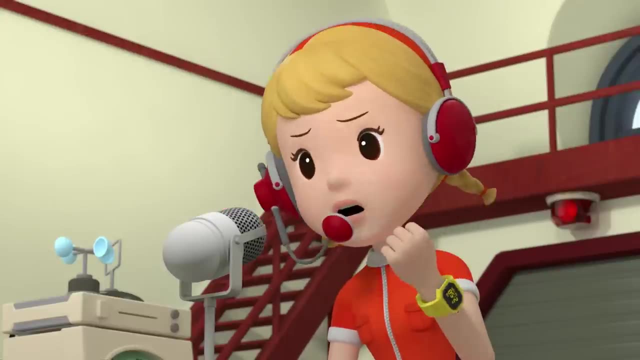 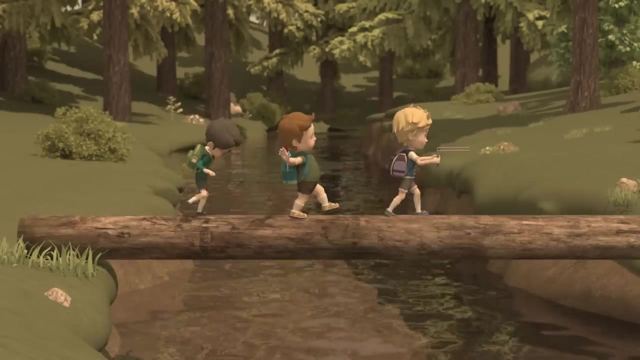 it's an old cabin in the middle of the woods, but I've never been here so I'm not really sure. okay, remain calm and don't panic. describe what's around. do you remember how you got there, God here? well, at one point the road forked and we went to the left, and later we crossed the river. on a log there was. 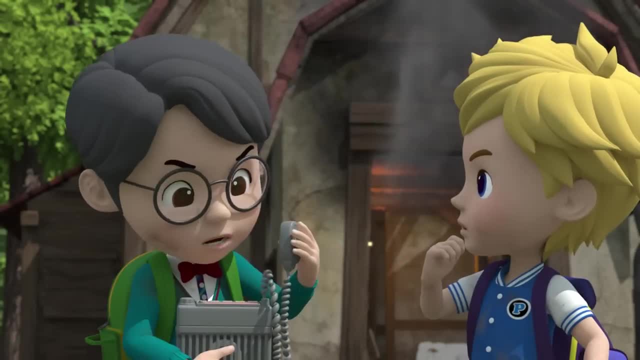 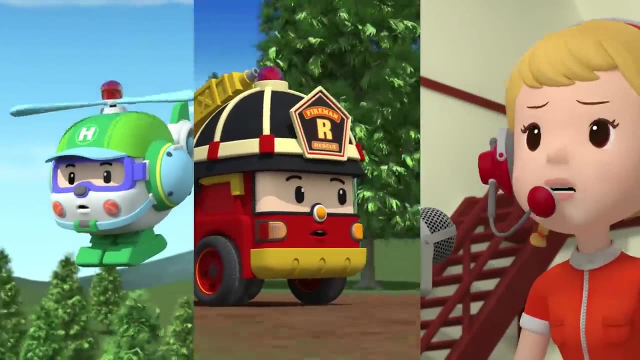 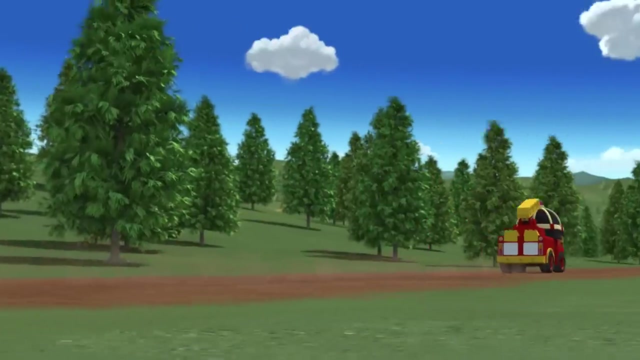 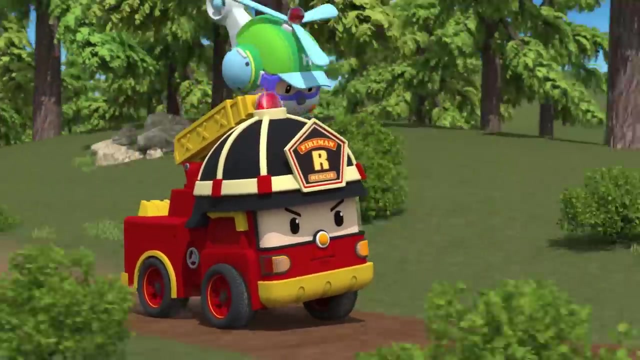 a cliff where we fell off, and that's how we found this cabin that's on fire. okay, heads up you guys. there's been a fire reported in the woods in a cabin. I need you to get there, sending location. now, Heli, I'll head through the forest. you tell me where to go. you got it. 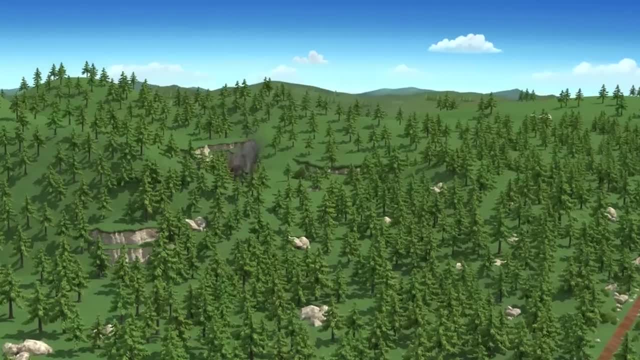 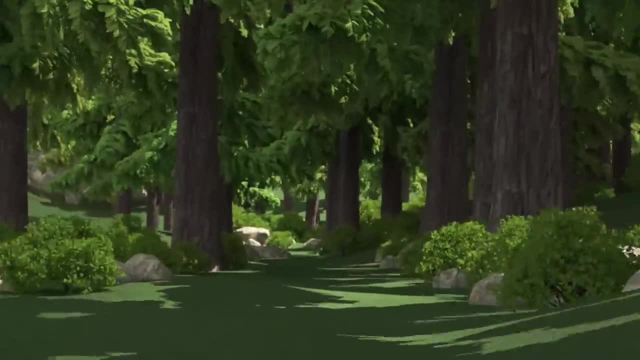 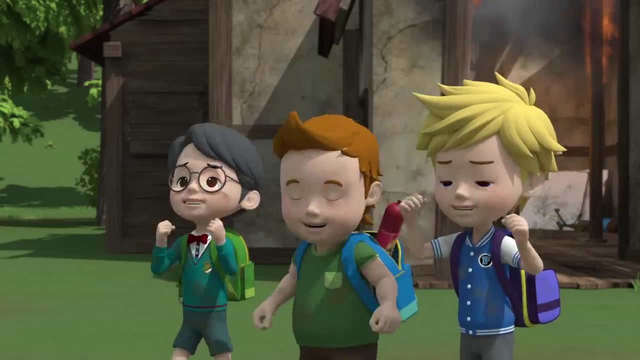 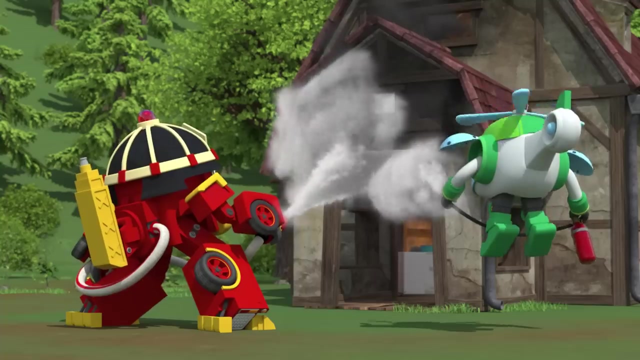 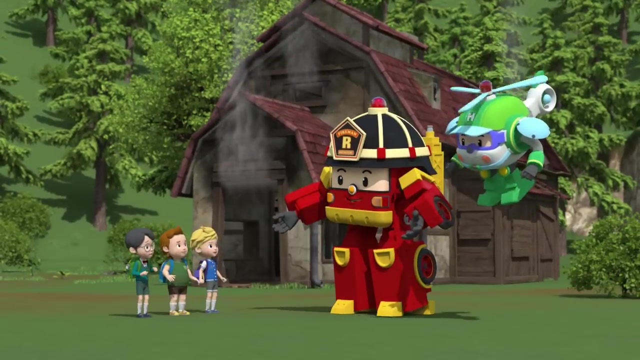 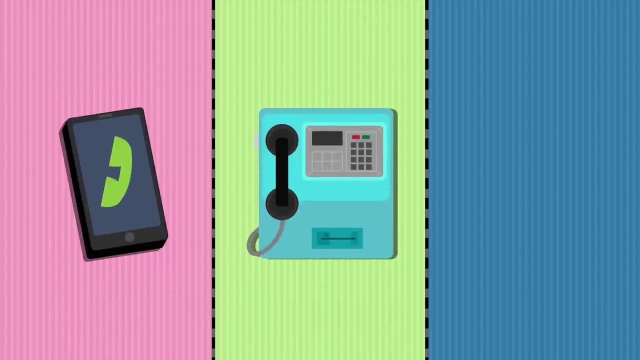 huh, Roy head left. thank you, okay. oh, that's great. so any time you What's happening, Roy? Right, it was me, Raven 호. you see a fire, use a cell phone, pay phone or any other phone and call 911. Always remain. 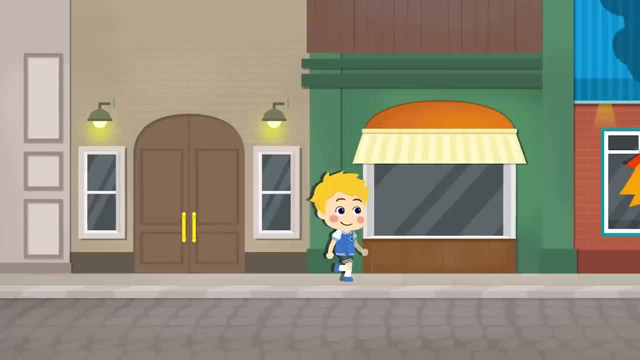 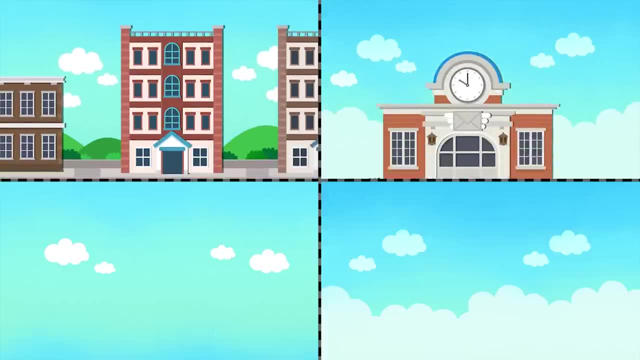 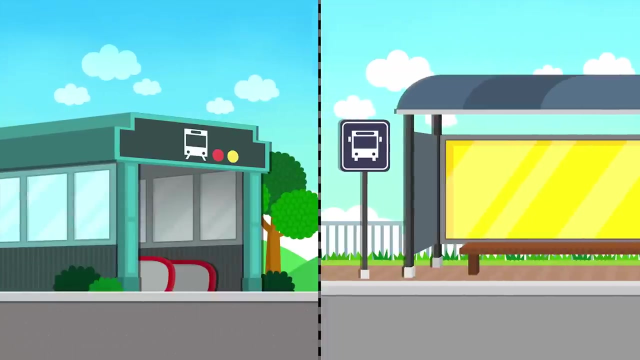 as calm as possible and describe exactly where the fire is. If the fire is somewhere you're unfamiliar with, look around for landmarks. Landmarks can be big buildings, libraries, schools, big trees, intersections, roundabouts, ponds, lakes, subway stations or bus stops. 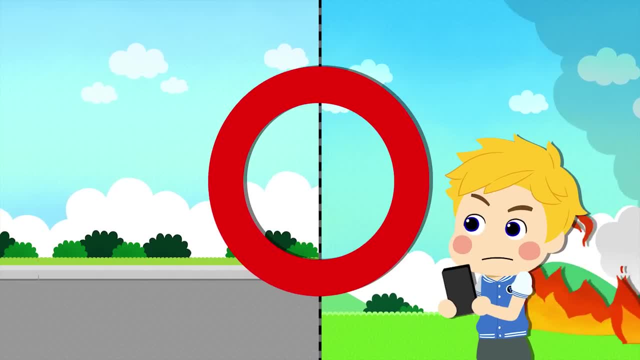 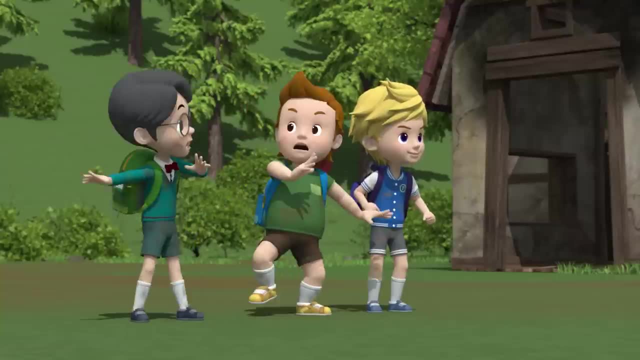 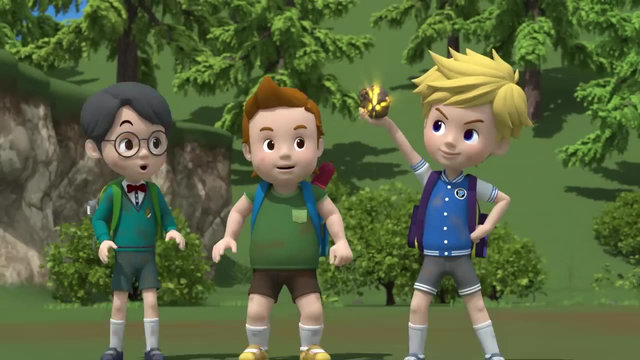 This is so firefighters can find the fire more easily. You understand? Yeah, Roy, Awesome. Why are you guys all the way out here anyway? Oh, the shooting star. Oh no, It would still be inside Ta-da. I remembered to bring it out. 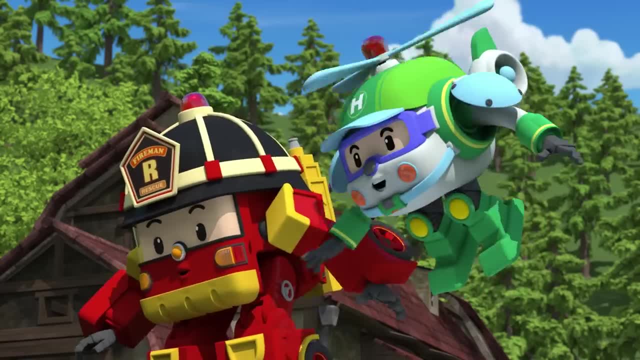 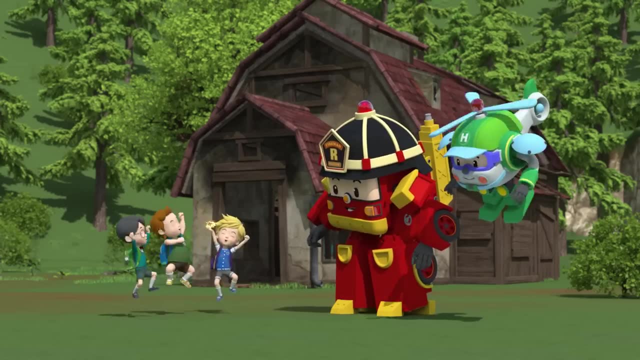 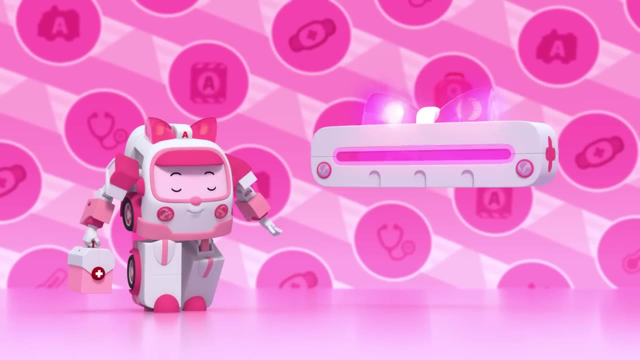 Yay, We got a shooting star. You guys found the meteorite. That's awesome. Everyone's been talking about that. Well done, guys. We found it. Ya-ha, Ha-ha-ha. It's no better time to play it safe. 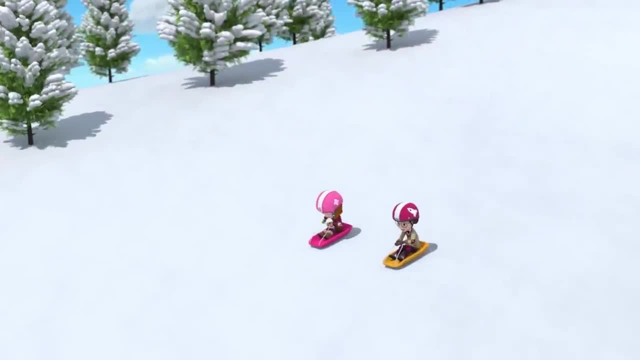 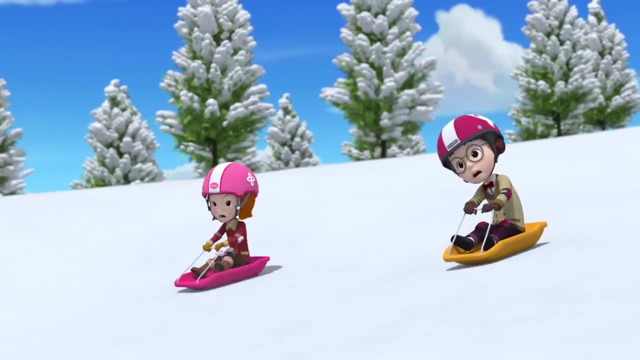 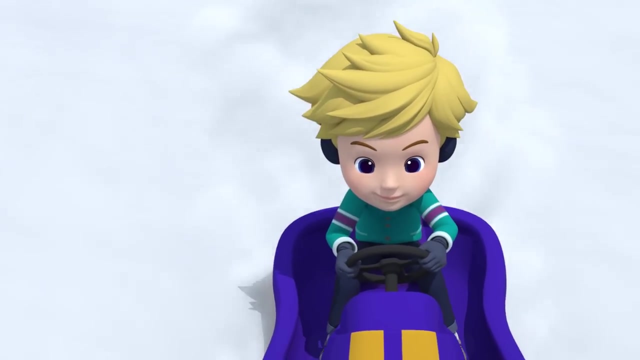 Whee, Yahoo, Woo-hoo. This is great. Yeah, Heads up, Huh, Woo-hoo. Hey, Don't you know? that's dangerous? I'm the fastest person here, here. oh, is that what you think, don't you see? nobody can even match the speed I go. 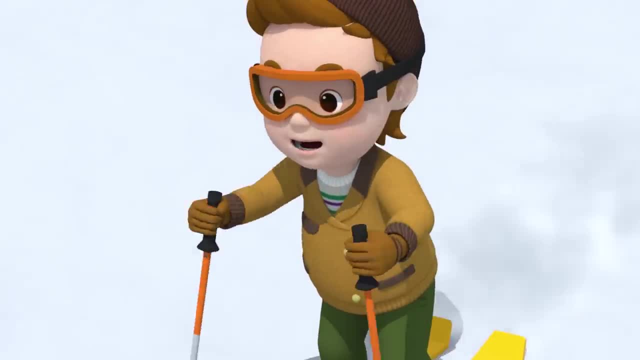 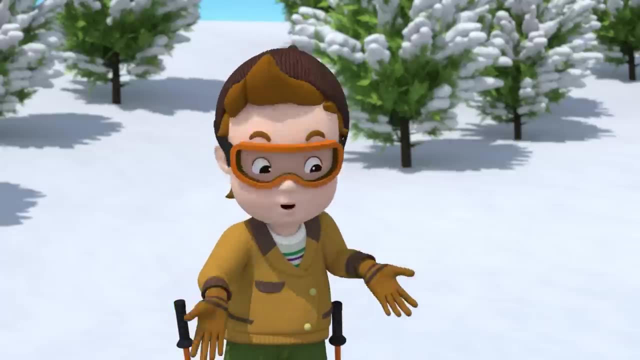 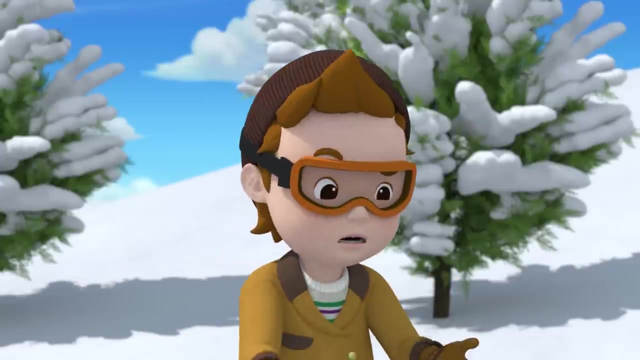 when you fall behind, don't get snow in your face. what? what took you so long? someone's a real slowpoke. slowpoke. I'm fast. you don't know what you're talking about and I don't think that you could ever beat me in a race. hey, come on. I. 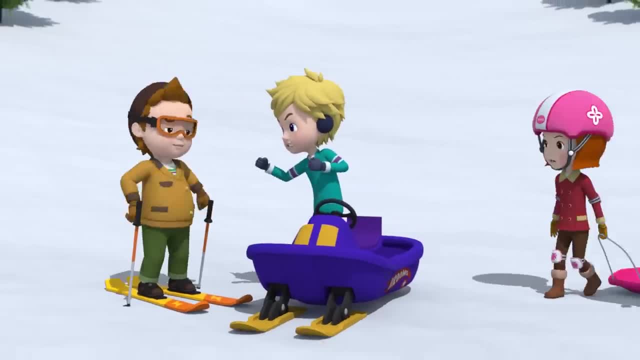 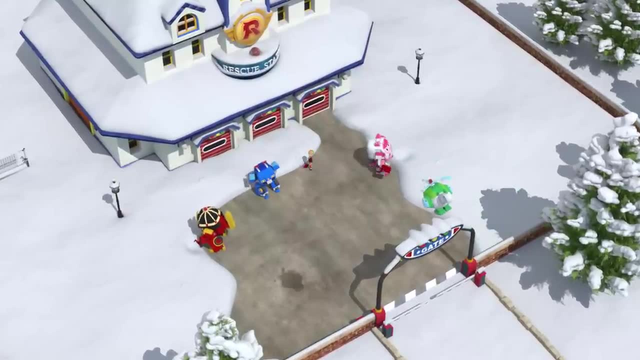 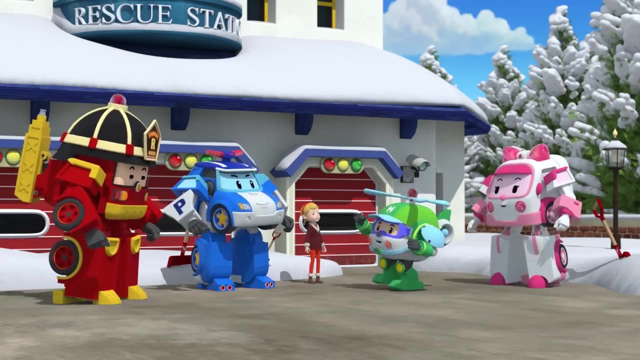 challenge you to a rematch. I look forward to winning again. would you guys stop this? where have you been this whole time? there's so much work to do. let's do it later. the kids are sledding on Apple Street and it looks so fun on Apple. 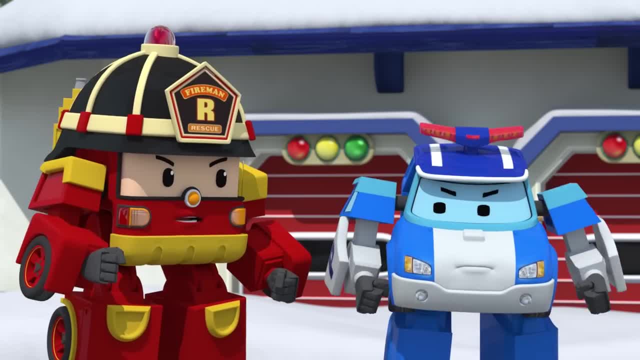 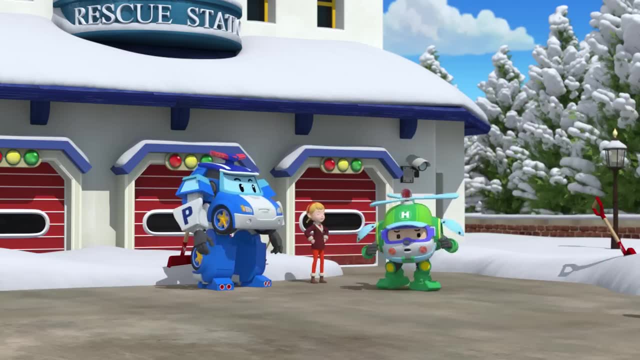 Street till you. that hill could be dangerous. are they alone? they need to be careful going down a hill that steep. I'll go check on them. I'll come as well. oh, I want to come, Kelly, you're going to stay right here until your shoveling is? 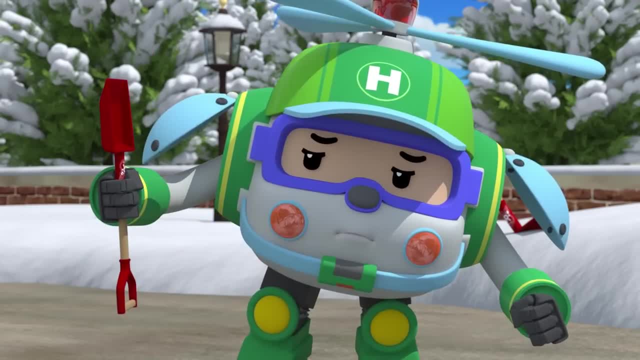 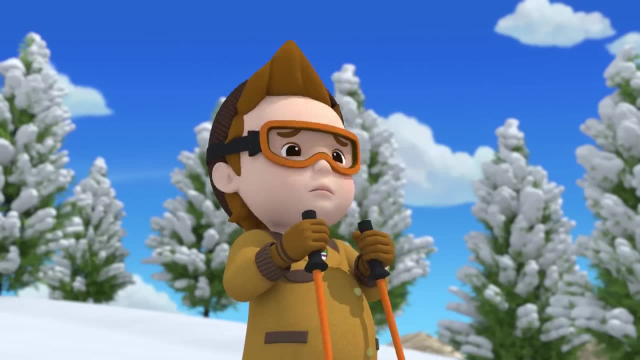 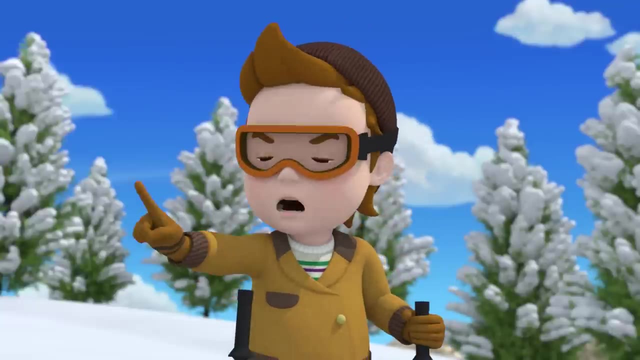 done, hmm, and all I wanted to do was sled. don't you think this hill is a little tall? oh, my school is so steep. is someone chickening out now? I'm not scared. one, two, three and then we start. when you're out, now, I'm not scared. one, two, three and then we start. 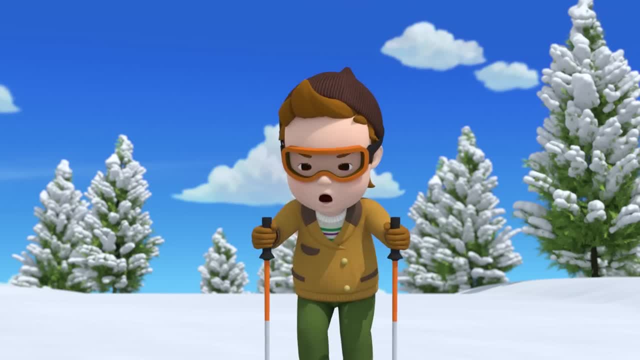 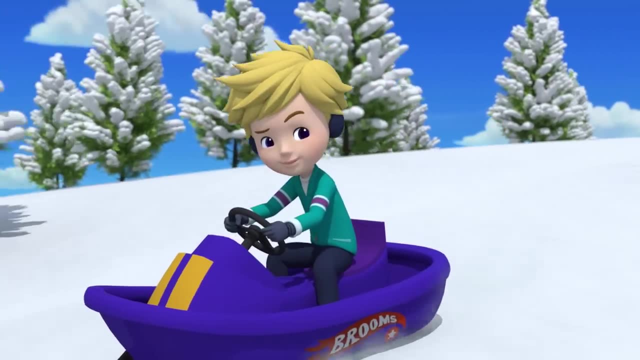 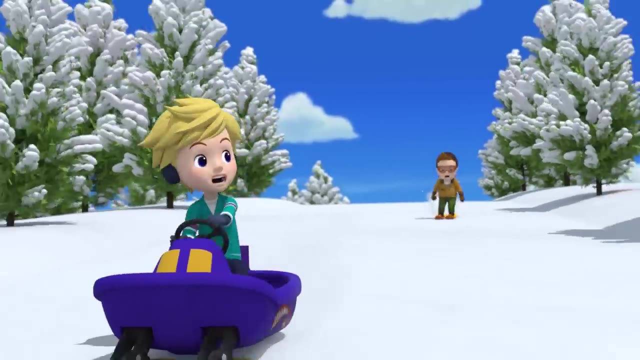 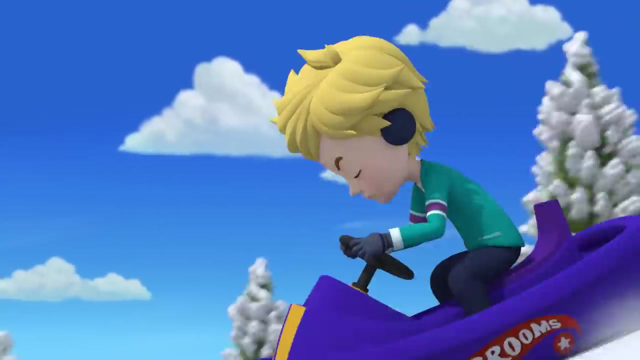 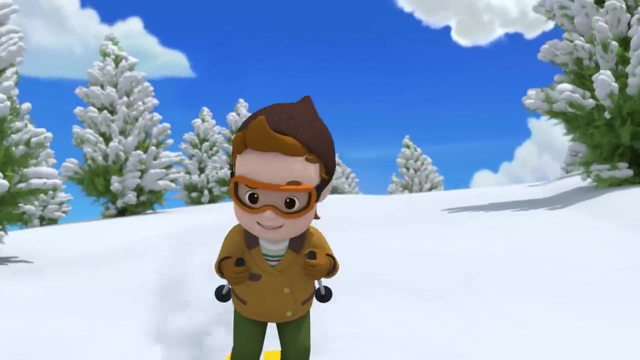 okay, oh yeah, one, two, smell you later. hey, get back here. I can't lose. okay, I'll go get my stuff. if someone gets in the way I have to get in my way, Look who's still the fastest Me. Sorry, what was that? 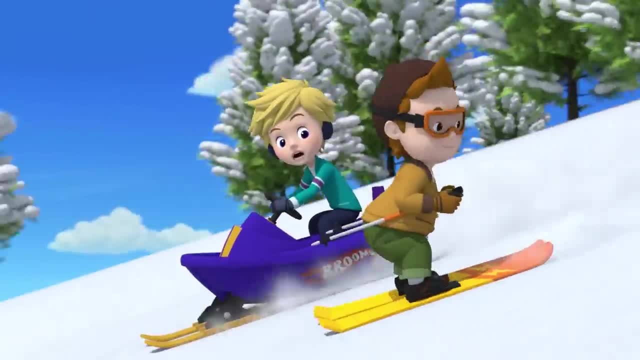 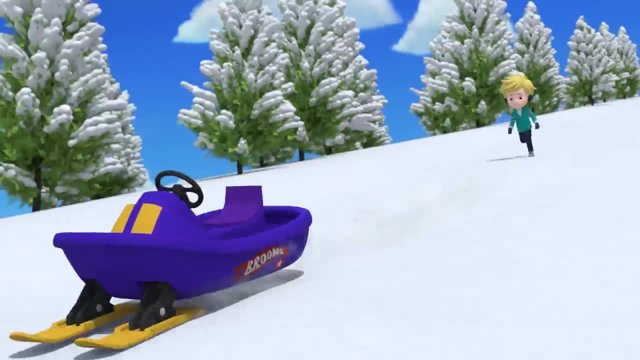 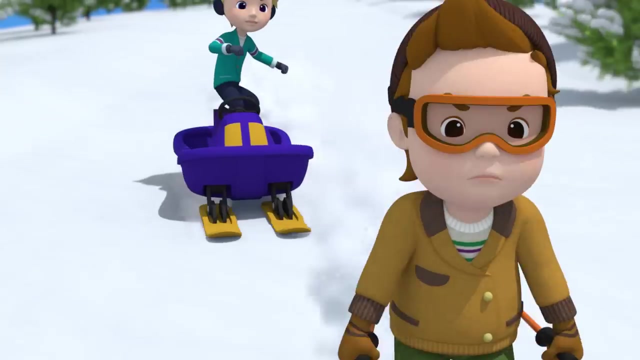 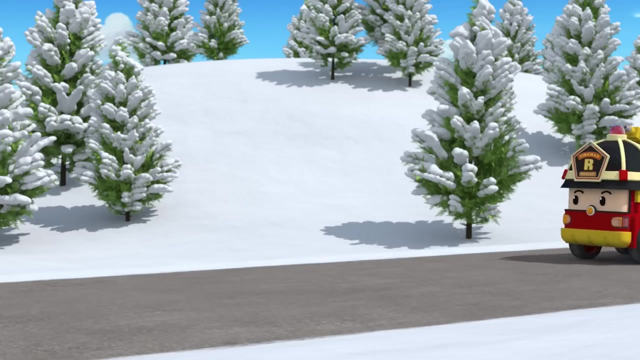 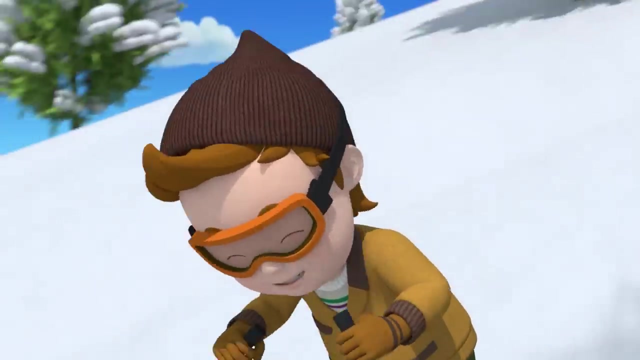 Sorry, Johnny, See you at the end. Just admit, I win. No way. Where did Helly say the kids were? Oh goodness, How fast are they going? Ten bucks says I win. Huh, Oh, Johnny, watch out. 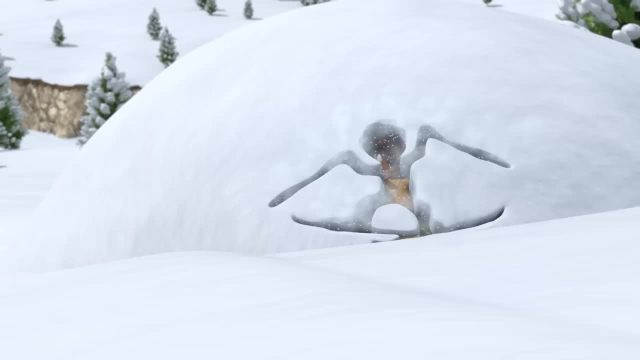 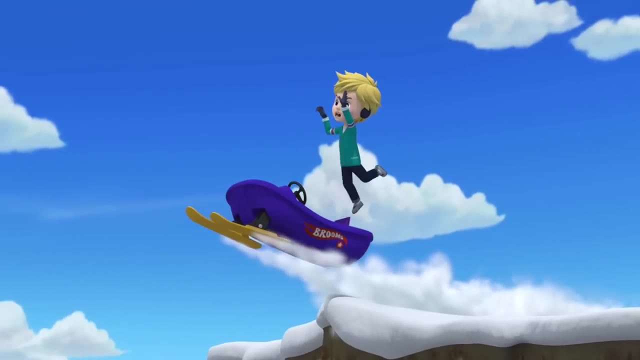 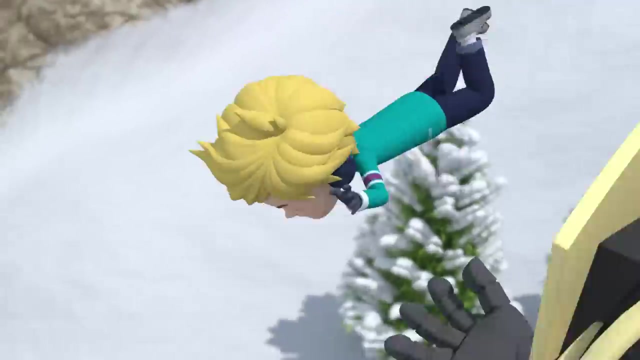 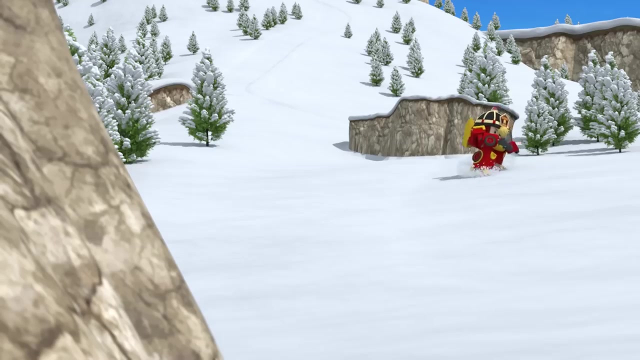 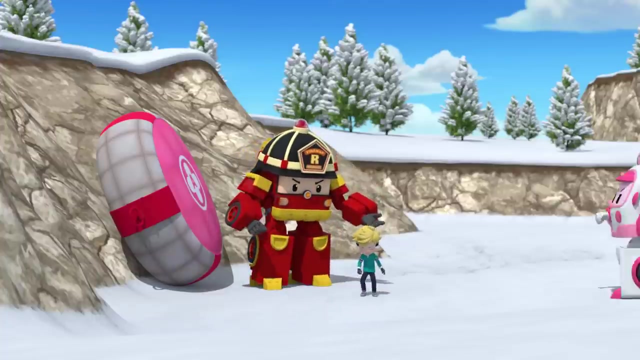 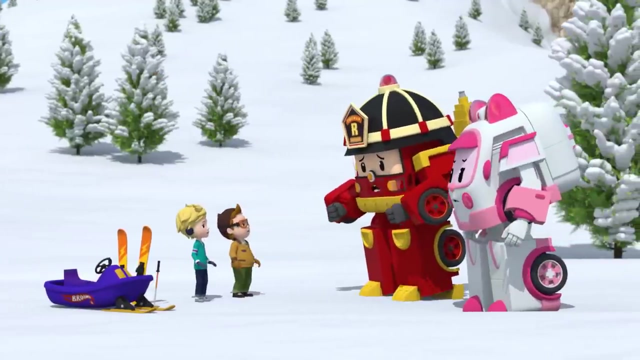 I'm not falling for that. Victory is mine. Look out, Peter, you all right. Yes, Roy, Thank you Listen. don't you know how dangerous that was? You two could have gotten away. You could have gotten really badly hurt. 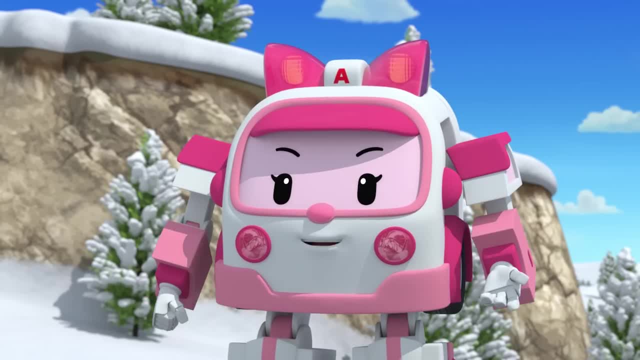 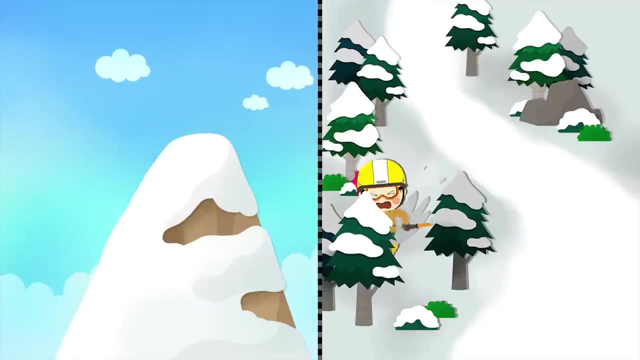 We won't do it again. Roy, You guys, I know skiing and sledding can be a lot of fun in the winter, but you must remember: don't go anywhere that looks too steep or isn't a designated trail. Stick to slopes that were designed for you. 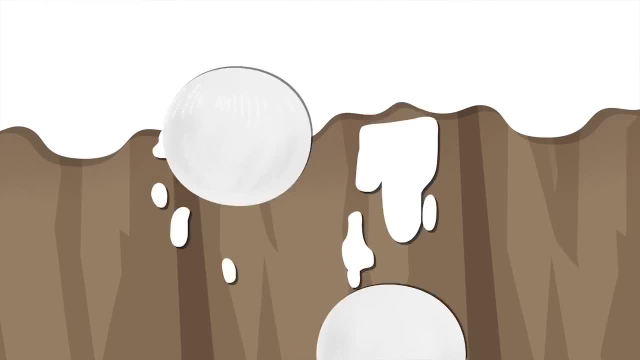 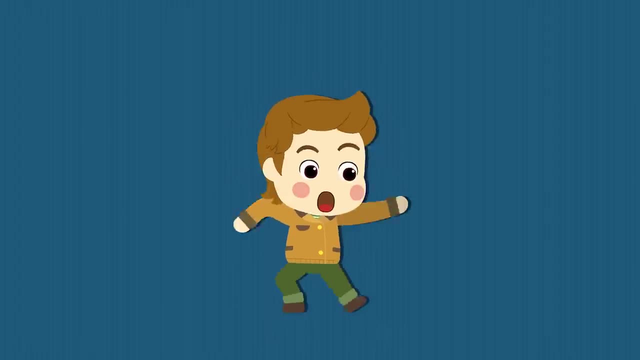 Racing can be dangerous because you go too fast or don't pay attention. Ride together and always stay focused. Before doing winter sports, make sure your body is stretched and ready for action. Always remember to wear a helmet, knee pads and gloves for protection. 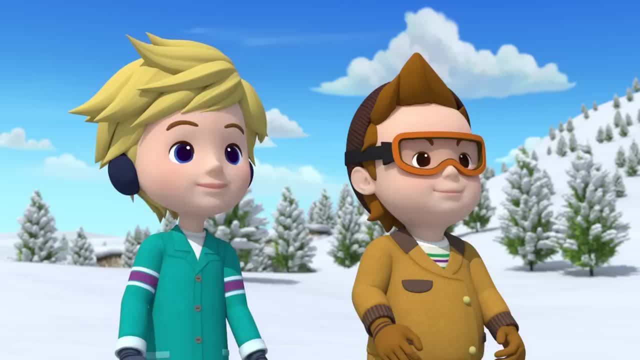 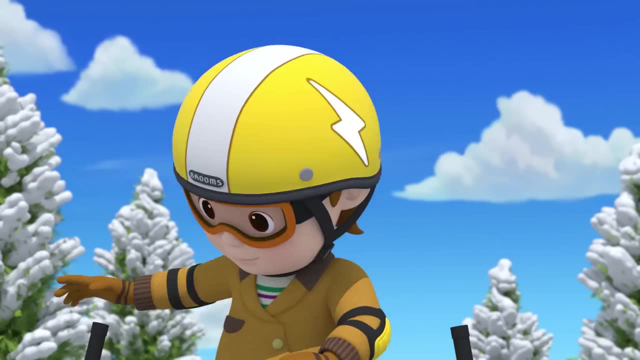 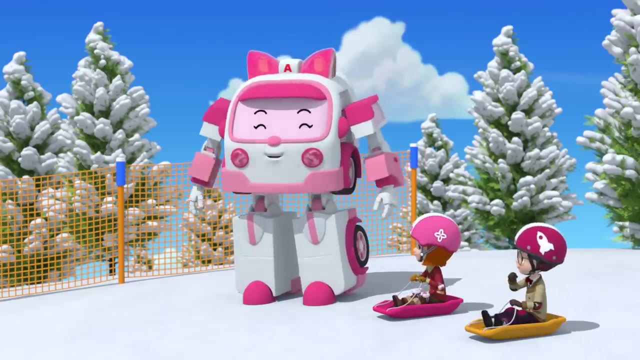 Remember that safety is always the most important thing. Yeah, We'll do better, Amber, Heh, Hmm, Everyone ready? Yeah, So let's ride. Finally sledding time. Helly, I don't remember saying you were done. 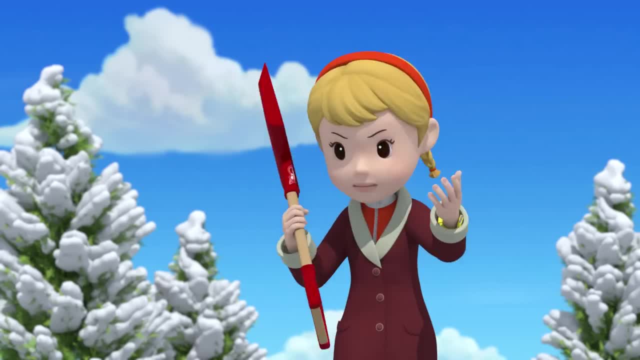 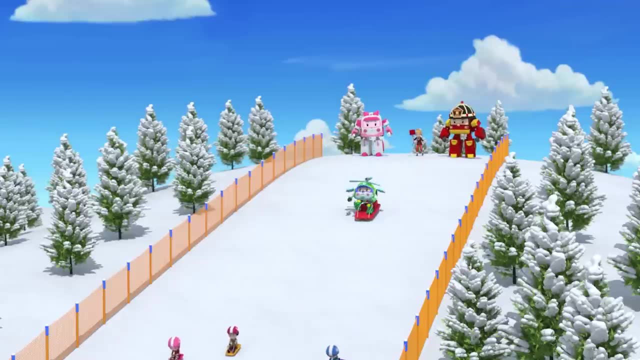 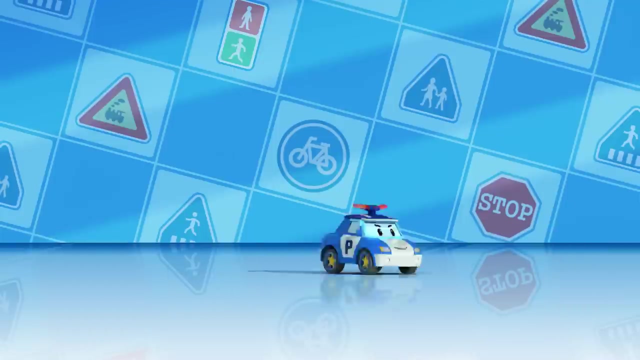 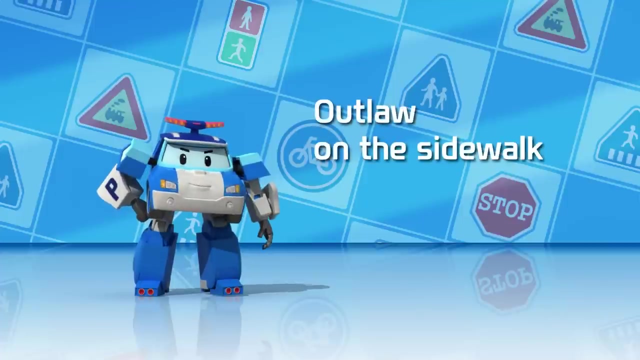 Uh, but but I I just want to sled. Helly, Get your rotor back here now. Outlaw on the Sidewalk. This is a fun ride. It's fun, right? I think we'll go back to the sidewalk. 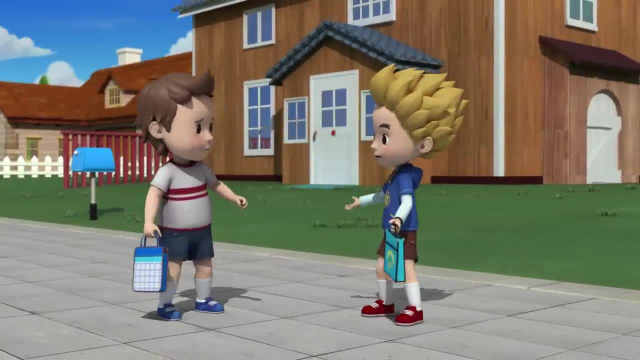 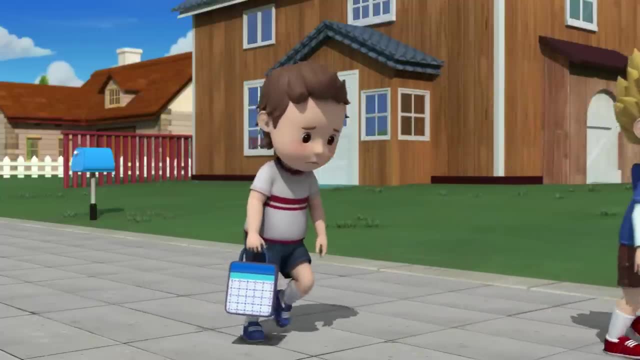 Ah, I really don't like homework. Yeah well, I'm so hungry. Doug, why don't we go play for a little while? We can't. If we're late, Jenny will be mad. Yeah, you're right about that. 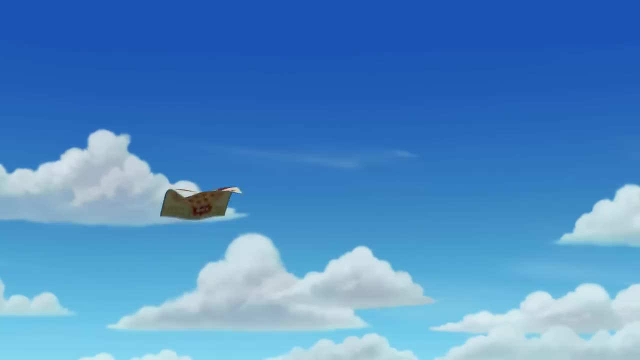 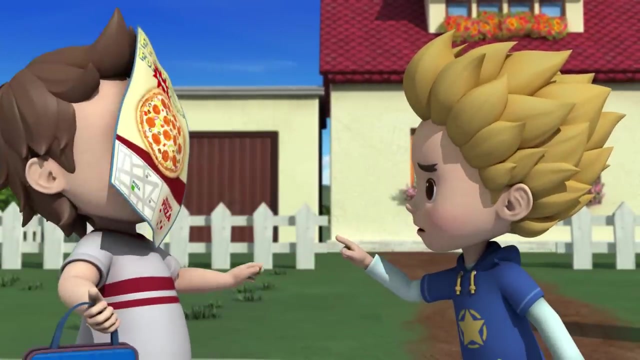 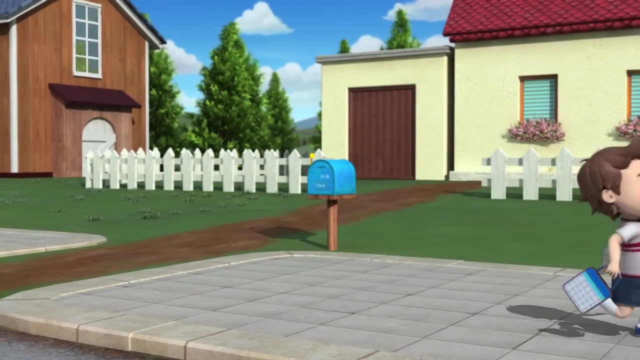 Ugh, Hmm Pizza. The first 100 customers get free pizza today. What Free pizza? Yeah, Let's go get some. Uh, hang on, But Jenny's still waiting for us. If we bring her some pizza, I bet she won't mind so much, right. 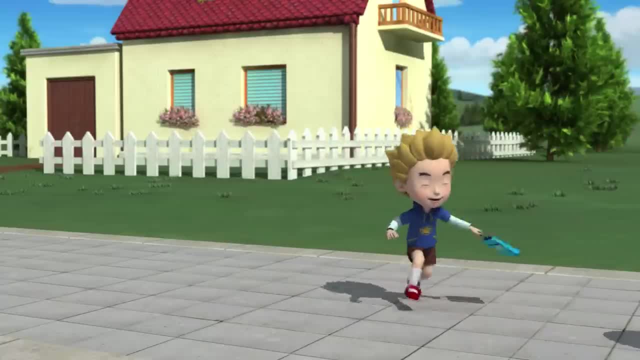 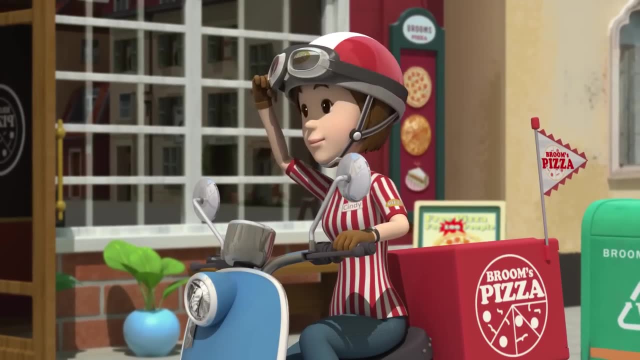 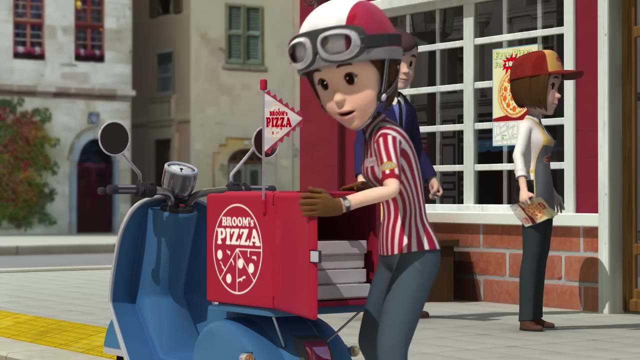 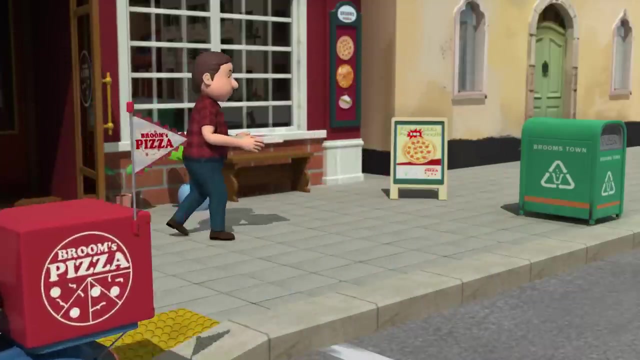 You think so? Of course, Excuse me, please Pardon me, sir. Wow, there's no time to rest today. Okay, pizza's on the way. Kevin, are we almost there? Yeah, we should be just about there. 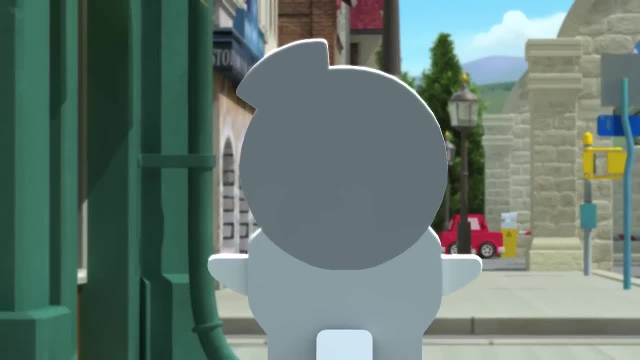 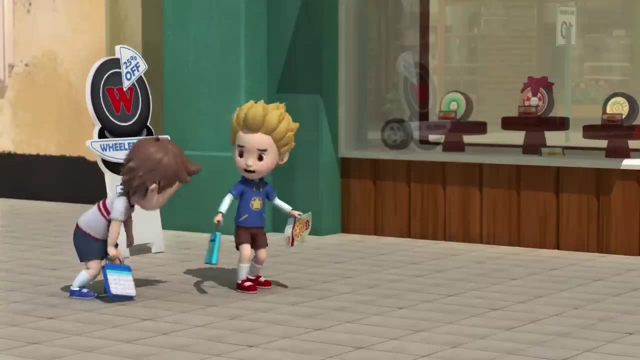 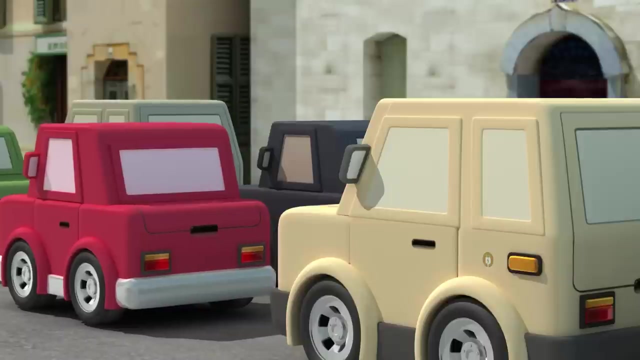 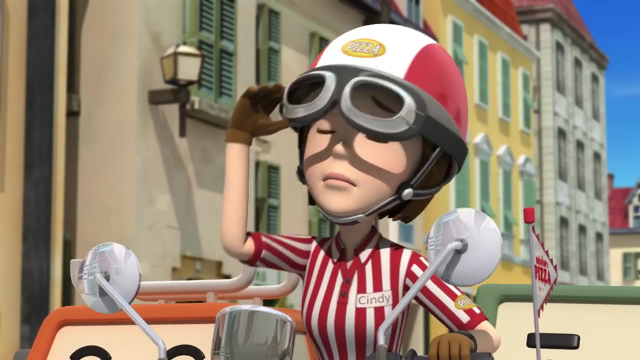 Let's see. I think it's right around here. We found it Time to go, Time to go Time to eat. This is not the right place. We got tricked by that sign. Wow, traffic is so bad. Well, in that case. 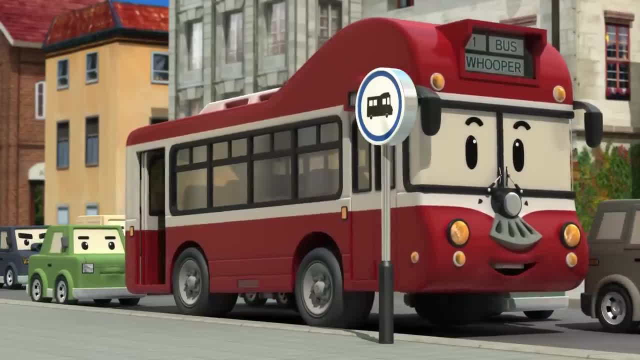 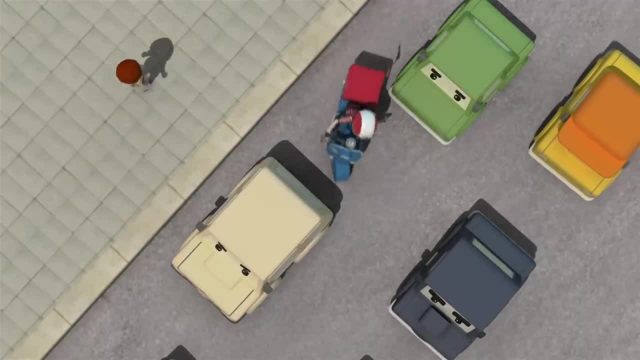 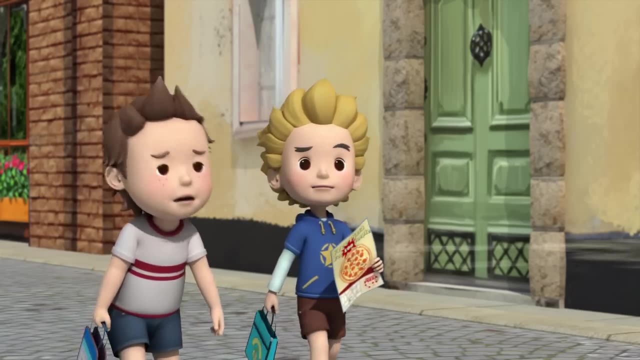 There. Okay, this is 7th Street, Sorry, Huh, Huh, Uh, Uh, Uh, So I'm pretty sure we're just about there. Um Huh, Hold on. Huh, I can smell it. Kevin, I can smell it. 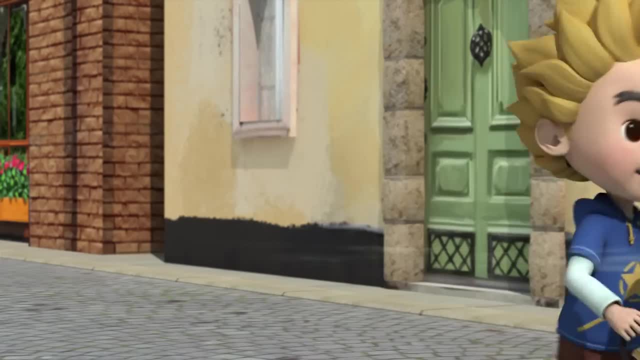 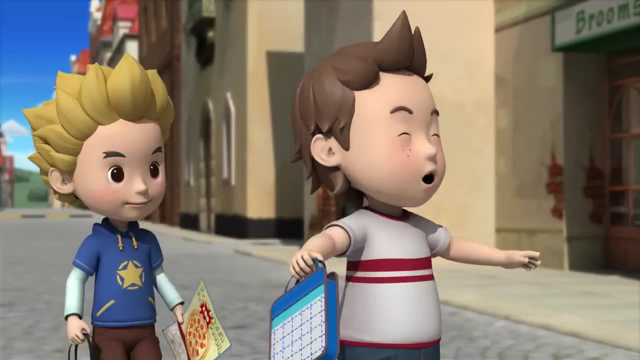 You go. Doug Your nose is never wrong. Hahaha, My nose says that we're getting close. Oh, Oh, Oh, Huh, I found it. What. That's awesome. Where is it Where? I'll take a hot dog, sir. 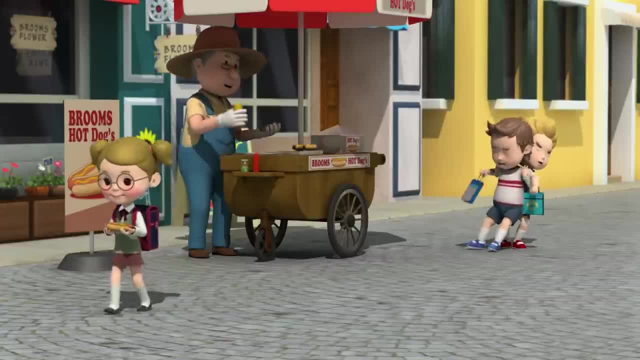 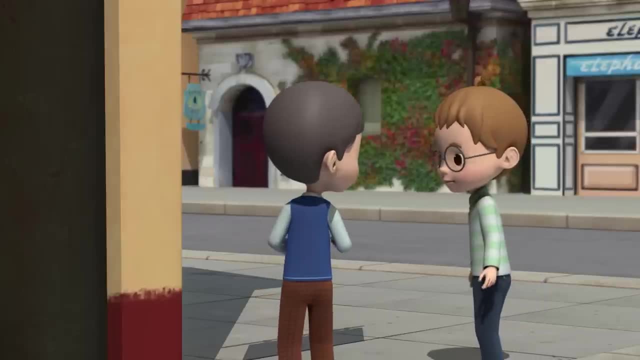 What I'll take a hot dog, sir. Awesome, Get moving, Doug. We're going to miss out on the free pizza. Hot dog, come back. I think we're almost there. Are they really giving away free pizza today? 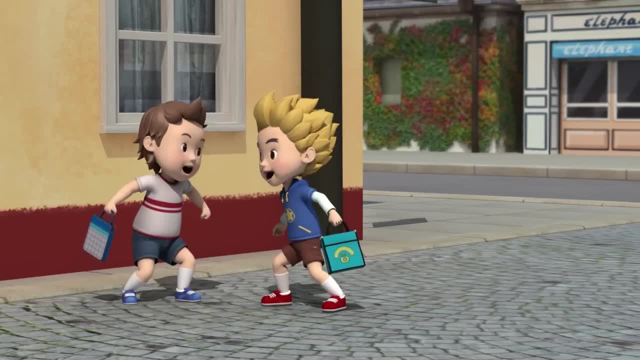 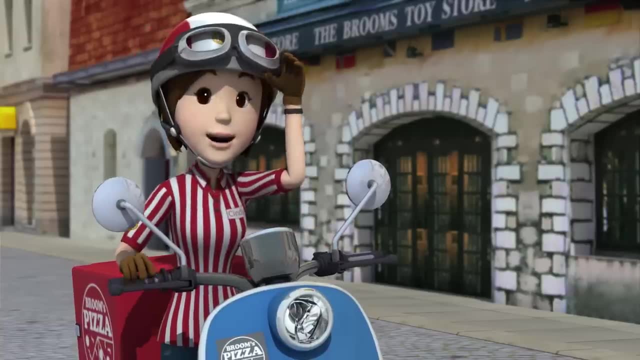 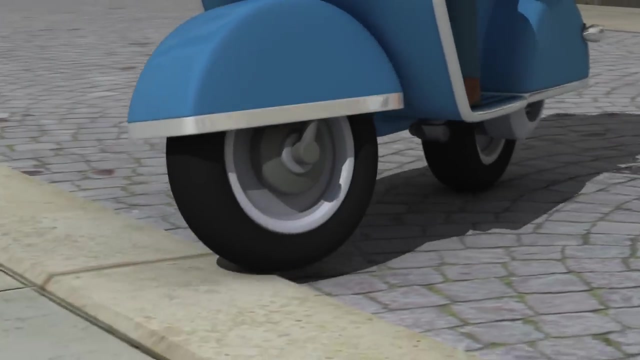 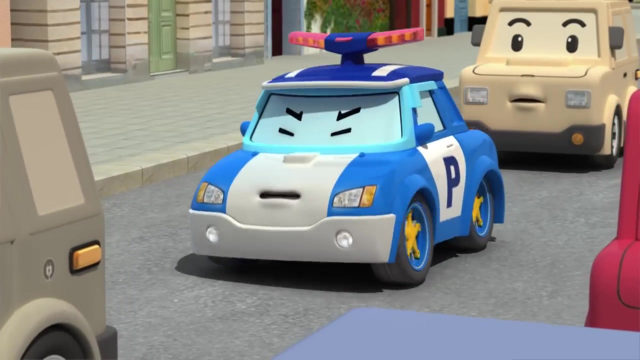 That's what I heard. Huh, Alright, This way, Come on, let's go. Phew, I've just got one more pizza to go. Should be around here somewhere There. Huh, Why is that scooter on the sidewalk? 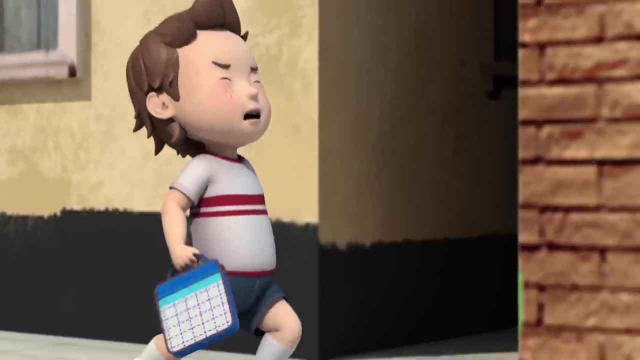 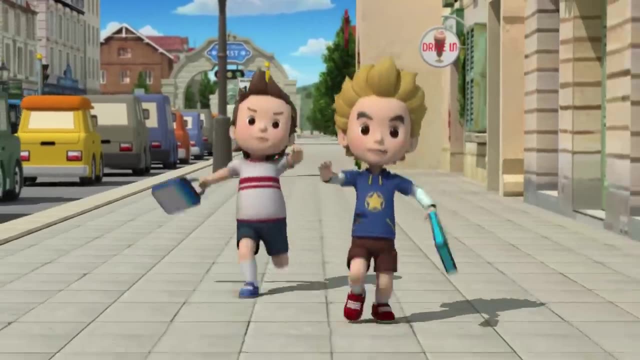 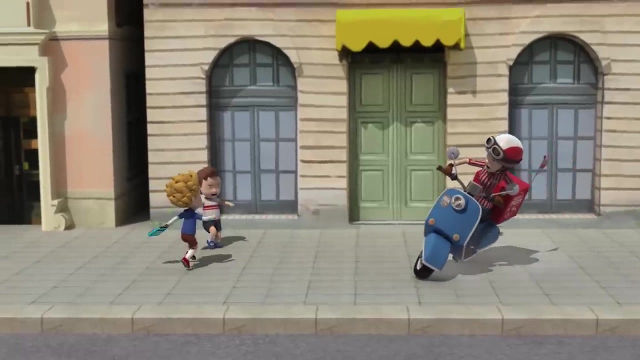 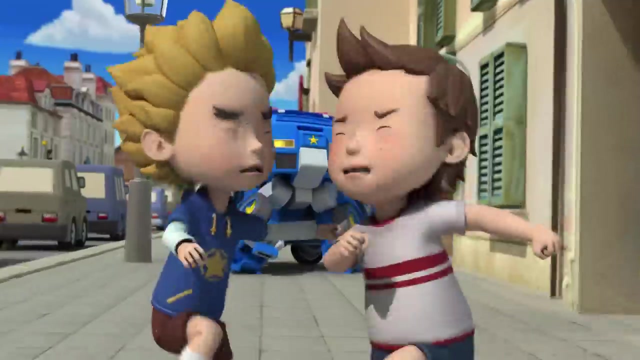 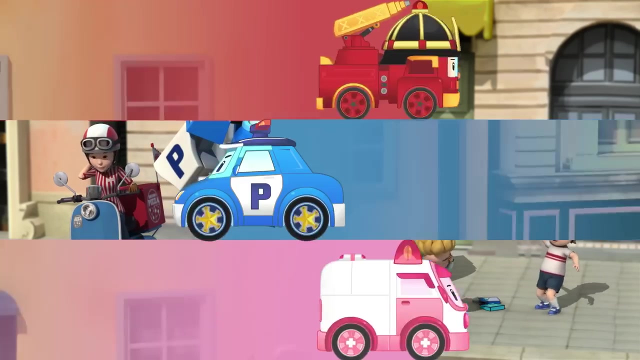 Try to run faster. We're almost there, Do you promise? Huh, It's a scooter. Hold on, Huh, Huh, Are you two alright? Why do I see two of everything? Don't you know? Motorized vehicles should never be driven on the sidewalk or on crosswalks. 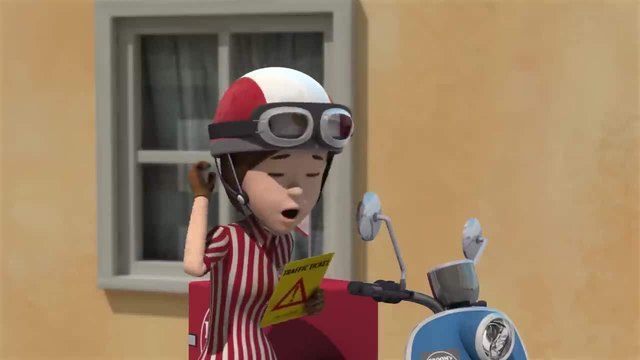 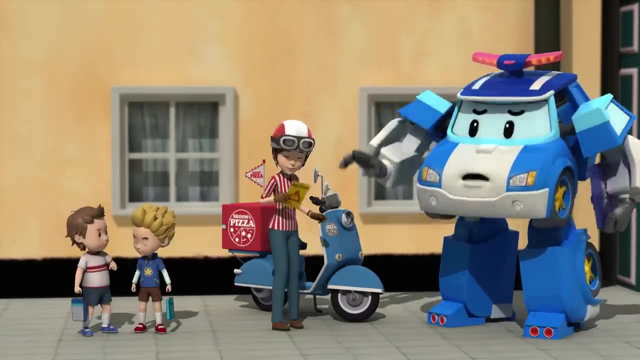 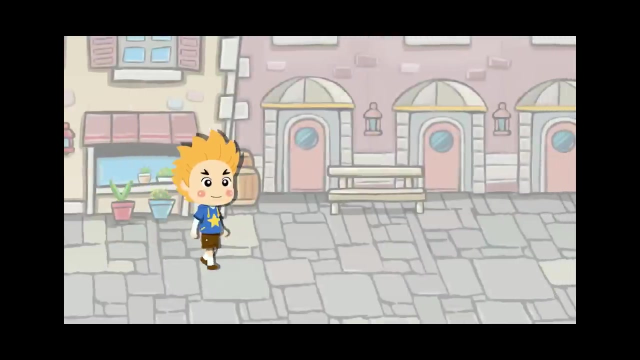 I don't know what to say. I didn't even realize I was on the sidewalk. Well, I guess we could have avoided her. That's right. No, that's not right. Huh, If you should encounter a vehicle on the sidewalk, don't attempt to maneuver around it. Instead, stand in one spot. 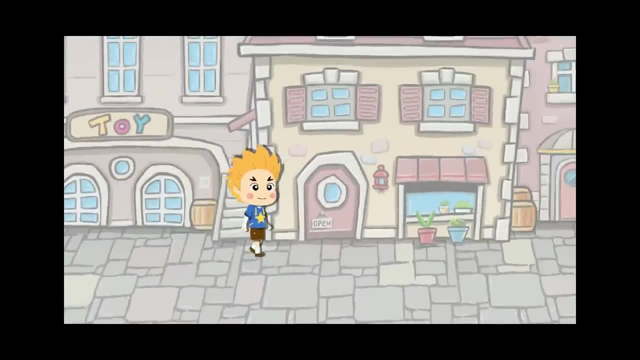 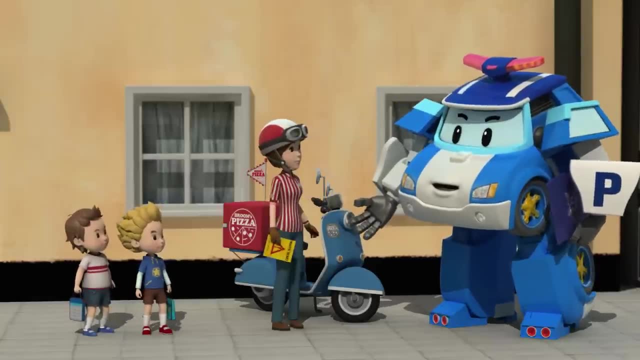 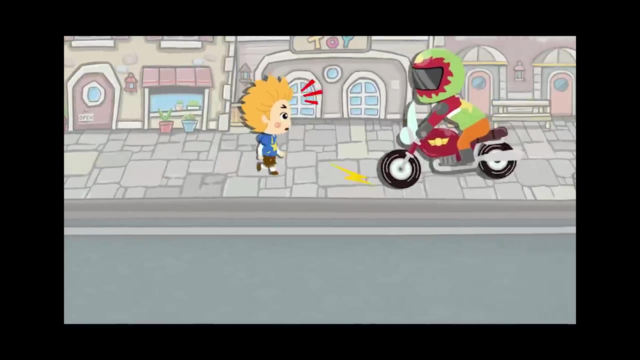 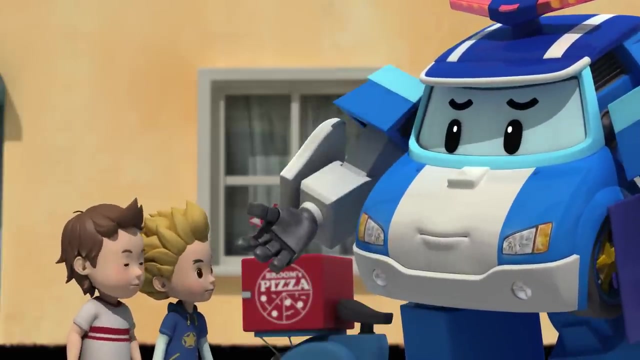 Or lean against the nearest wall. So because motorcycles can move fast, even on narrow roads, you have to be cautiously aware when you're going down a side street, getting off a bus, and even when you're walking on the sidewalk, Do you see kids? You could have an accident if you run around recklessly the way you were. 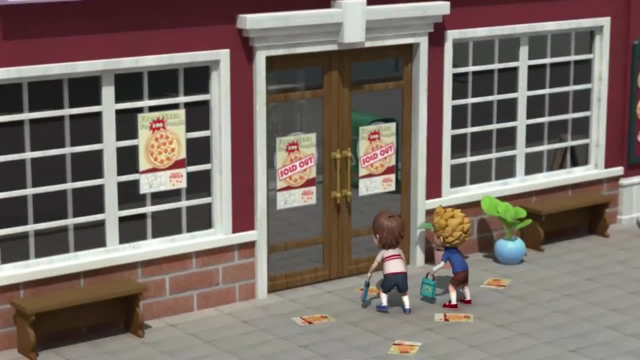 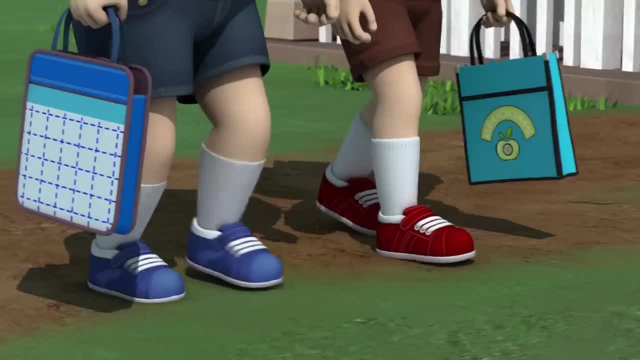 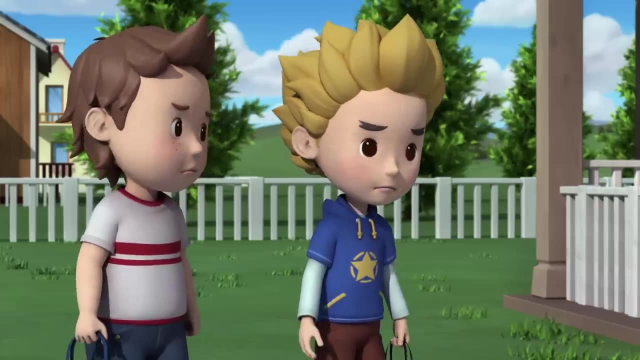 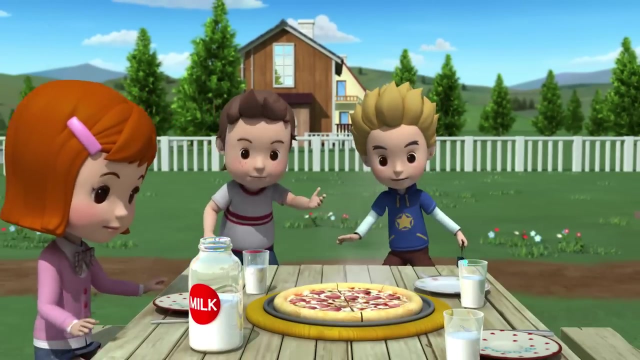 We get it, Polly. No, We missed the pizza. What took you two so long? We're real sorry, Jenny. Yeah, we're sorry. Well, hurry up Your pizza's. getting cold What? Wow, Pizza Delicious. 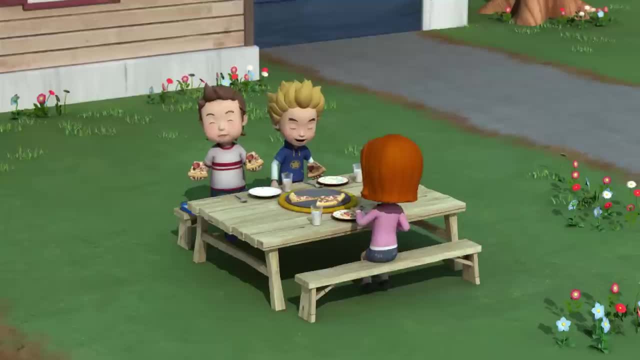 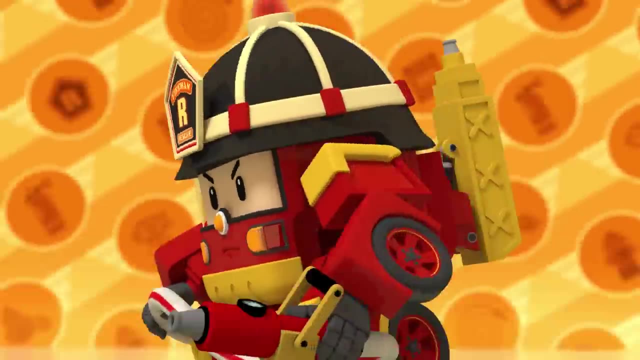 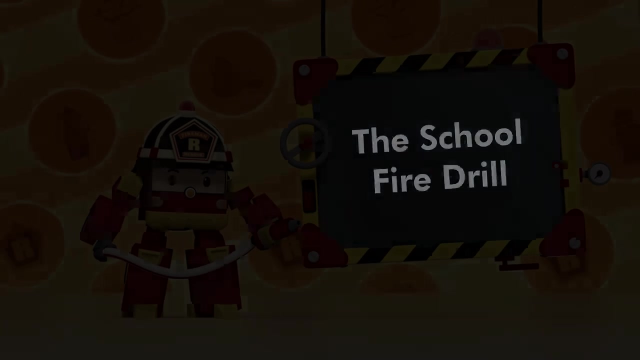 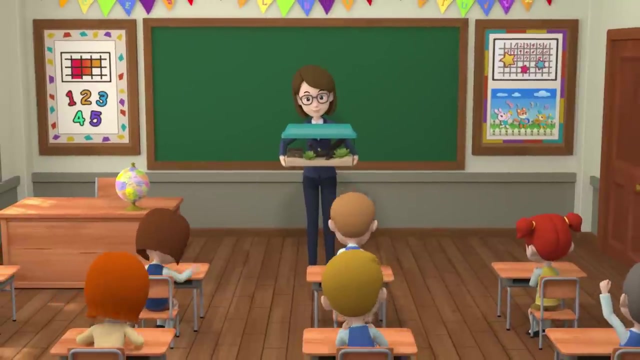 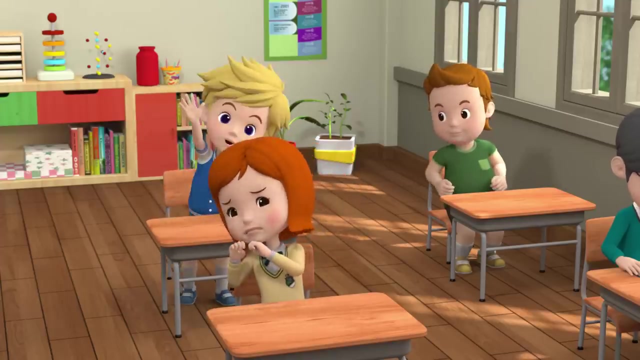 Hey, come on One slice at a time. The School Fire Drill Everyone. we have a new friend today. Whoa, Awesome, Awesome. Someone needs to be in charge of feeding him. Ugh, Pick me. I can do it, Pick me. 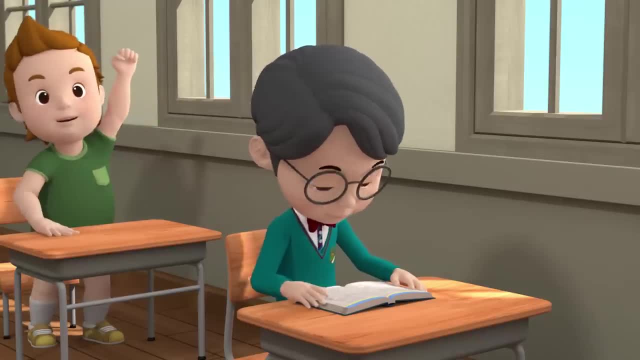 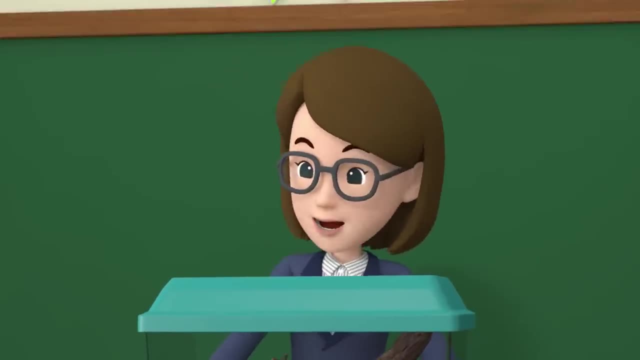 Um, Oh, Charles, How would you like to take care of him this week? Me Really, ma'am, Mm-hmm. Since I know you love animals, I'm sure you'll do a good job with our class pet. 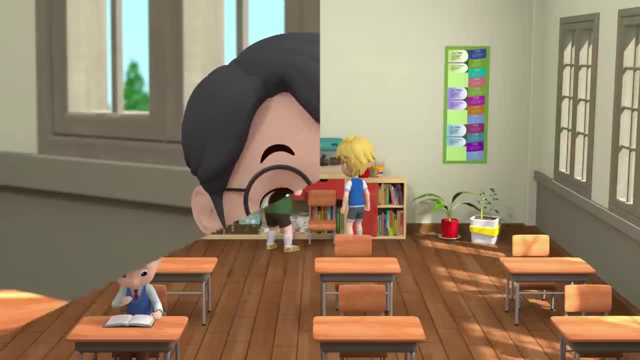 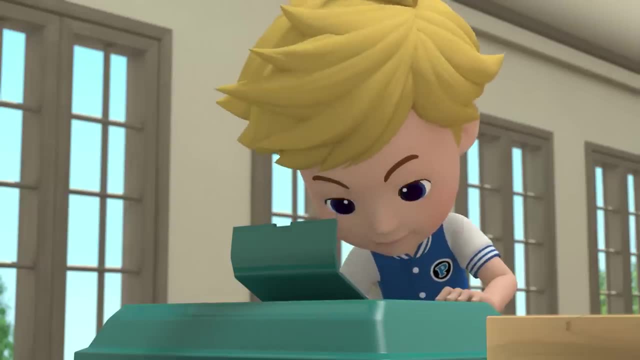 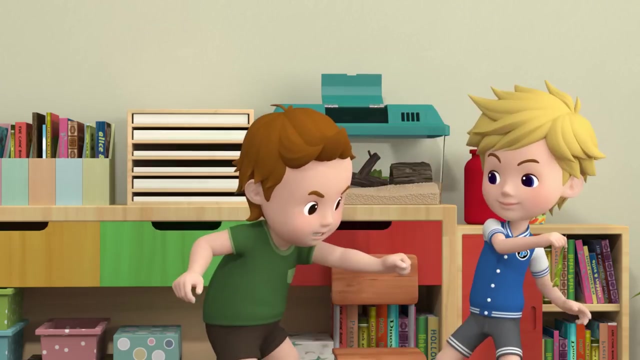 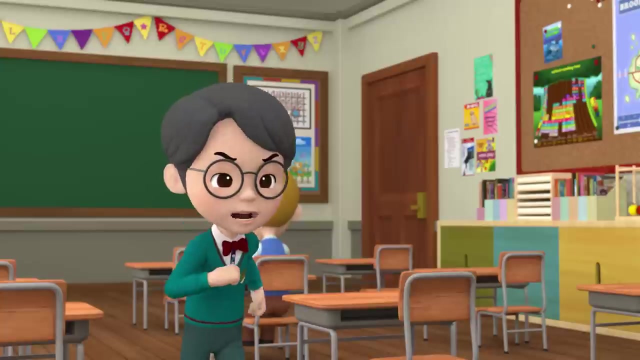 Are you up to it? You bet I am, Whoa. Why can't you stay still? I got him Whoa. Come on, let me hold him Me first. Hey, stop it. Huh, You're being cruel to him. 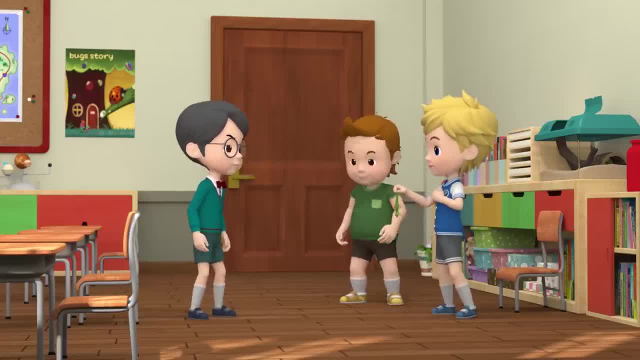 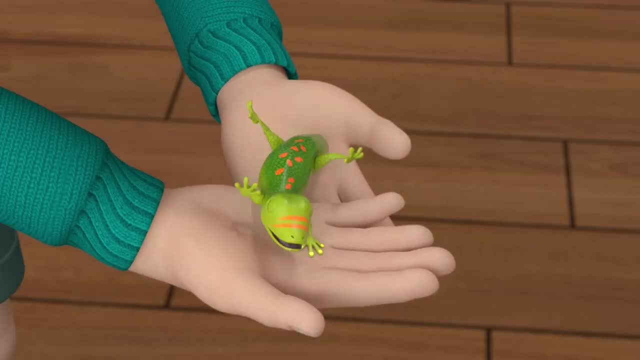 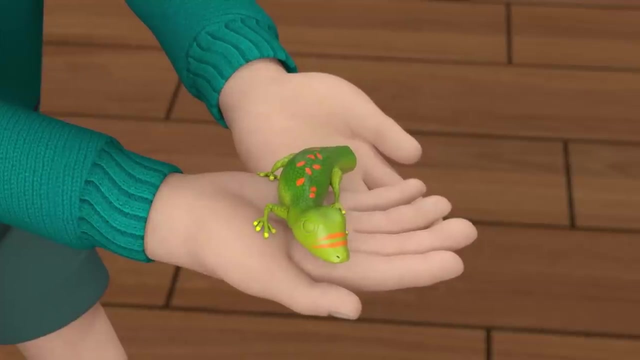 What? We're not being cruel. I just wanted to play with him, That's all. That's right. Come here and give it a try. No, I broke his tail. Some lizard and gecko species drop their tails when they feel they're being threatened. 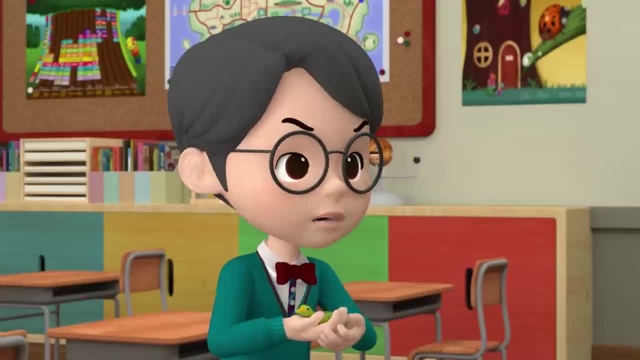 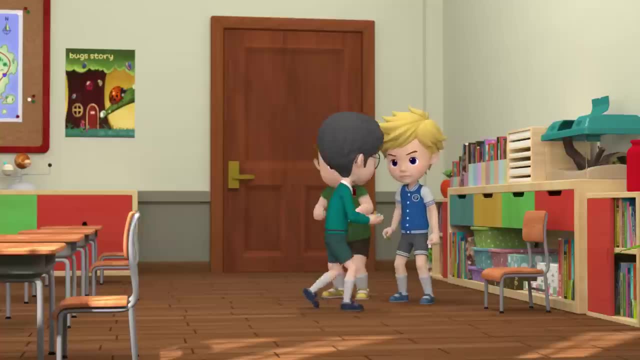 Oh, man, Ugh, That's gross. Listen, their tails hold valuable nutrition, so losing them can be really bad. I'm taking him home to keep him safe and you can't touch him anymore. Okay, I'm sorry, little guy. 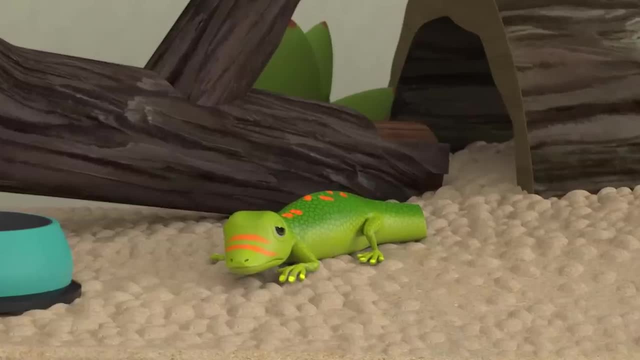 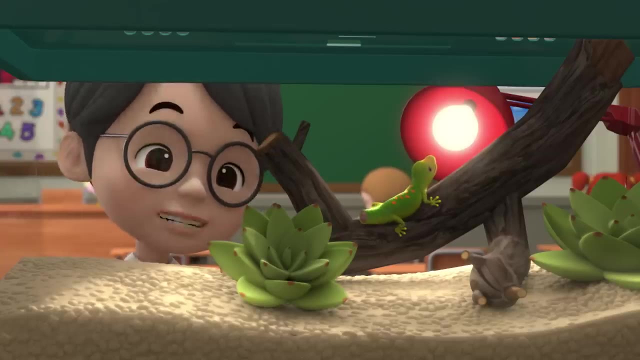 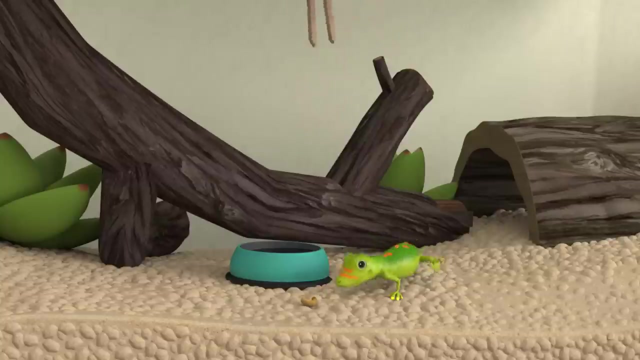 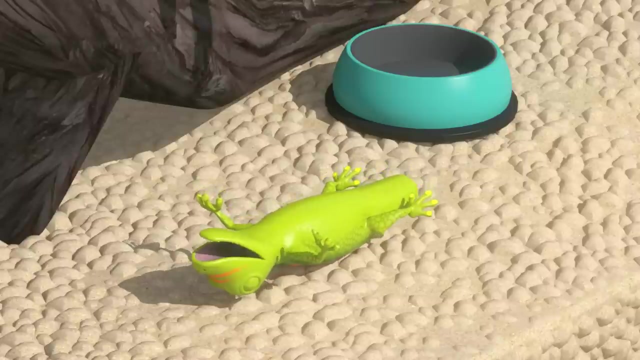 It'll grow back soon. You need a name, huh. From now on, I think I'll call you Finn. Haha, Is that better? Finn, Eat up, okay. Ah, Hahaha, Hahaha, Hahaha, Hahaha. 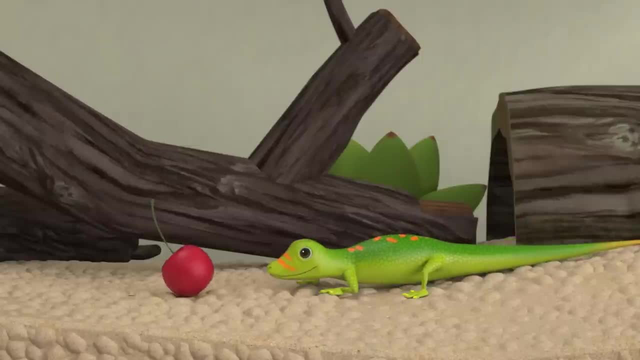 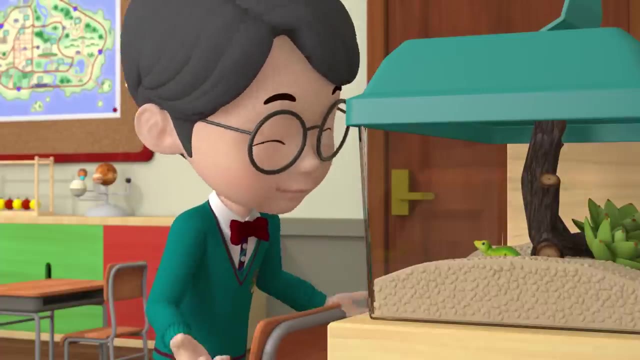 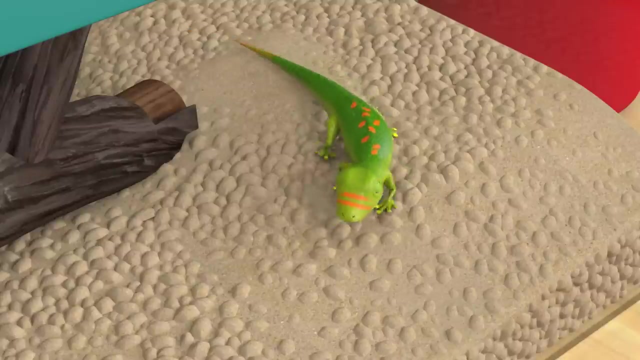 We should play dodgeball. Huh, Yeah, Hahaha. That good, I see your tail grew back. That's great. Oh, your water's empty. I'll get you some more… Hahaha, Huh, What's this? 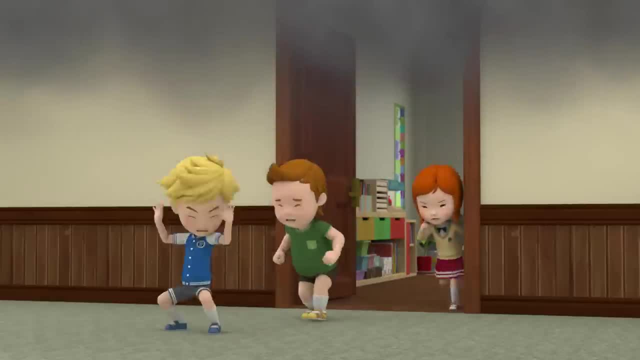 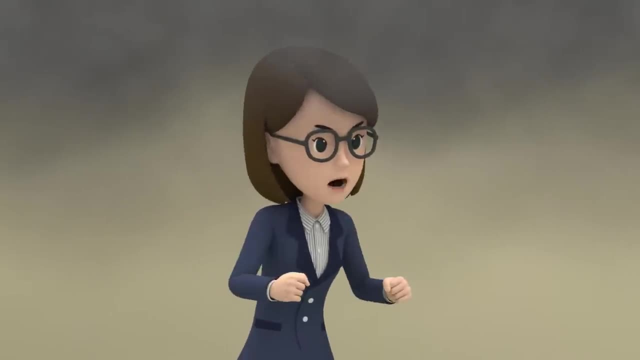 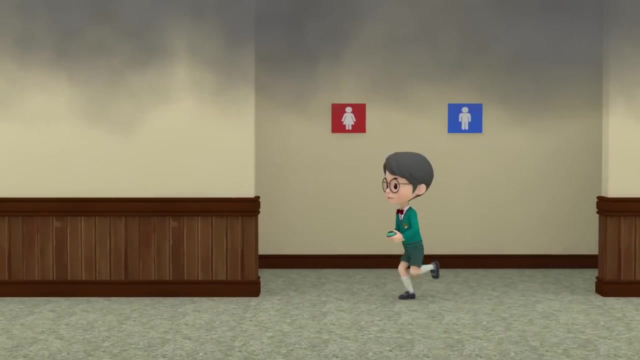 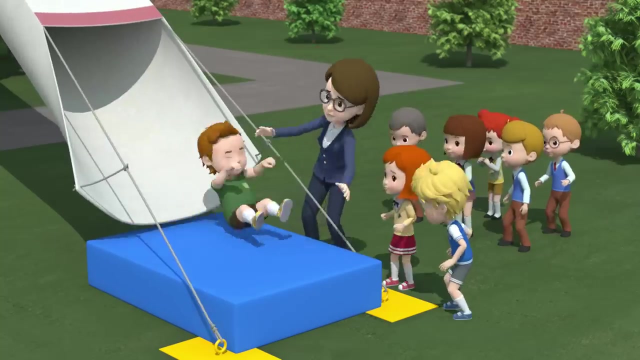 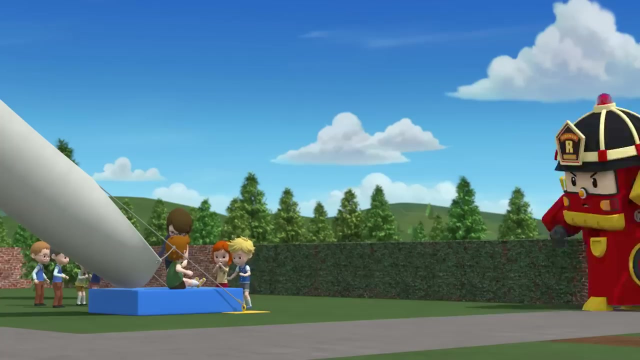 Fire, Fire. I didn't do it this time. It wasn't us, Everyone this way. What's happening? There's a fire downstairs. Single file line and follow me Right, But Finn, Everyone, alright? Yes, I think we've got all the students outside. 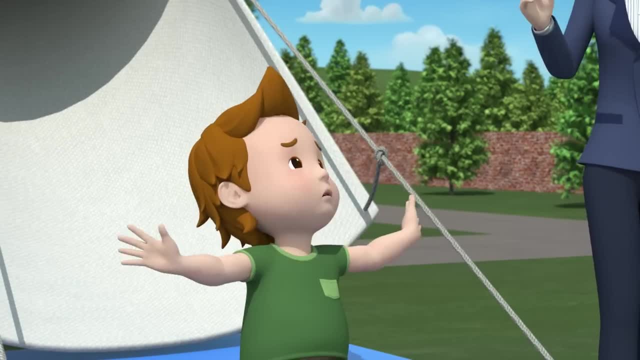 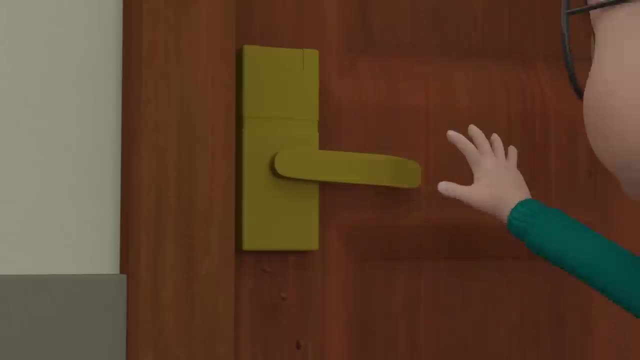 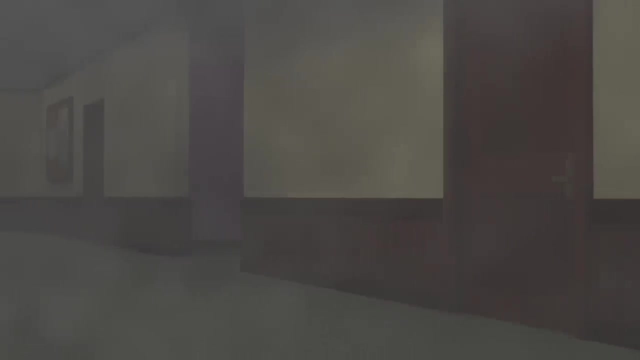 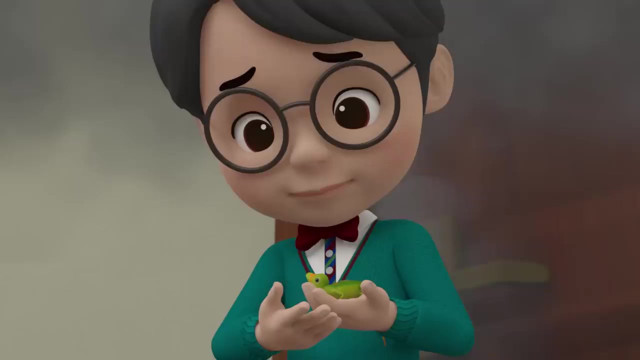 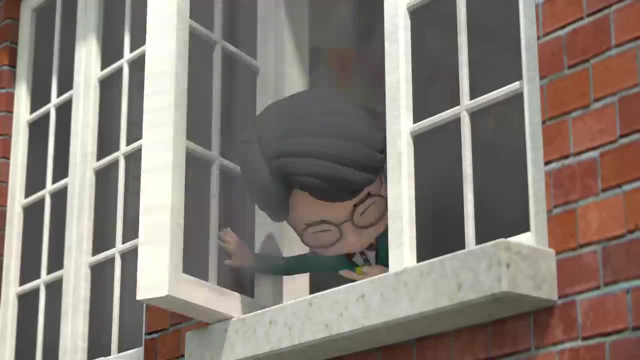 Wait, hang on, Charles isn't here. What, Charles? Hey, Finn, Now we can go. But we can't go that way. This is bad, huh? Don't worry, we'll make it out of here Over here look. 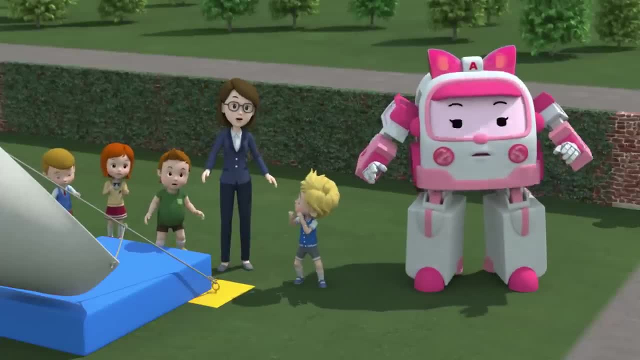 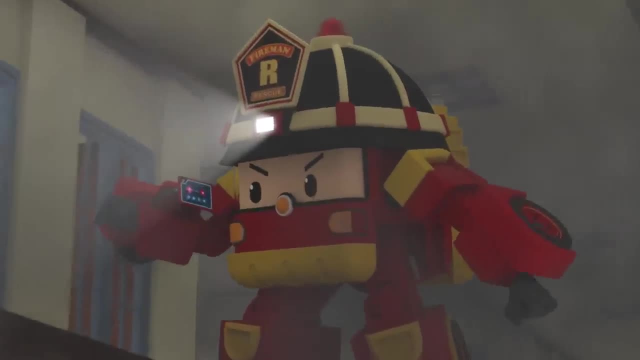 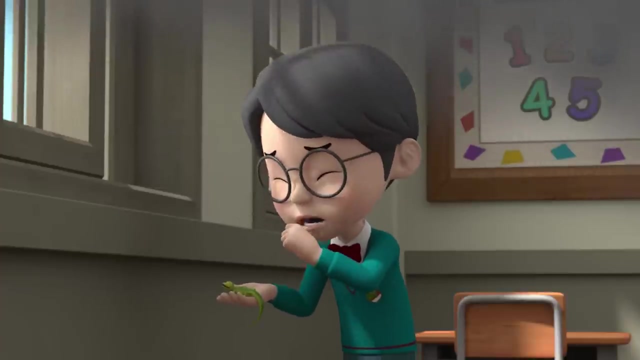 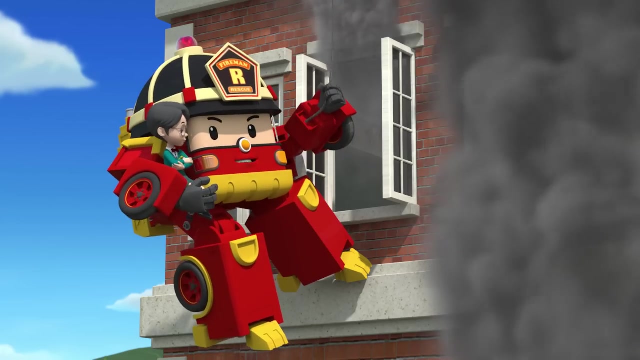 I can't get out. It's Charles. He's in the classroom. Charles, Charles, Charles, Roy, he's in their classroom on the second floor. Great, got it. Help me someone. I'm here, Roy. Okay, you ready. 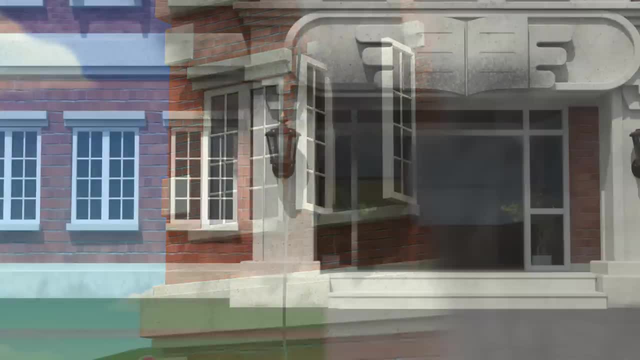 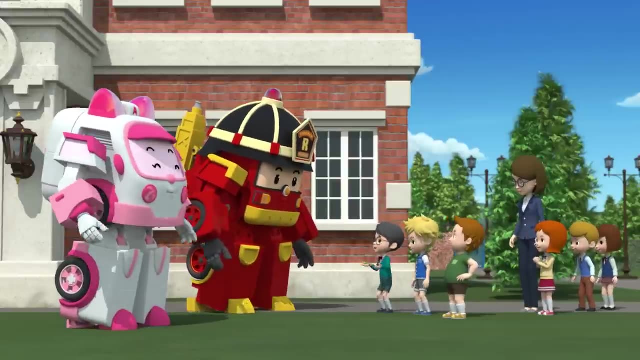 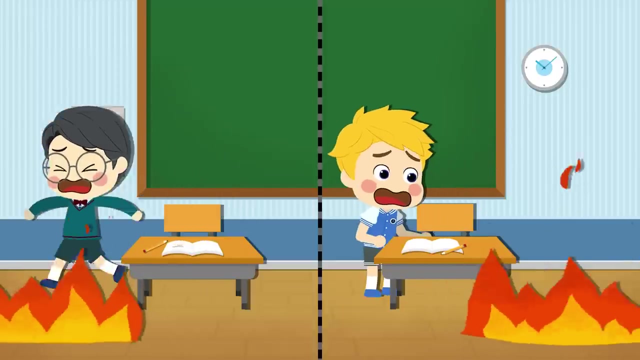 Yes, Here we go. The fire's all put out now. Thank goodness no one was hurt, Roy, thanks for saving me today, Charles. what you did was incredibly dangerous. When a fire breaks out, you must leave all your belongings and get out as fast as possible. 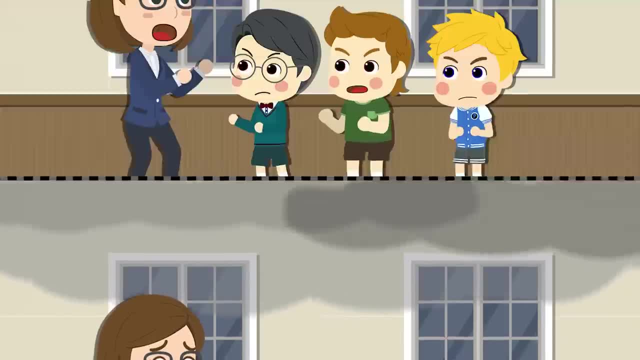 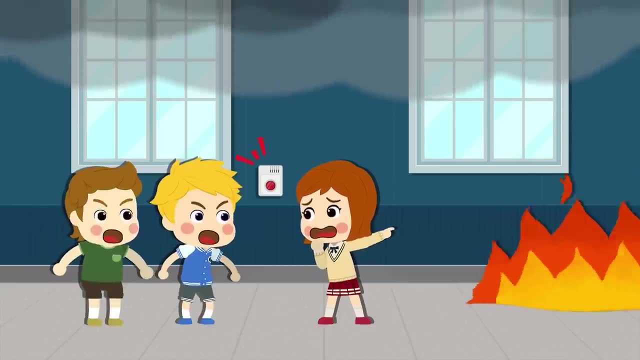 no matter how important it might be, Don't run off by yourself. Listen to your teacher and follow their instructions till you get to a safe place. Hit the fire alarm if you're the first one to see it. Cover your nose and mouth from smoke, duck down and leave quickly. 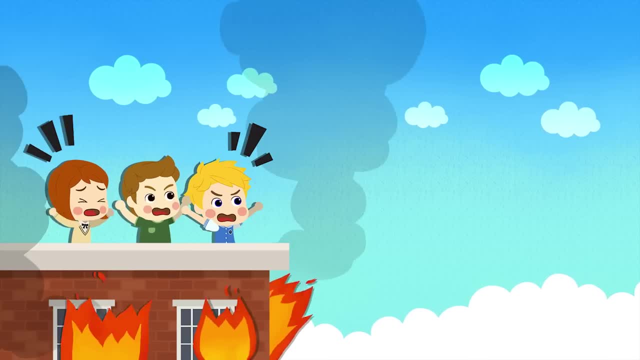 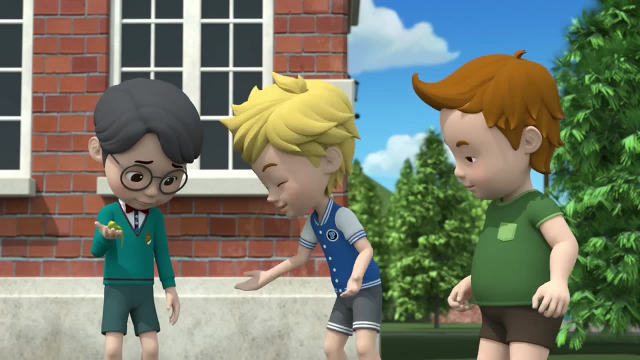 If the fire gets so bad you can't escape, run to the roof and yell for help. Got it, Roy, I'll remember. Sorry for making you guys scared, That's all right. Since you did that, you saved our class pet's life. 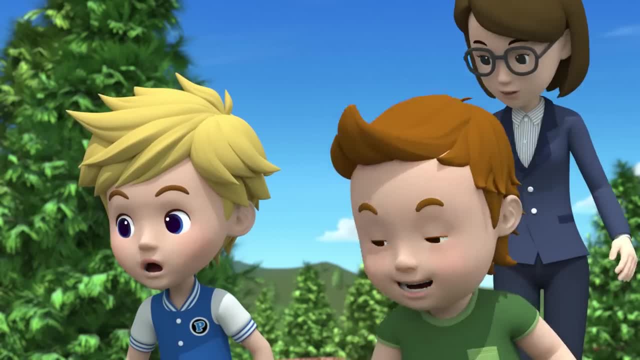 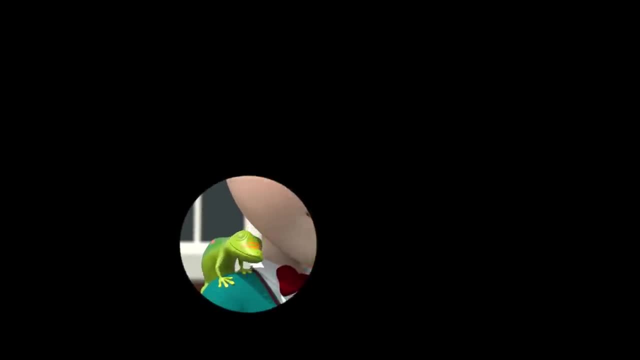 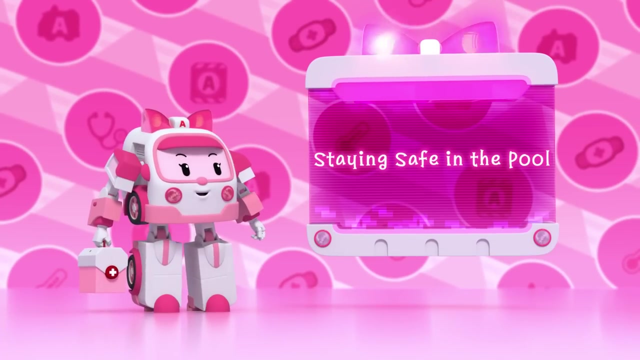 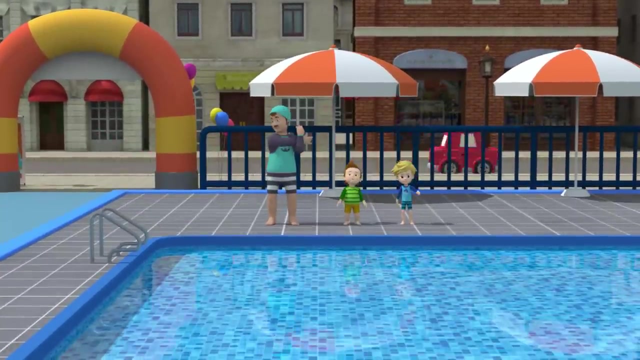 Yeah, You saved him. Oh Hey, Fin's trying to say thank you, The tickle Staying safe in the pool. One, two, three, four. One, two, three, four, Dad, are we ever going to swim? 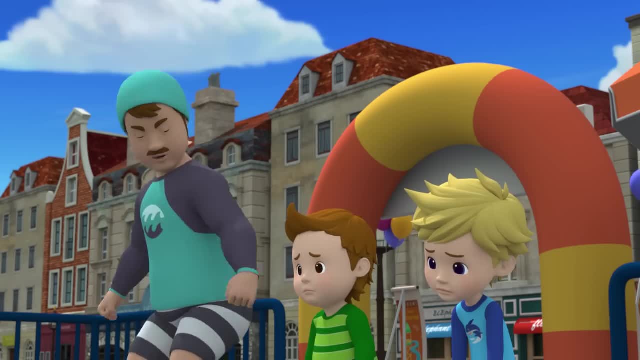 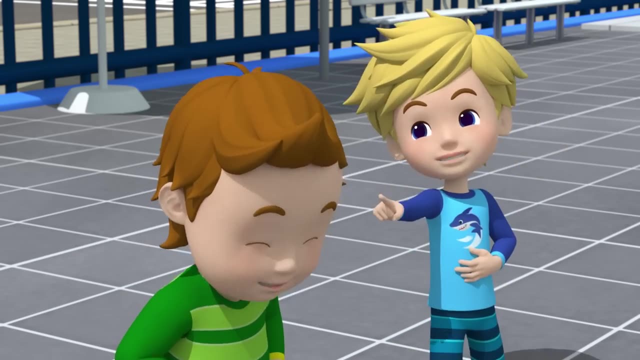 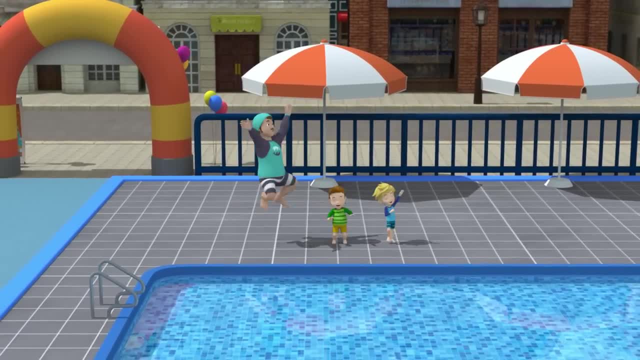 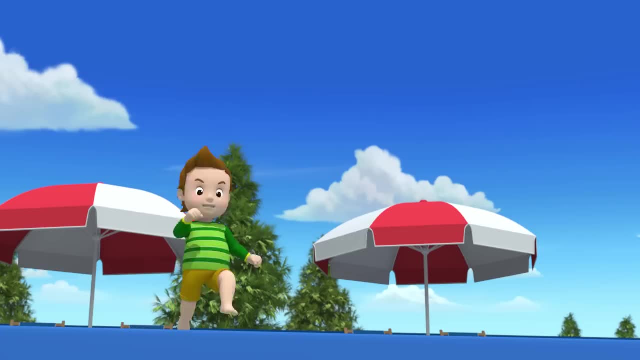 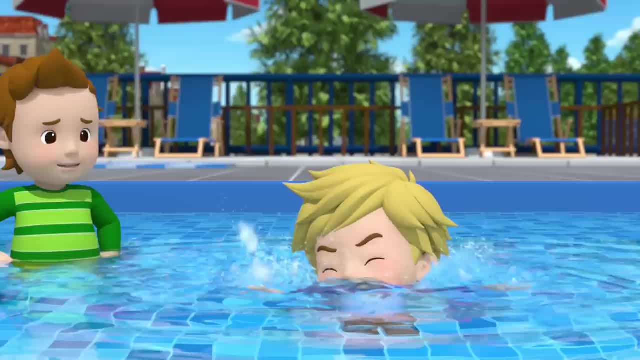 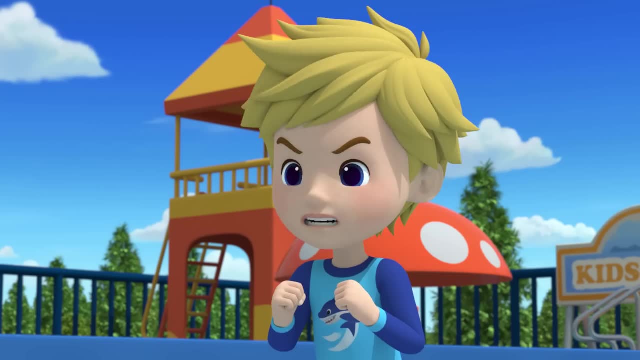 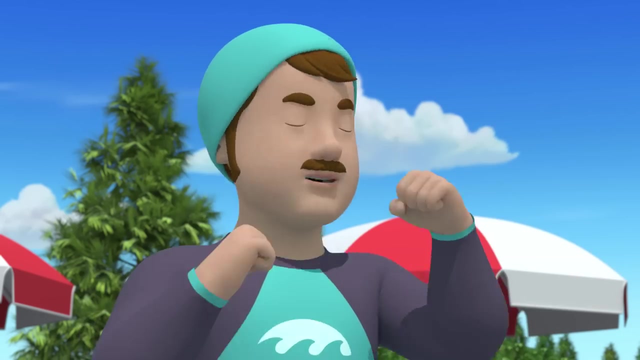 Ugh, Peter, Do you not know how to swim? What do you care, Peter? it's no problem, You can just learn. Stick with me, kid, and you'll be swimming in no time You think so. First breathe in. 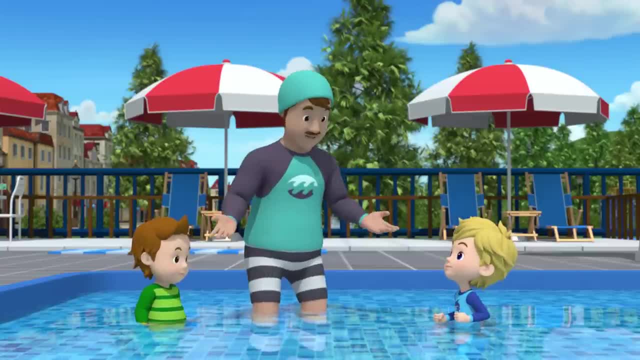 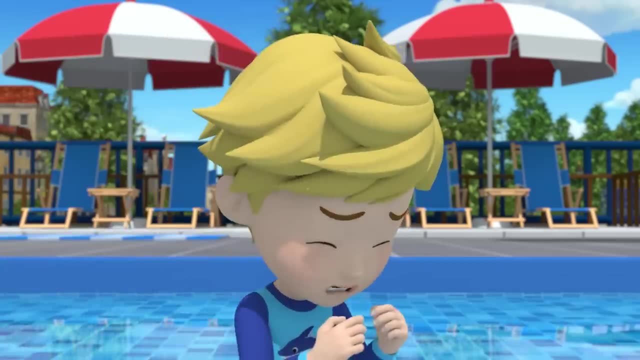 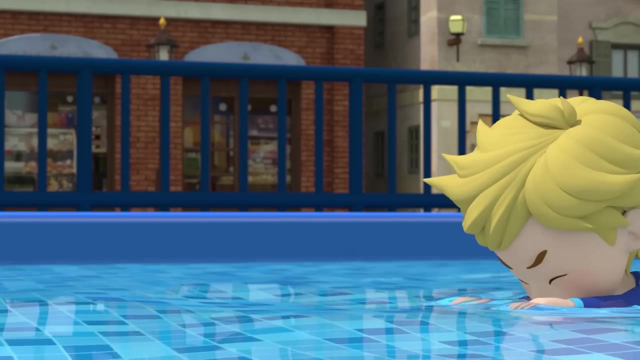 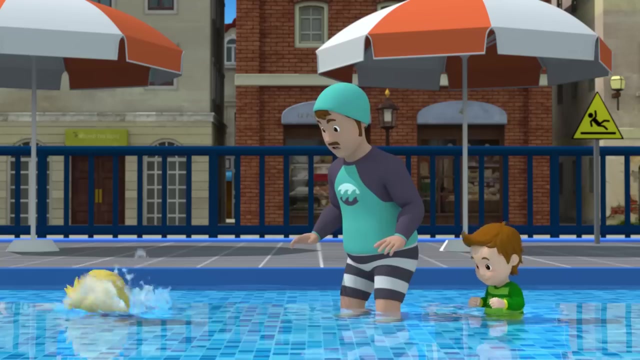 Then you want to hold it and let it out nice and deep. You try. Come on, Johnny, That's the way. Keep those legs straight. Whoa, You're swimming on your own. Don't let me do it on my own. 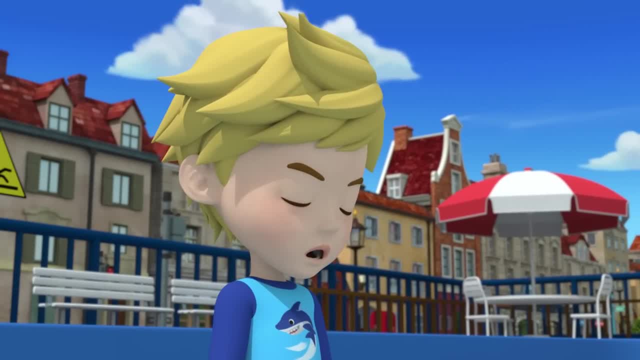 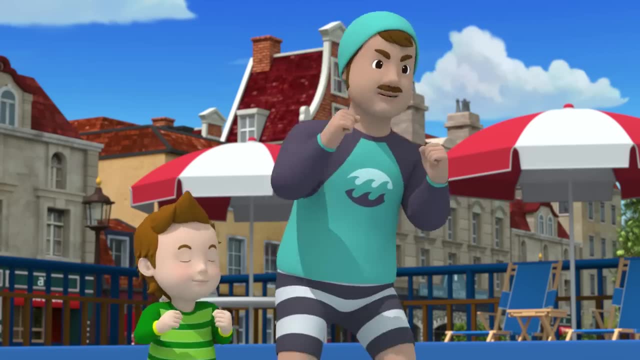 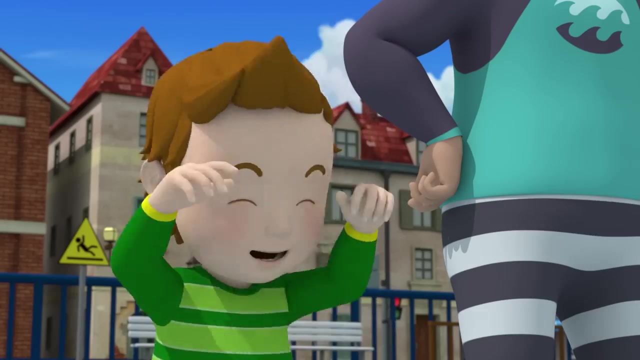 Peter, come on, You got this, That's it. Just keep kicking. You're almost there. All right, I did it. I was really swimming. You did real well, Peter. Johnny, let's go over to the other side. 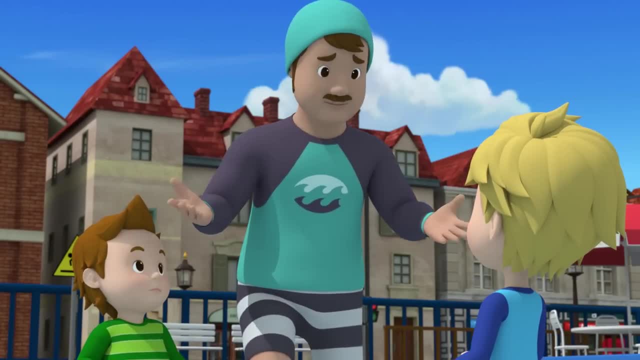 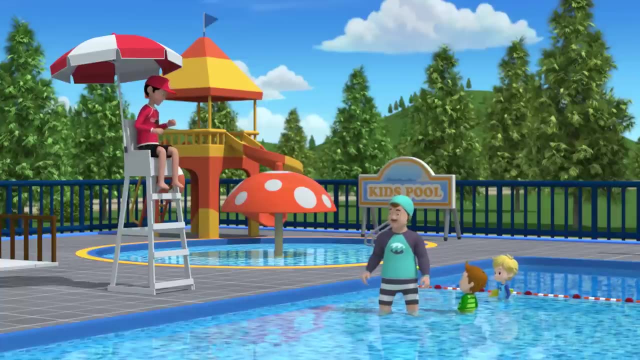 All right, Hold on. Let's not go to the deep end just yet. Hey, as long as I have this, I'll be good Time for my break. Everyone out of the pool now, please. Well, looks like it's time for a snack. 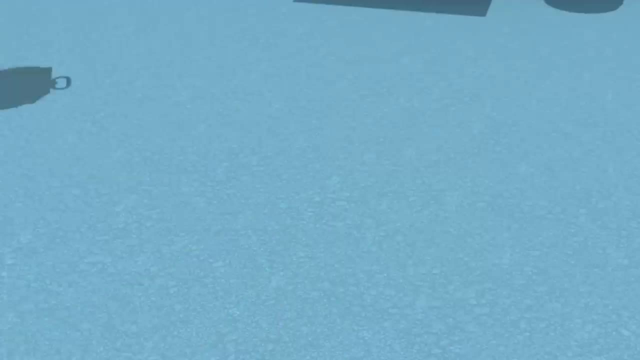 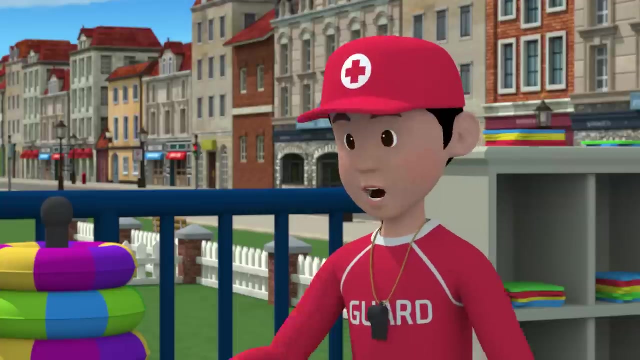 Wow, Let's go eat. All you do is toss it like this: It inflates right away and you're ready to assist a swimmer who needs help. Thanks, Amber, It's a big help. Keep them here for when you need them. 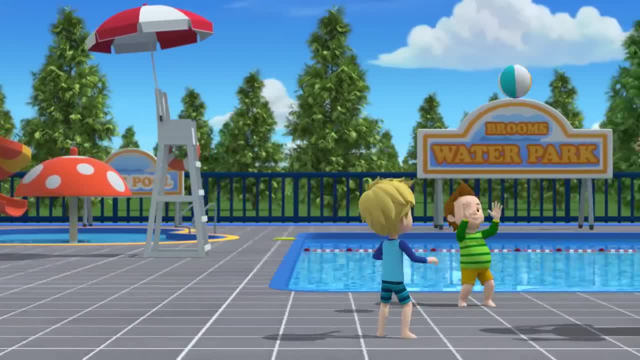 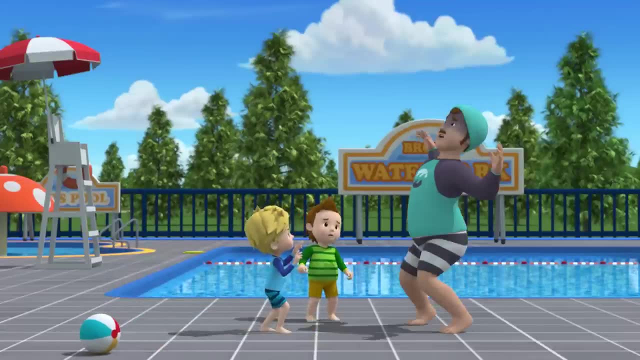 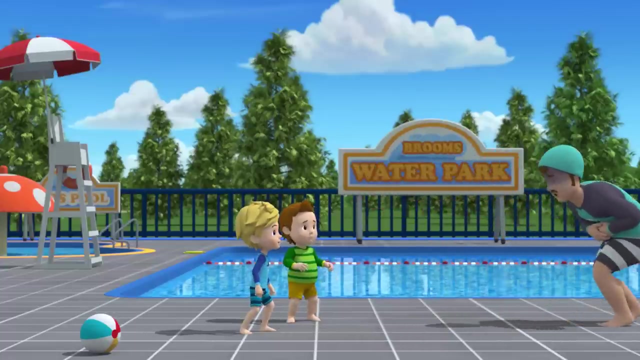 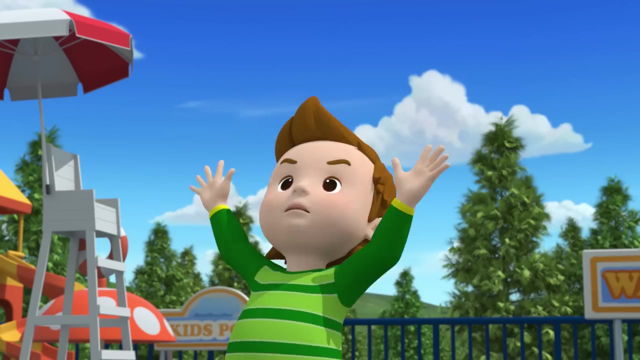 Sounds good. That's it, Got it. You're up, Great. What's wrong? Oh, no, Are you okay? No, I need to use the restroom. You guys keep playing. I can't take him anywhere. Why'd you have to hit it so hard? 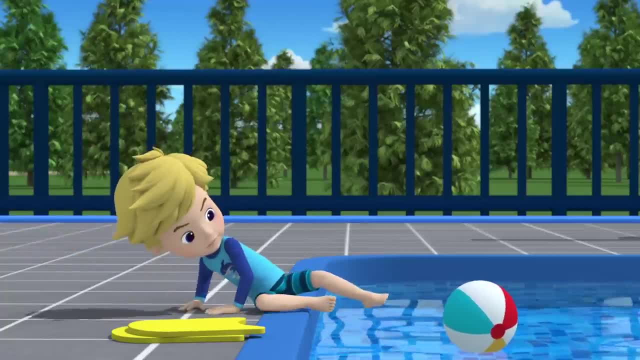 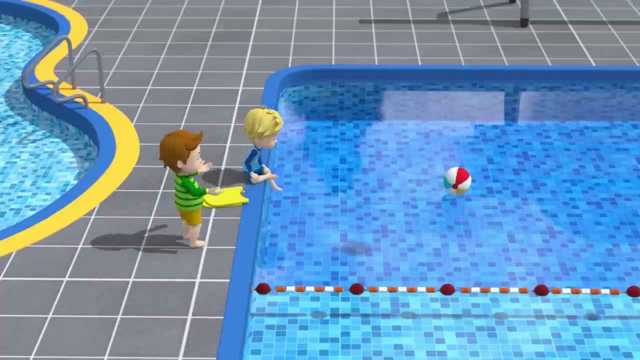 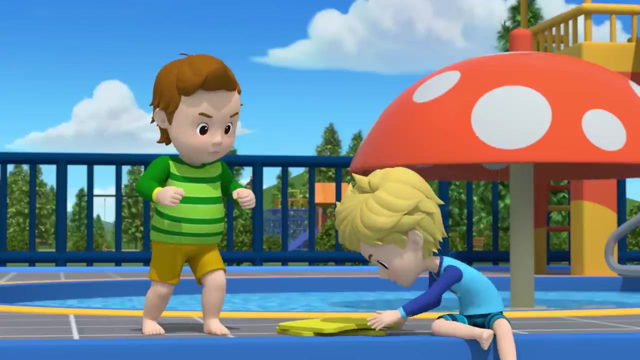 Wait, I'll get it Just a little closer. Nice work, Peter. What are we going to do now? I'll just jump in and get it What You can't. It's in the deep end. I'm just getting in for a minute. 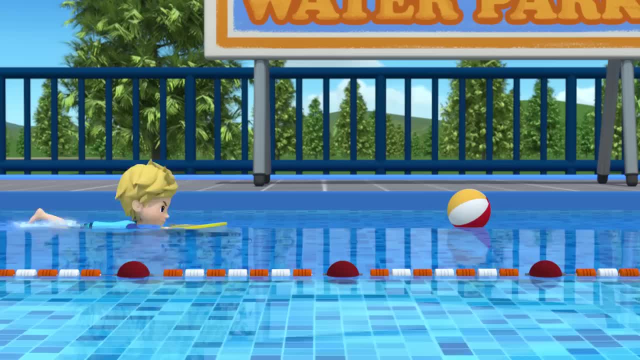 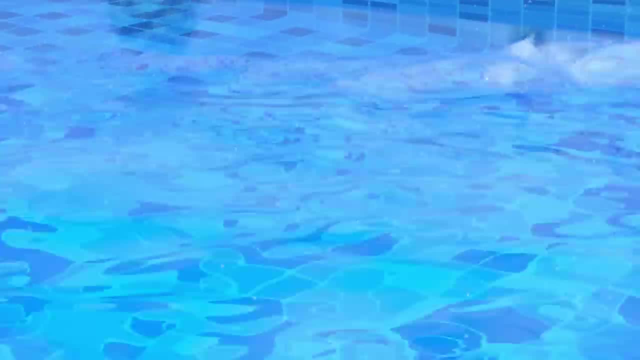 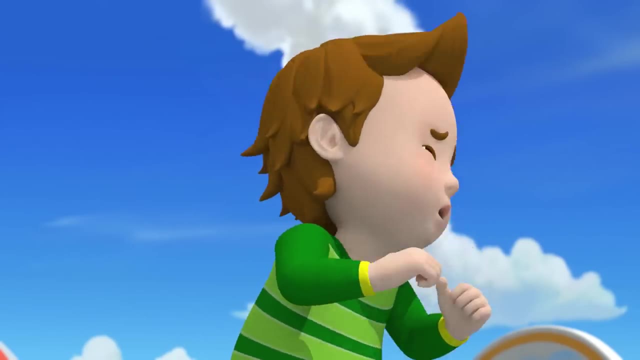 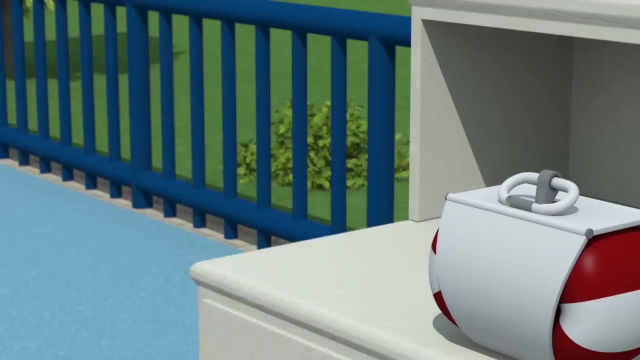 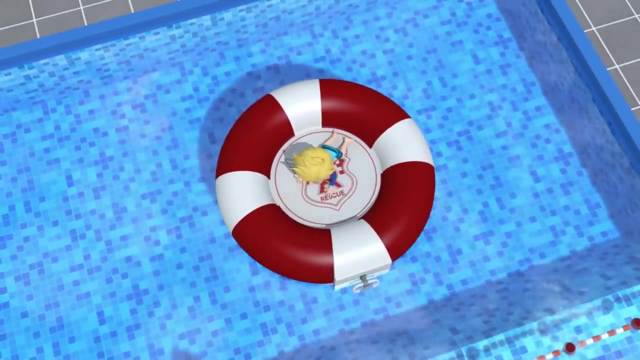 I'll be right back. Wait, Peter, I got it. Johnny, get ready to catch it. Johnny, help me. Peter, someone help My friend's in the water Over here. Please help Peter, I'm alive. 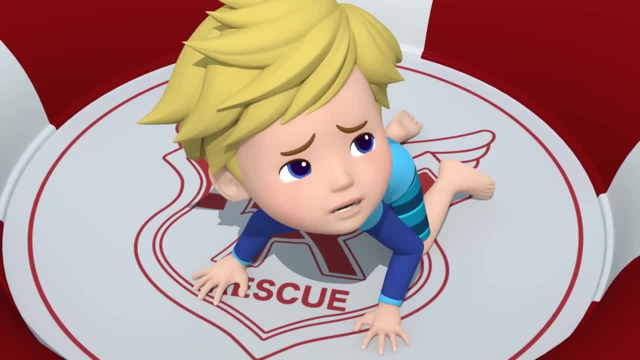 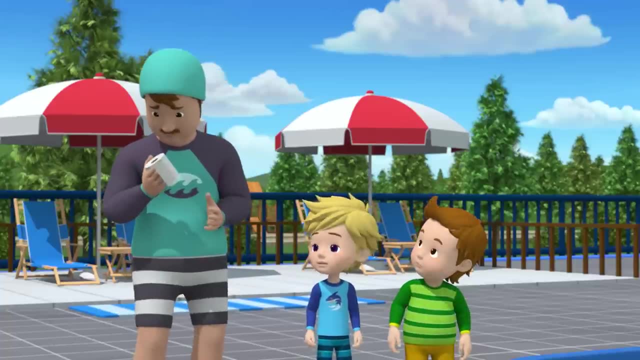 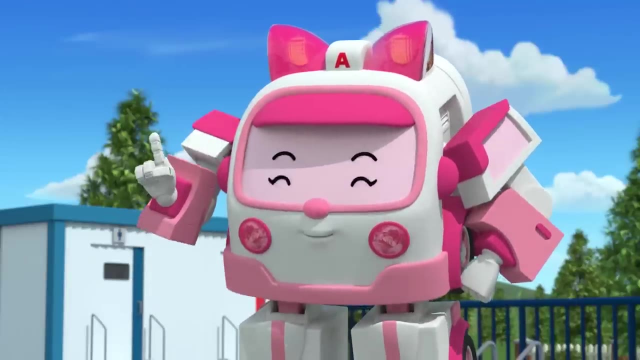 Peter, are you all right? Yes, I'm much better now, Peter, you're so lucky. you know I'm sorry, Amber, I never should have left them by themselves. Peter, Johnny, I'd like to go over some pool safety rules with you. 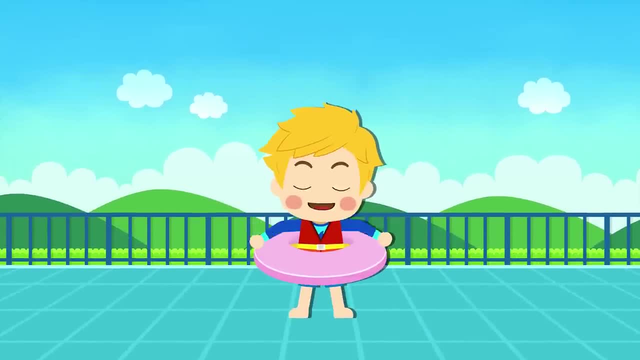 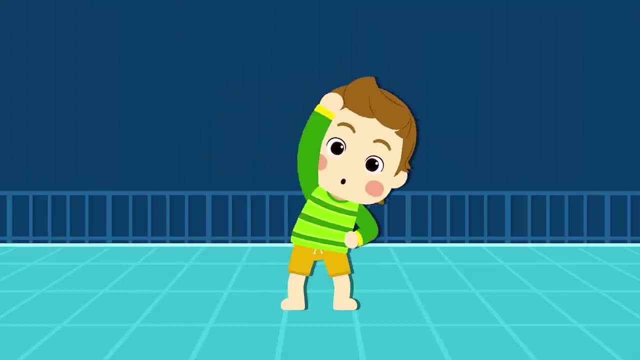 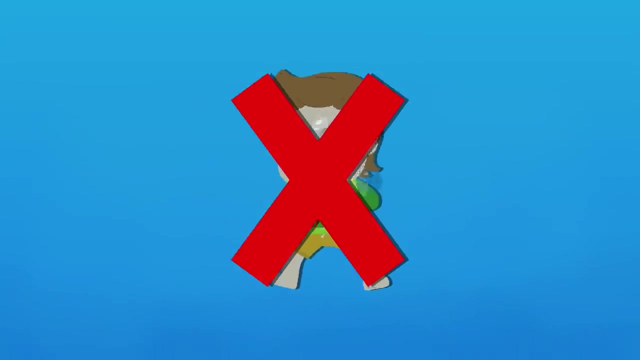 When playing in the water it's a good idea to use safety gear such as a vest or inner tube. Never swim in deep water by yourself. Try to warm up a bit before swimming to avoid cramps. If you jump into cold water too quickly it can cause heart problems. 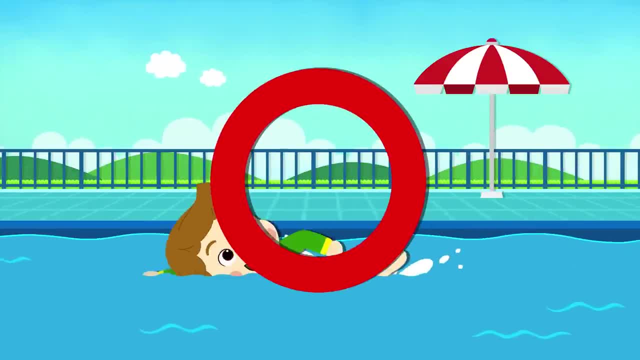 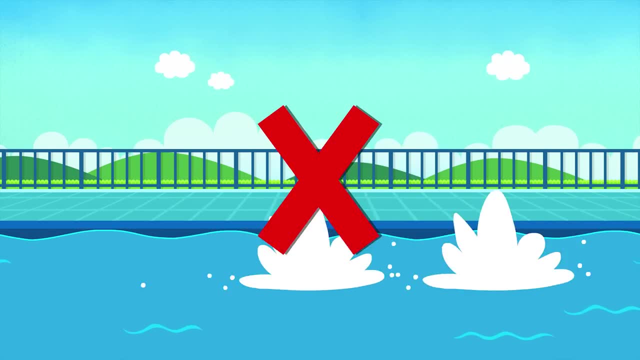 Take your time getting used to the water and go in feet first. Never run on the pool deck, as it's often wet and slippery. Before diving, be sure that the coast is clear. Don't jump back in immediately after eating. Give yourself time to digest. 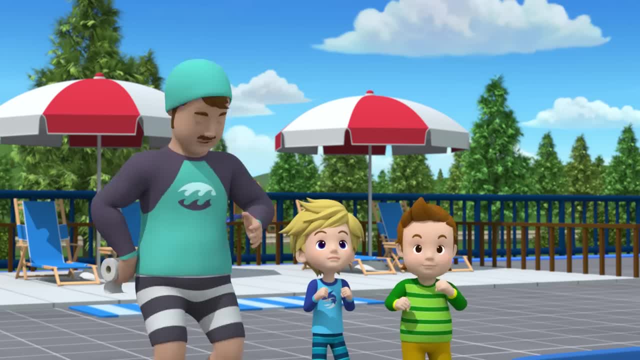 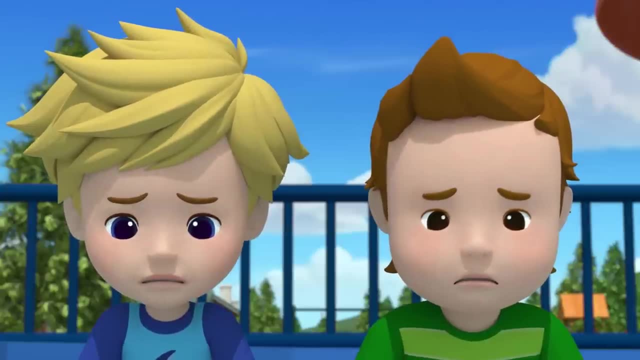 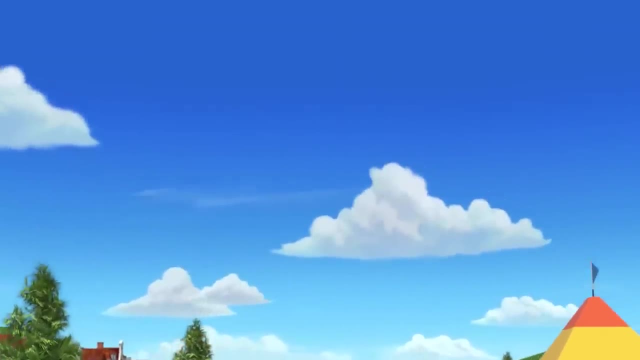 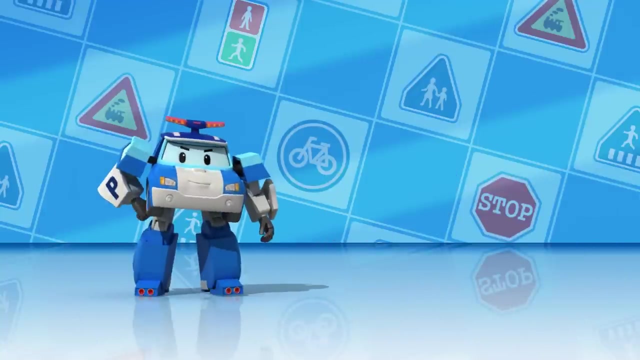 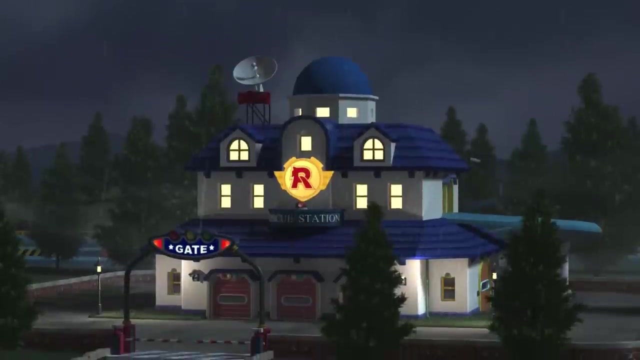 Think you can do that. Sure, Amber, And from now on I won't take my eyes off you. Right, So much safer, But we're not babies, Come on. Seat belt safety. нужен сидuma Seat belt safety. 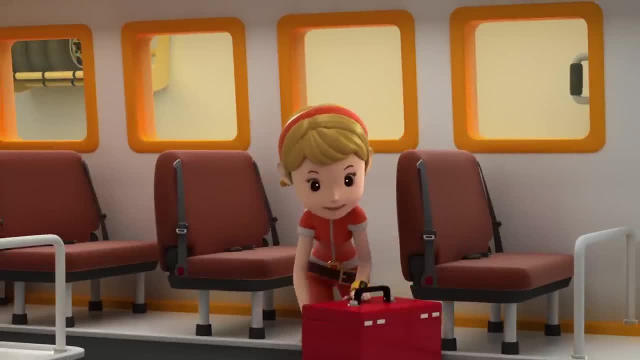 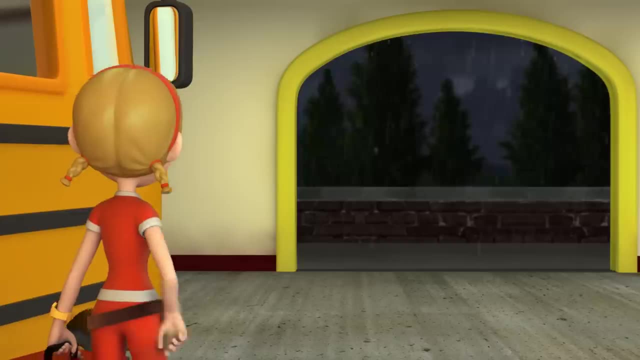 You're all set School Bee. These new seat belts will help you keep the children extra safe. Thank you so much. This will make the kids and their parents happy. You're right, I hope this rain stops so you can take the children on their field trip tomorrow. 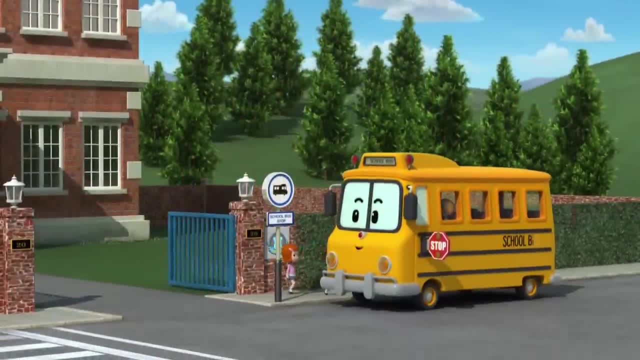 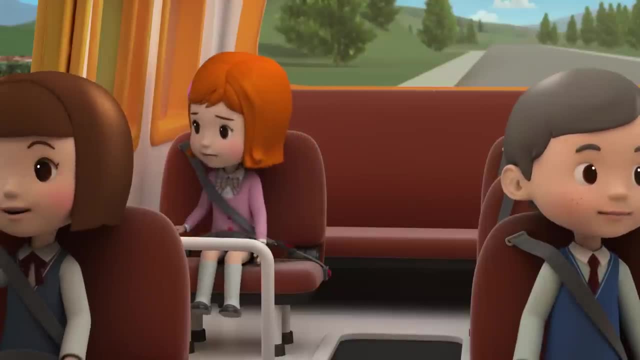 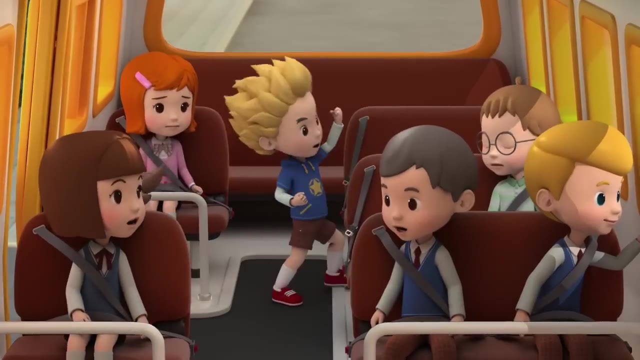 I hope so too. Oh, I'm so glad that it's a beautiful day. Hey kids, are we ready? Not yet. We're still waiting for Kevin and Doug to come out. Where are they? All? right, I get the window seat. 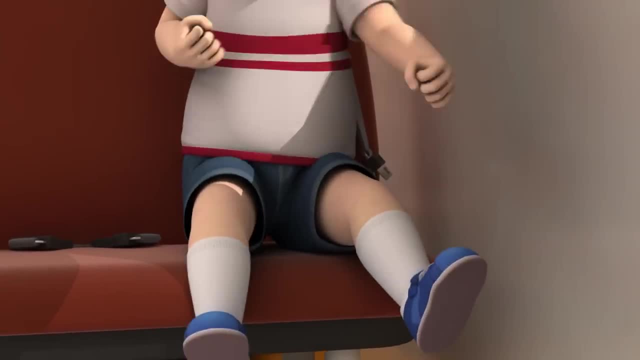 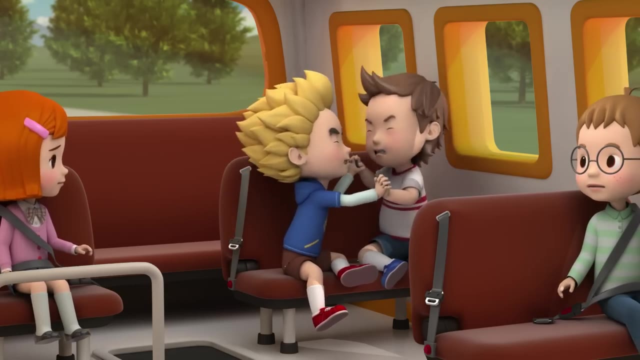 No, you don't Stop. Yes, victory is mine. That wasn't fair, Doug. Oh, no, you didn't. Yes, I did. Oh children, stop that, please. It's time for us to go, so I need you to strap yourselves in. 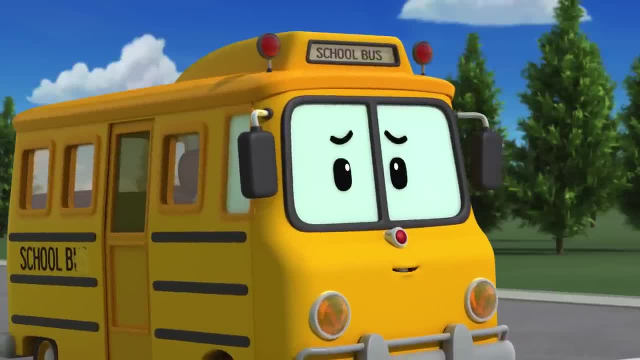 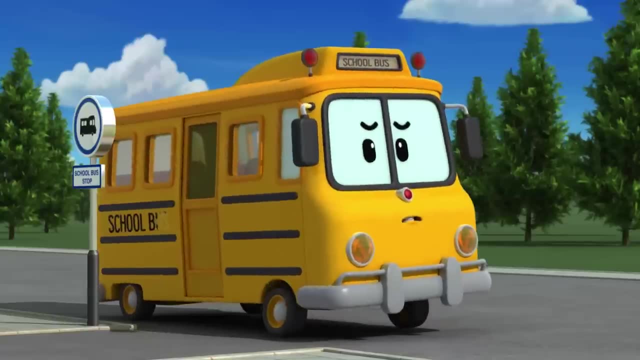 What Schoolbee got new seatbelts. They are new. They're three-point safety belts. They've been proven safer and more effective than the old ones. Seatbelts need to be worn properly if they're to keep you safe while you're in a car. 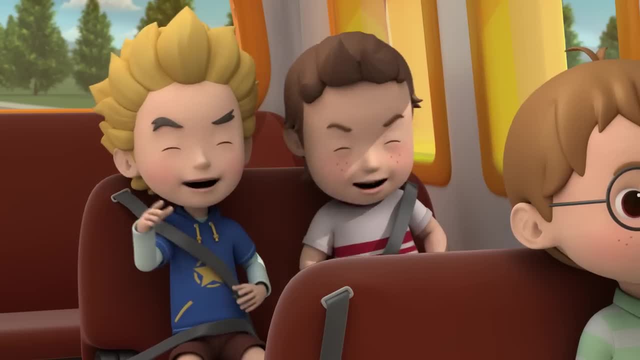 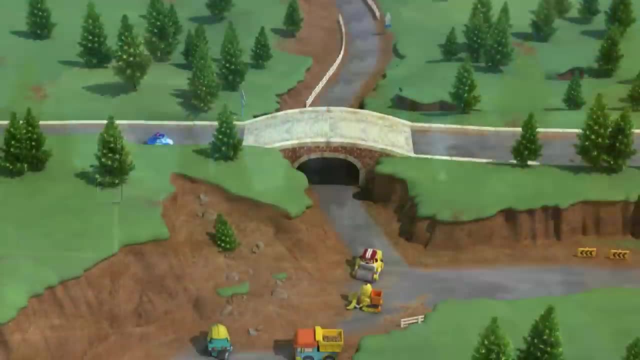 If you wear them like that you could get injured. We know that Schoolbee Phew. Well then, let's be on our way. Okay, fellas, keep up the good work. We can knock off for lunch early. 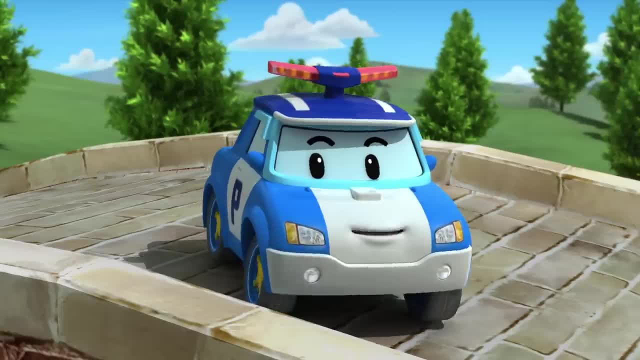 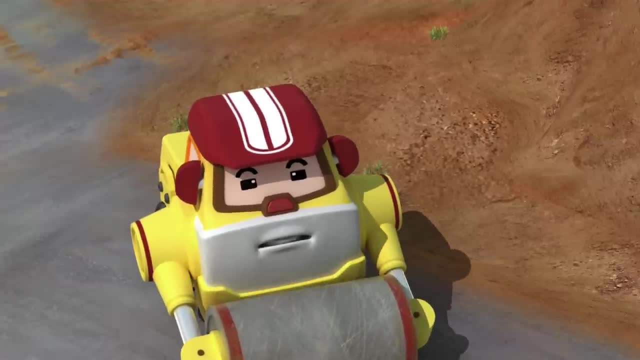 Hi there, Max. Oh hi Polly. It looks like you guys are working hard. Yes, it's because of the rain. It made a mess of the hillside. How are you Me? I'm great, I'm making sure there's no other damage. 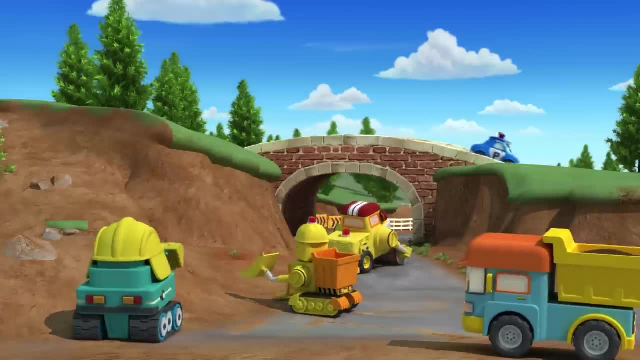 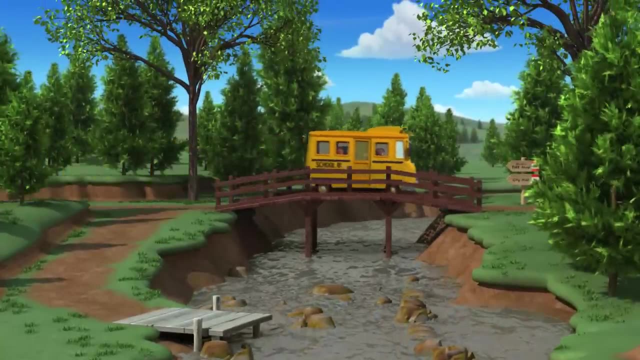 Keep up the good work, everyone. Bye, Polly. Isn't this a beautiful day. Let's go out on an adventure. Oh wow, Come on, It's my turn to sit there now. Hey, there's a rabbit- What. 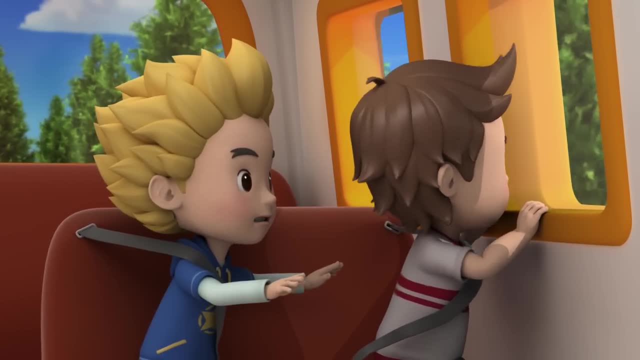 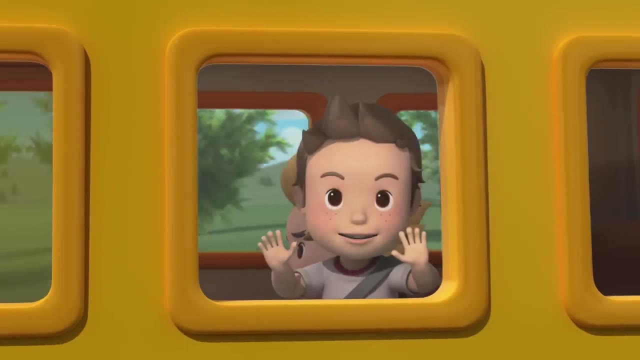 Let me see it. Oh, he's gone now What? Aw? I wanted to see him. Wow, It's a squirrel Where. Look out, Let me see, You just missed him. Aw, I can't see out the window because of this seatbelt. 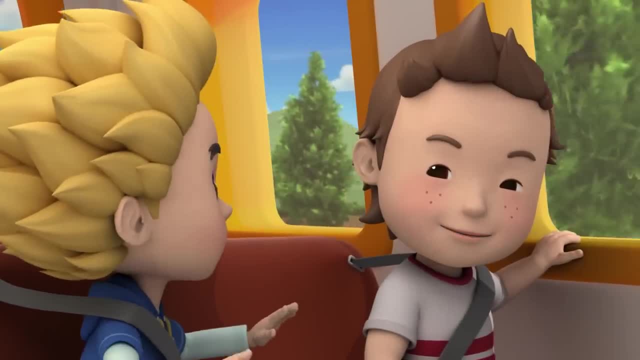 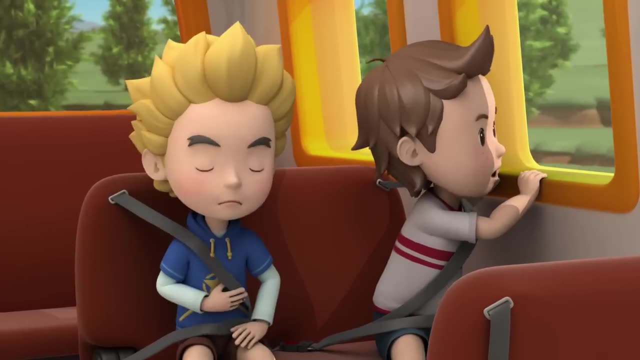 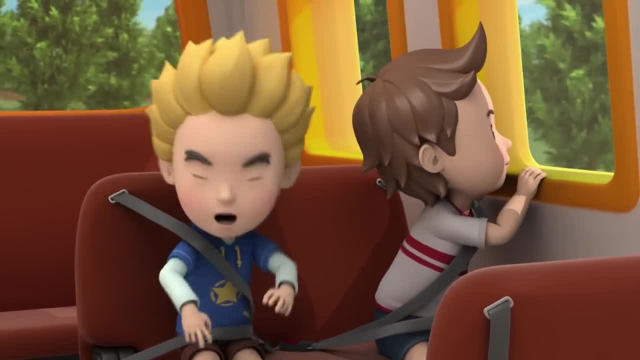 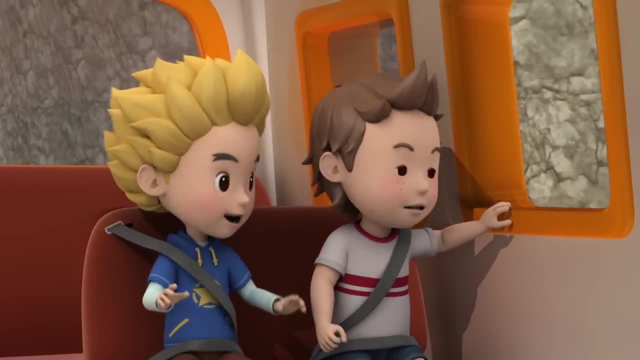 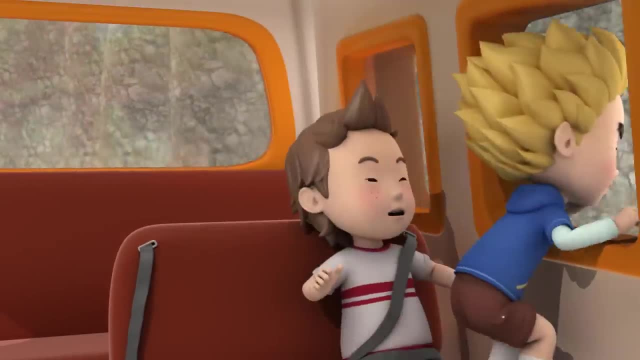 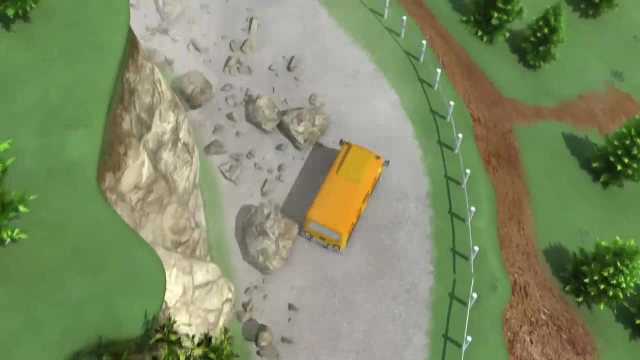 Oh, now he's gone. Aw, come on. Huh. What does that mean? Huh? Well, whatever it is, I'm not missing it. Huh, Woohoo. Oh no, Kevin, Get back in and put your seatbelt on. 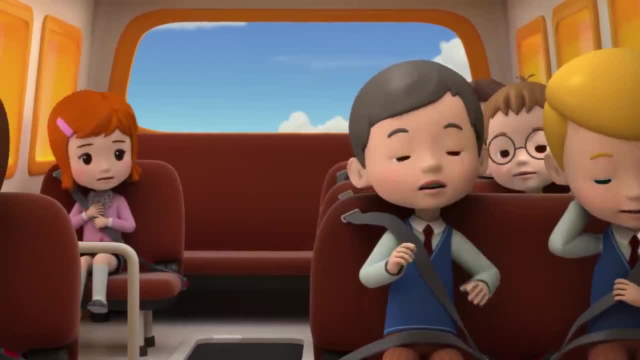 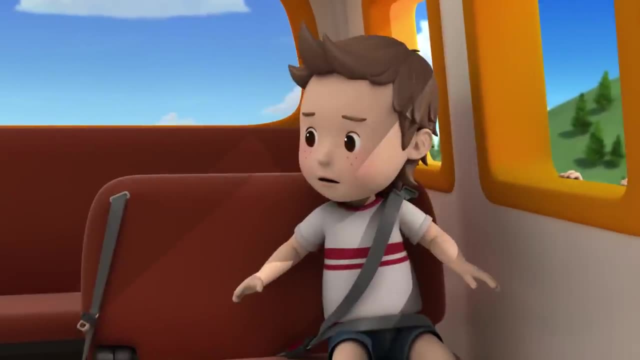 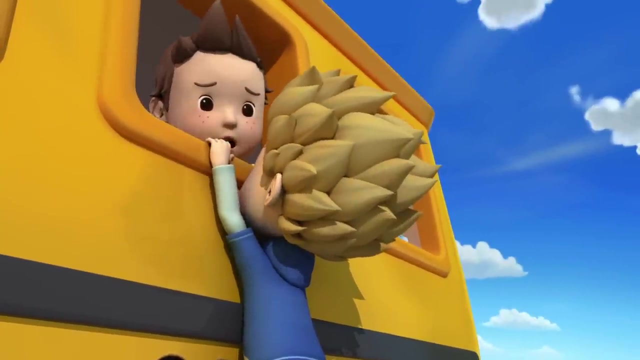 Ah Yeah, yeah, we're okay. Your new three-point safety belt saved our lives, Schoolby. Somebody help me. Where's Kevin? I'm out here. Doug Kevin, what are you doing out there? I just wanted to look out the window. 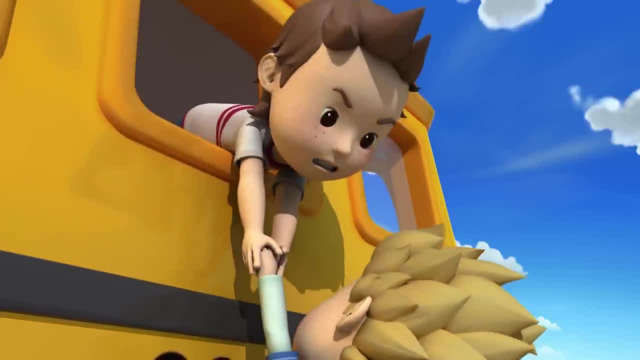 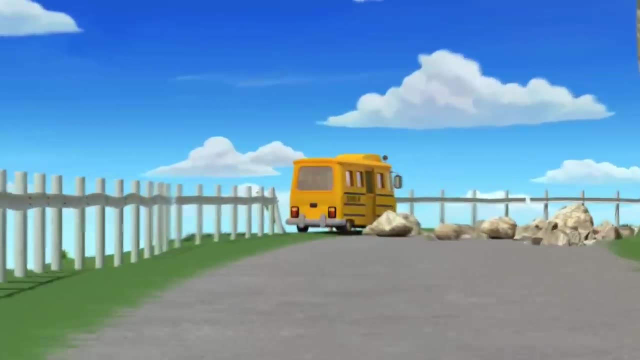 Hold on, all right, I'll help you back in. Oh no, Somebody help us. There's a child in danger here, What It looks like. Schoolby's in trouble. I got you. Don't let go. Don't let go of my hand. 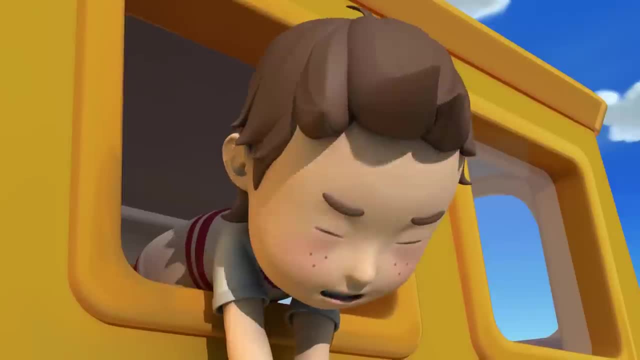 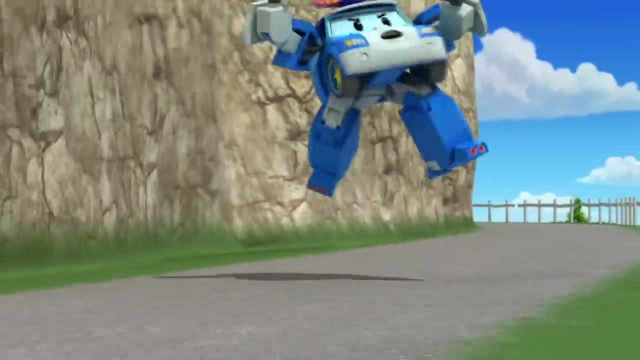 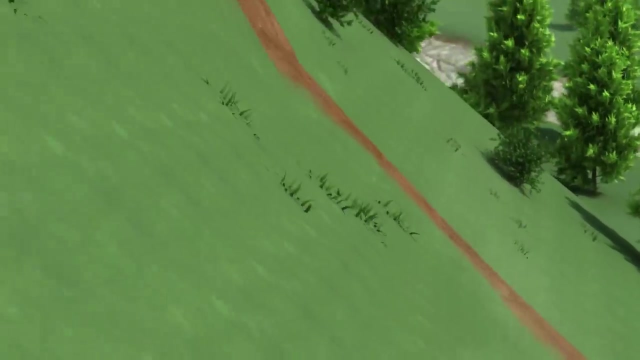 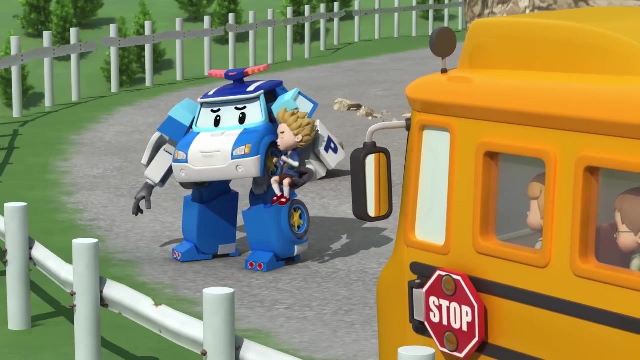 I won't. Please don't let me fall. I'm losing my grip. Hold on, Kevin, Kevin. hold on, Gotcha. Just tell me when it's over. Holy, Are you all right? Thanks to you, Hooray. 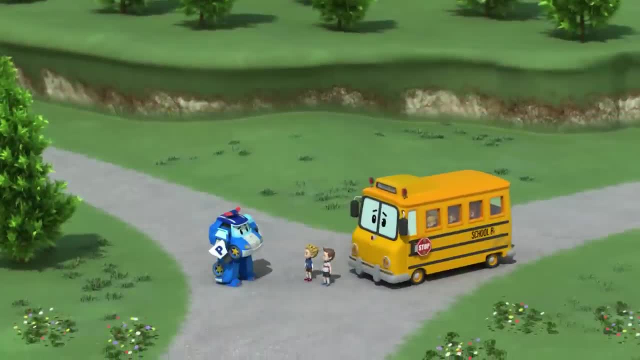 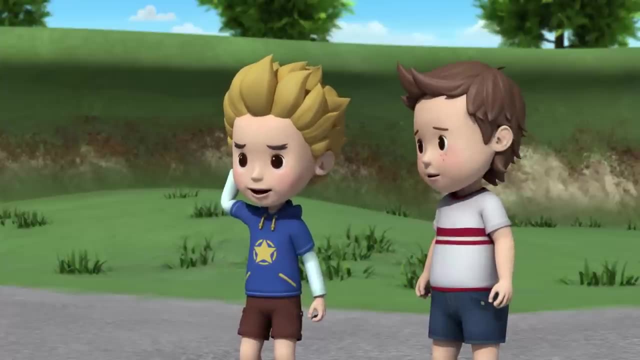 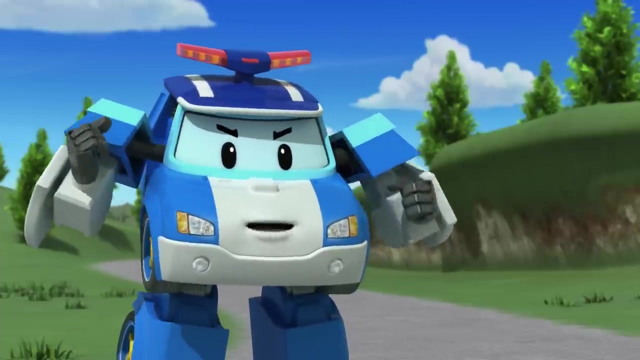 Hooray, Kevin. now do you understand why it's important to always wear your seatbelt? Well, I had it on when we started out, but then— Accidents can happen in a split second, and that's why it's important to wear your seatbelt, even on short car rides. 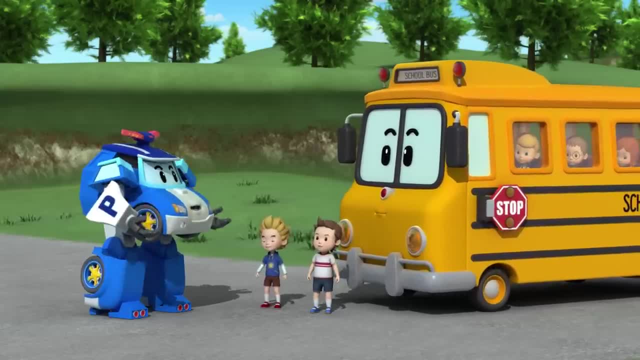 Listen up everyone. This is important. Your seatbelt can save your life In the event of a crash. your seatbelt can help you to avoid serious injury And if your car is in a serious accident, don't let it get stuck in your seat belt. 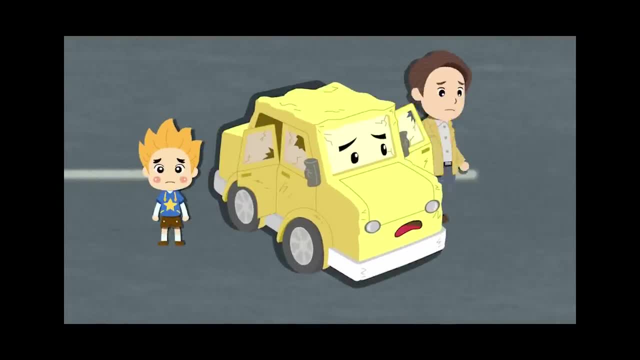 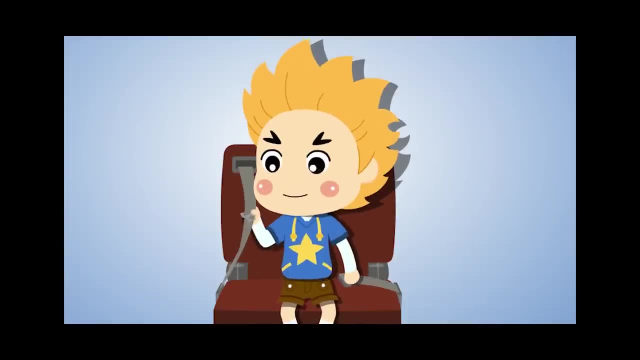 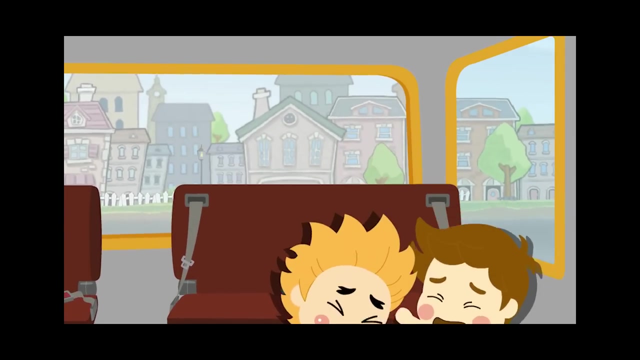 car ever rolls. you're more likely to be safer if you remember to strap in when you wear your seat belt. check to see that it's straight and not twisted across your chest and make sure you hear that click sound when you buckle up. fasten your seat belt as soon as you get in the car so you don't forget and get. 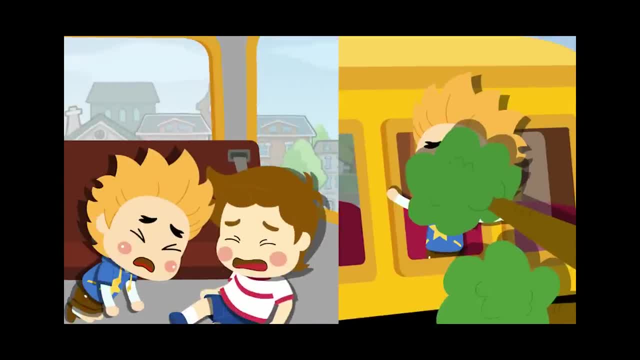 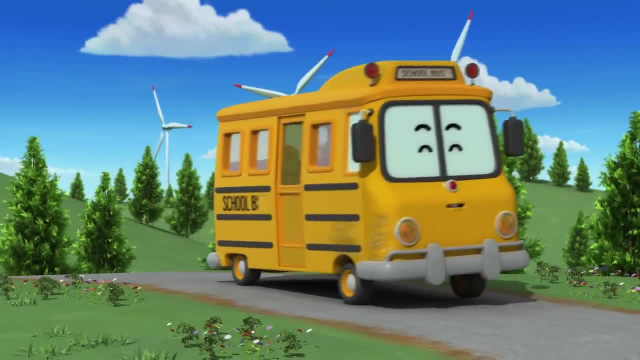 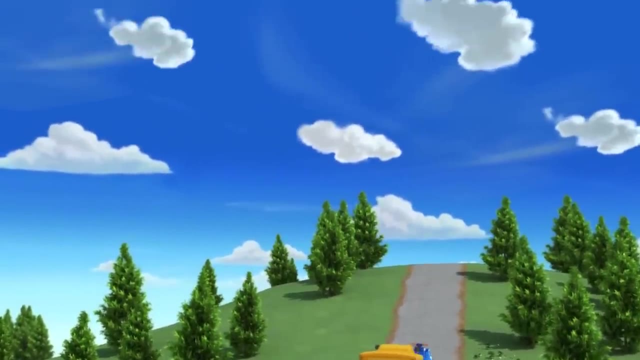 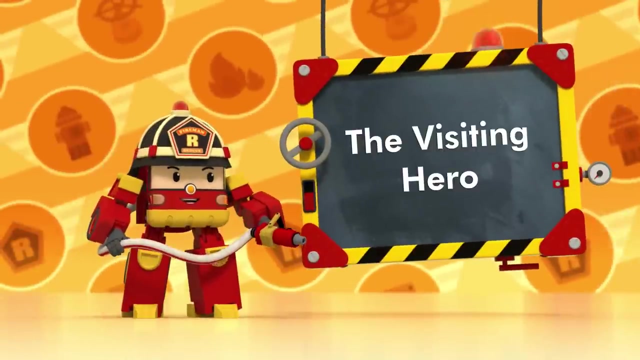 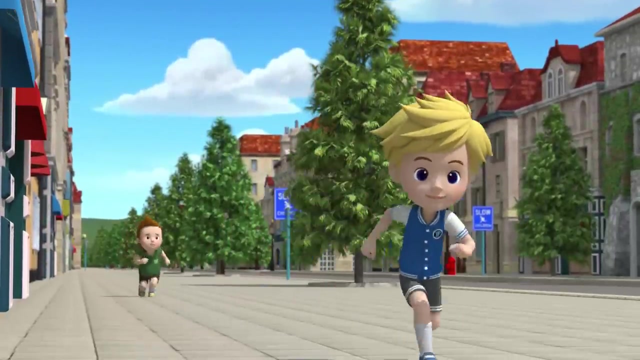 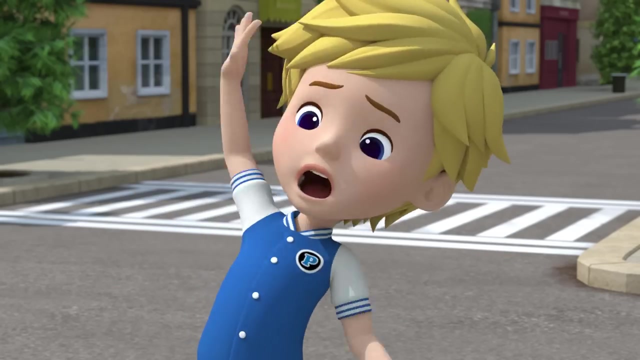 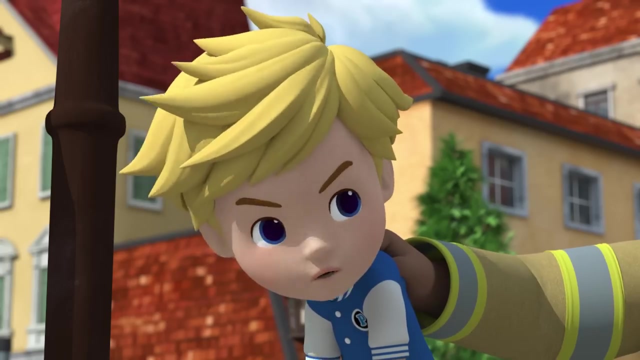 hurt and keep your head and hands inside the car at all times. don't know if you are here with me, though i will be okay, the visiting hero can't catch me. peter, wait up. hey, slowpoke, peter watch it. that wasn't very smart, huh? he didn't mean to, so who are you anyway? 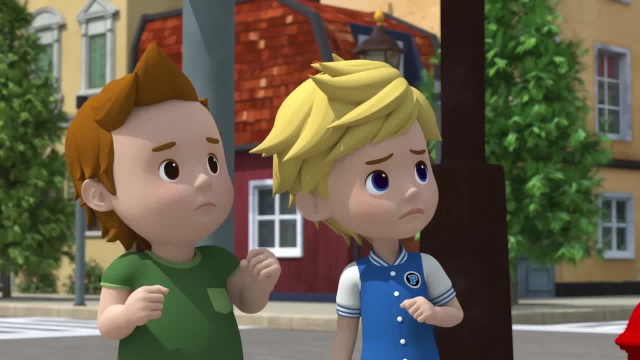 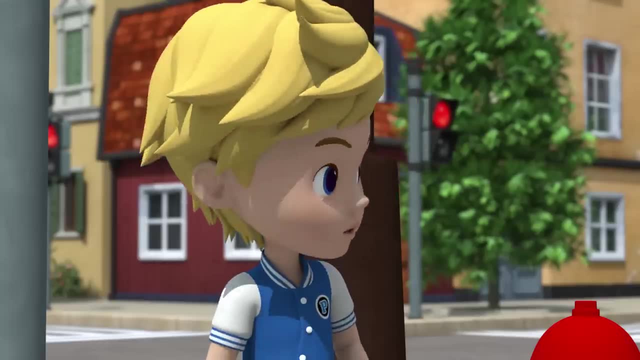 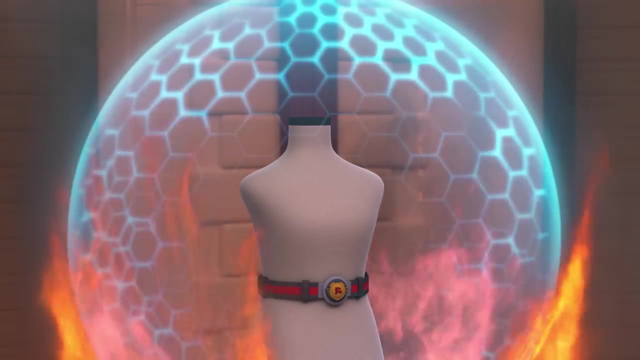 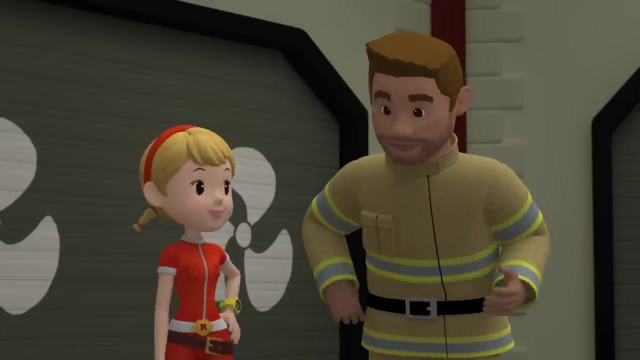 i'm a firefighter who also looks out for children who act up. firefighter, yes, and if you pull that stun again, you'll definitely be punished. fine, huh, and there you have it. it'll protect you in the hottest temperatures. you did an amazing job. we're back. hey everyone, this is tommy, the visiting fireman i told you about. 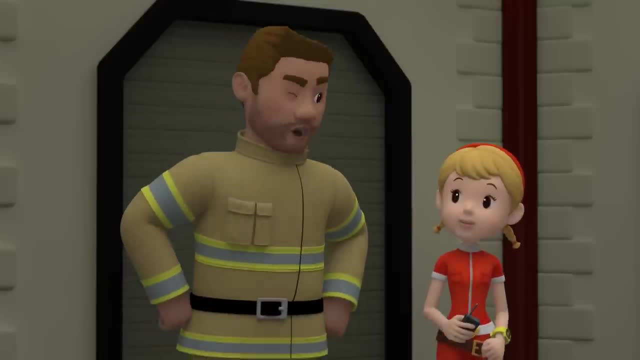 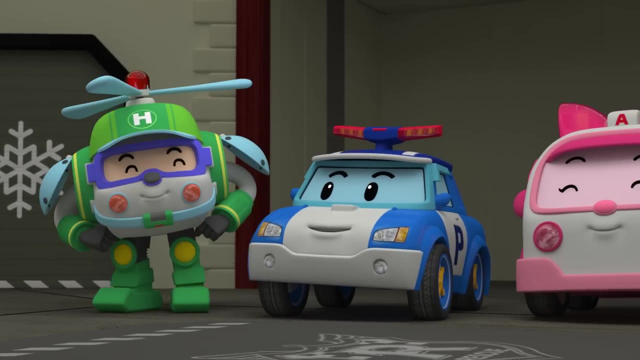 hi tommy, hey there everyone. i've been getting to know brooms town's gifted inventor here and she's awesome a gifted inventor. her stuff's pretty sweet. let me know if you ever need help with a rescue. thank you, i'll do that. oh, i've got all sorts of 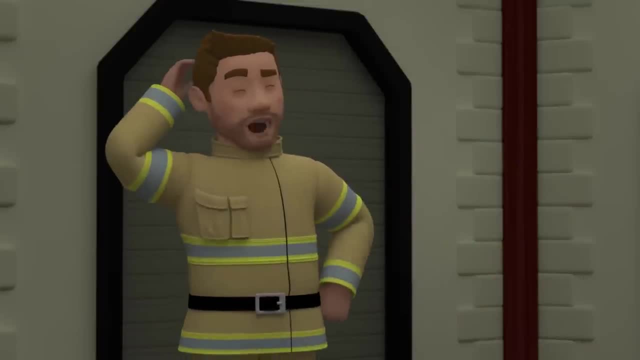 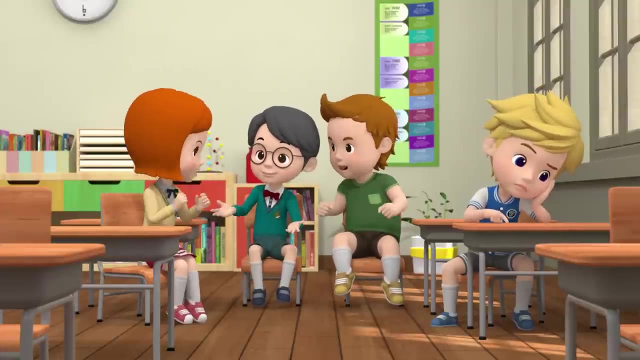 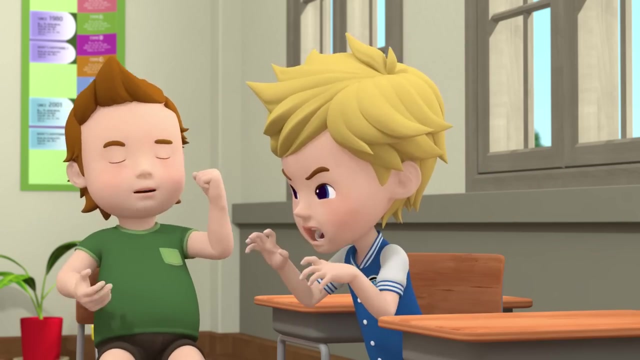 other stuff in storage. wait right here and i'll go get it. this is gonna take longer than i thought it would. hahaha. mr builder would have been a goner without him. he's like a firefighter superhero, huh. what are you talking about? that loser who went all crazy on us for no reason at all? 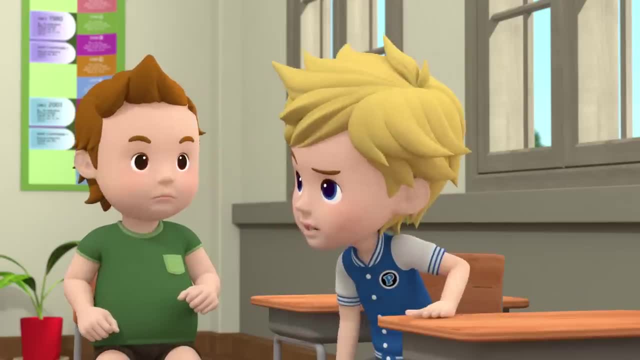 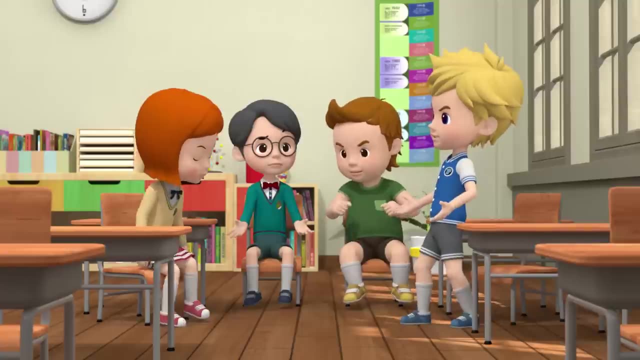 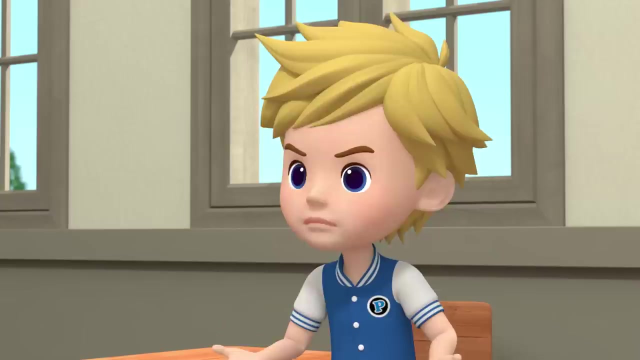 peter, don't talk about tommy like that. oh, i can't believe you're all buying his act. you guys should have been there yesterday. so there, you guys still think he's so great. peter, you shouldn't have been playing like that in the first place. what i'm with tommy, you're always in trouble. it really wasn't. 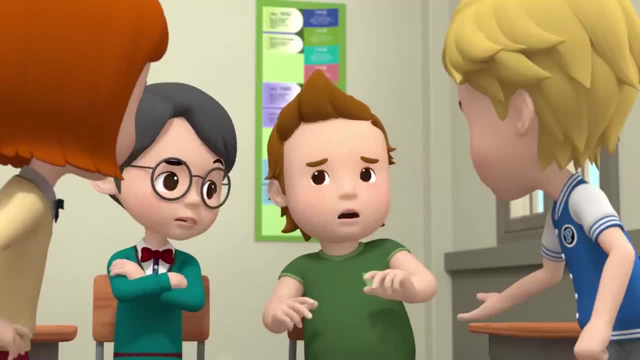 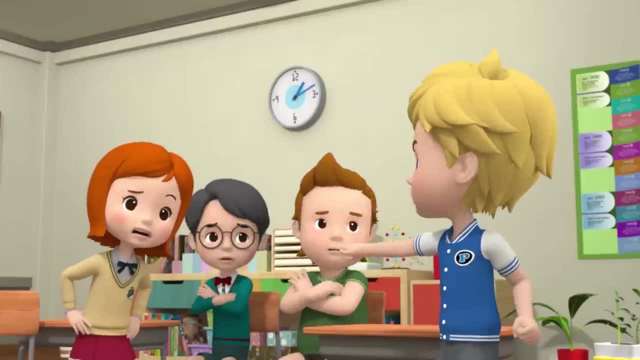 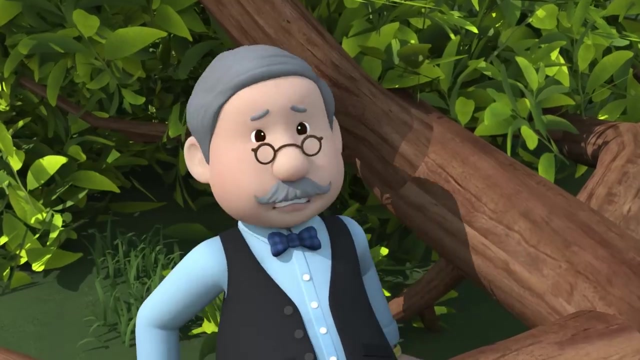 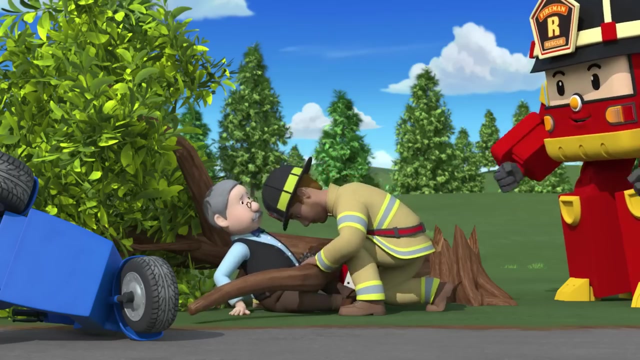 like that, johnny, please back me up. well, you shouldn't act like that, peter. oh, come on, johnny, come with me. i'm gonna show you that mr perfect isn't as great as you think. see that, there you're free. you saved the day, my friend. look at him. 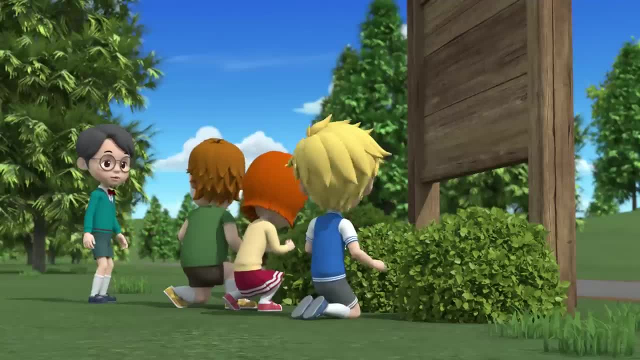 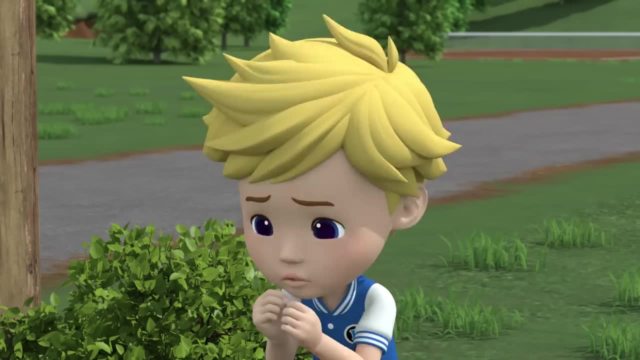 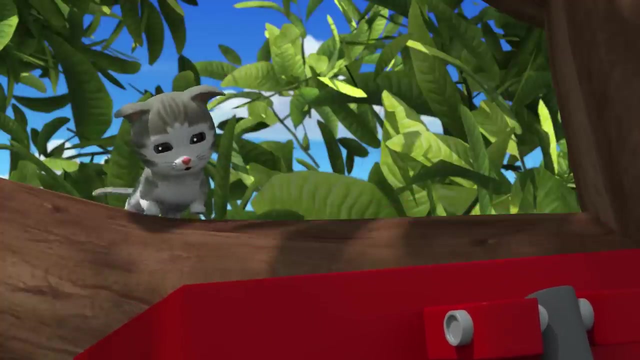 he's just so awesome. seriously, peter, i have to go home and do my work, me too. no wait, you can't go home yet. give me another chance to prove it. come on, look at that. can you believe how bad he's tormenting mary's poor little kitten? 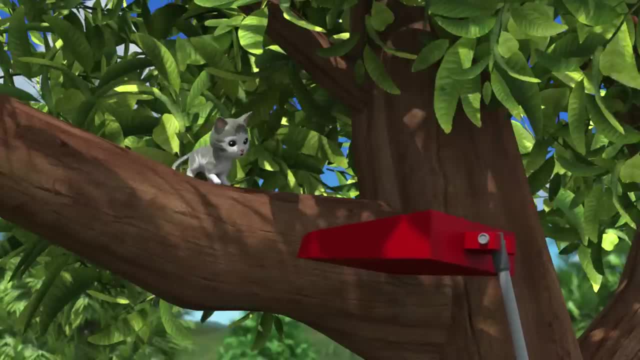 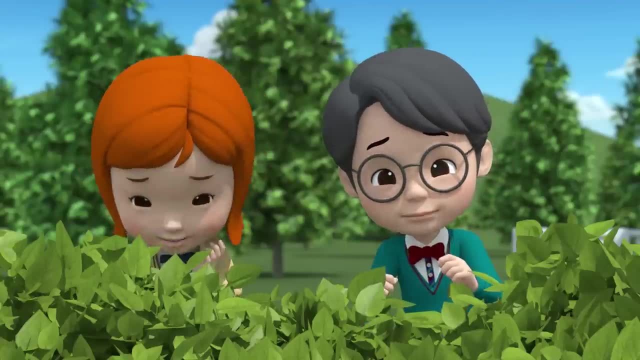 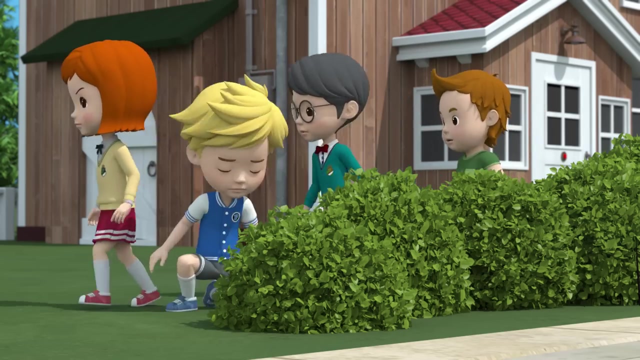 oh no, it's okay, you can do it. ah, good kid, how come he did it, isn't he compassionate? what? no, don't believe him, peter. you have to stop. i've had it. see you later. wait, don't go yet, jim. what's up? there's a fire at the warehouse and 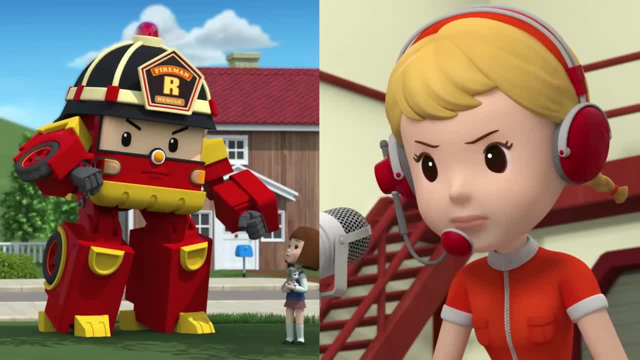 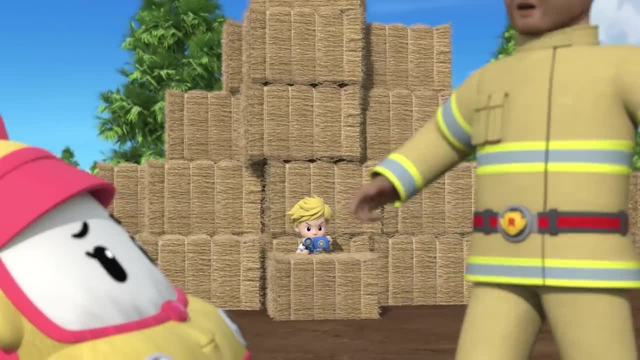 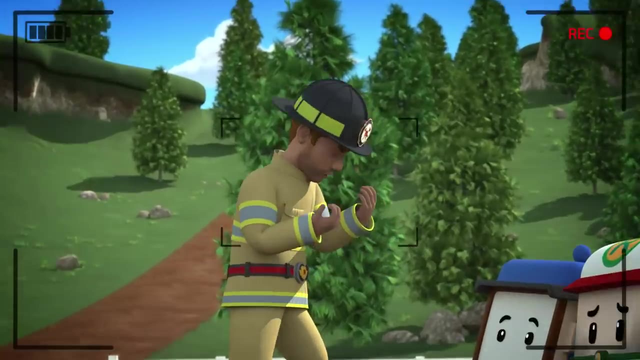 there's somebody trapped inside. you have to go now on my way. you kids could have been hurt. you should have known not to go play in there. awesome, now everyone can see what he's really like. listen up, you three. all that hay is very flammable. one spark and that's all.